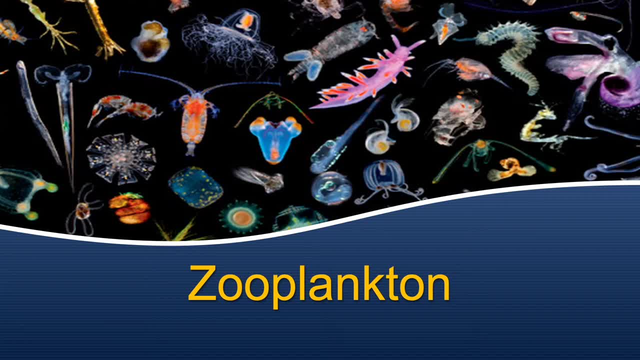 So, naturally, today's lecture is going to be focusing on these awesome marine organisms. This lecture will be a brief introduction into zooplankton and the many ways that people have been studying these tiny little organisms. I'll be going through habitat, diet, size, classification, basic taxonomy. 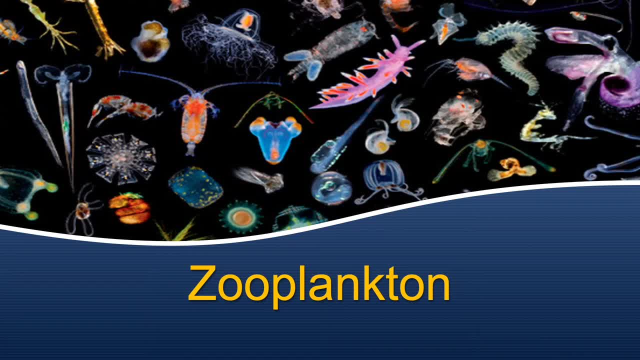 and migration patterns to help give everyone a better picture of why zooplankton are an important part of the marine food web. and to round out our lecture today, i actually also want to spotlight some of the cool research that has been done to help everyone better understand zooplankton. 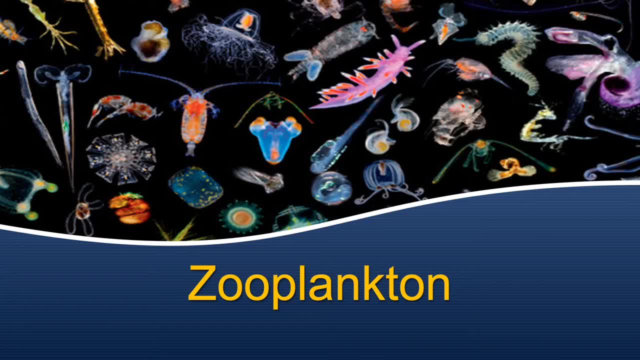 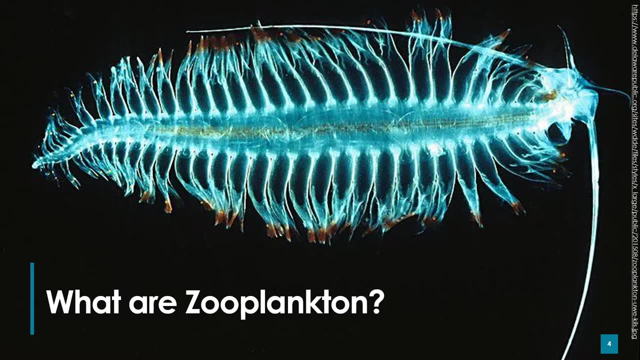 and their role within the oceans. all right, so by this point i think i have said zooplankton enough times, right, so i'm going to say it a couple more, unfortunately, so bear with me. um, today we're going to focus specifically on marine zooplankton. there are freshwater zooplankton and there are. 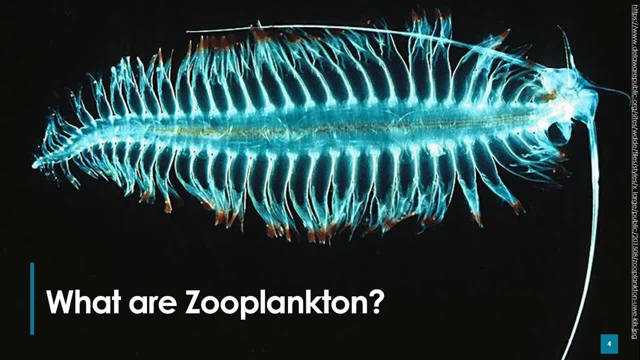 very lots of similarities between the two, but for today we're going to just focus on the marine guys. and so zooplankton are planktonic animals that can live at all depths of the ocean. the word zooplankton actually is derived from the greek. 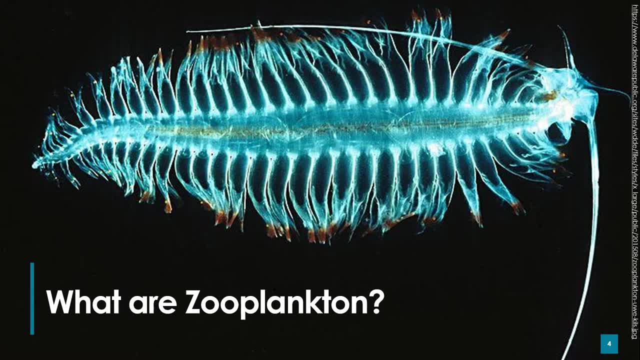 word zune, meaning animal, and planktos, meaning to wander or drift. so when you combine the two, what you get are wandering or drifting animals, which pretty much sums up zooplankton. this is one of those random tidbits that you might want to remember, because you never know when it might. 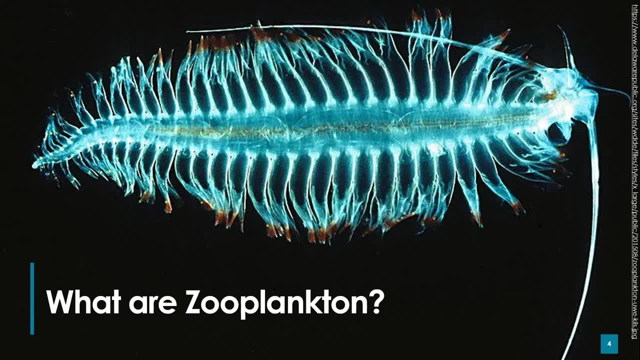 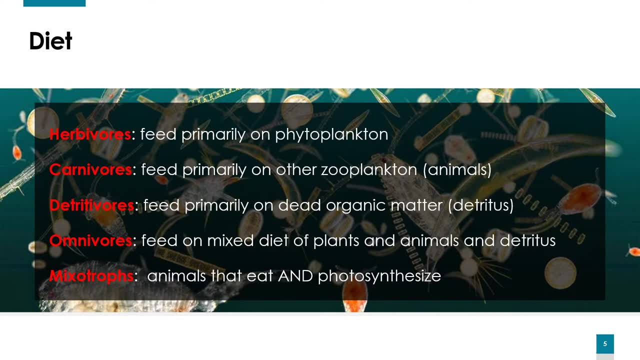 be handy for one of your zoom trivia nights. many might assume that zooplankton might consist of a other types of zooplankton, and while this is definitely one way to gather nutrients, zooplankton have evolved many different strategies in order to eat and to survive, and so, and one of those is 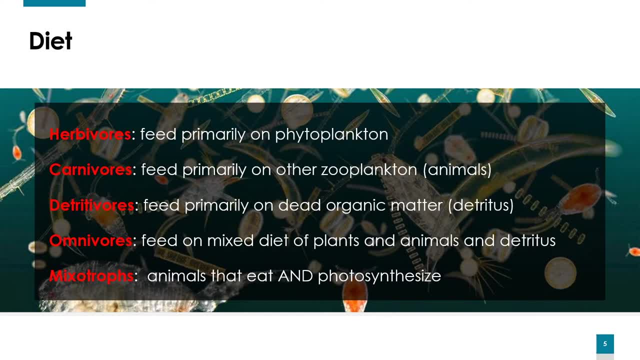 to actually be herbivores or herbiferous and feed primarily- excuse me, on phytoplankton, another one, what you're familiar with is carnivores- or to be carnivorous- carnivorous zooplankton, feed on other types of zooplankton, so other animals. 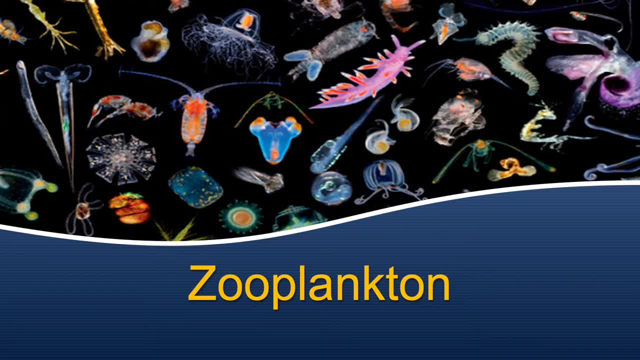 I'll be going through habitat diet, size, classification, basic taxonomy and migration patterns to help give everyone a better picture of why zooplankton are an important part of the marine food web. And to round out our lecture today, I actually also want to spotlight some of the cool research that has been done to help everyone better understand zooplankton and their role within the oceans. 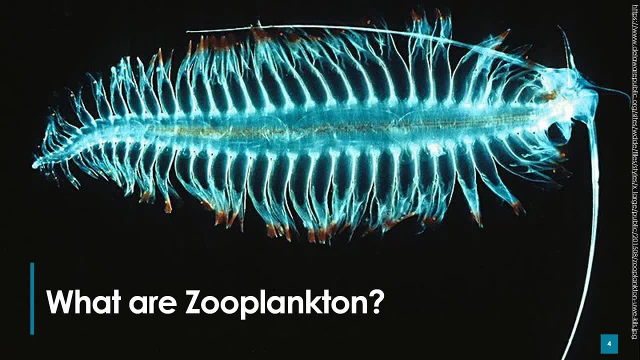 All right. so by this point I think I have said zooplankton enough times, So I'm going to say it a couple more, unfortunately, so bear with me. Today we're going to focus specifically on marine zooplankton. 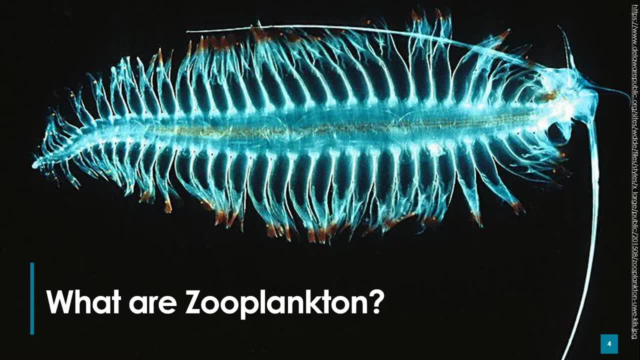 There are freshwater zooplankton, and there are lots of similarities between the two, But for today we're going to just focus on the marine guys. And so zooplankton are planktonic animals that can live at all depths of the ocean. 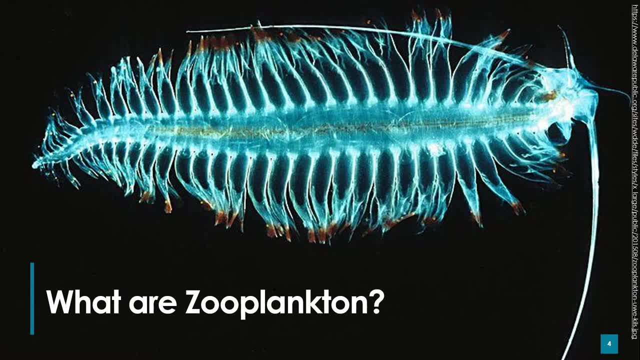 The word zooplankton actually is derived from the Greek word zooplankton, Zoon, meaning animal, and planktos, meaning to wander or drift. So when you combine the two, what you get are wandering or drifting animals, which pretty much sums up zooplankton. 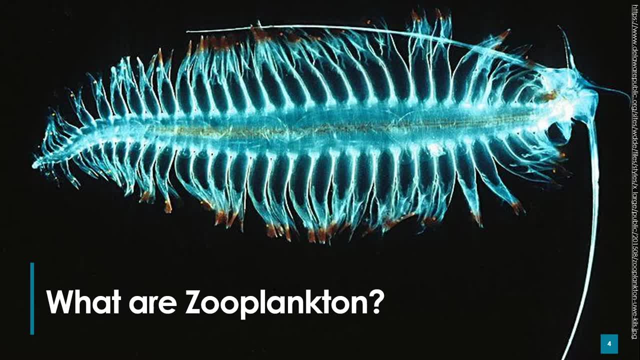 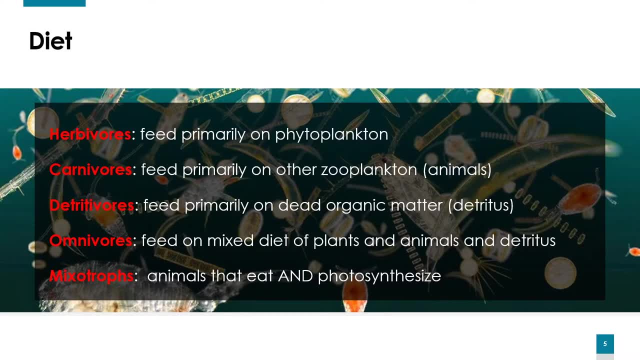 This is one of those random tidbits that you might want to remember, because you never know when it might be handy for one of your Zoom trivia nights. Many might assume that zooplankton might consist of a diet of just eating other zooplankton. 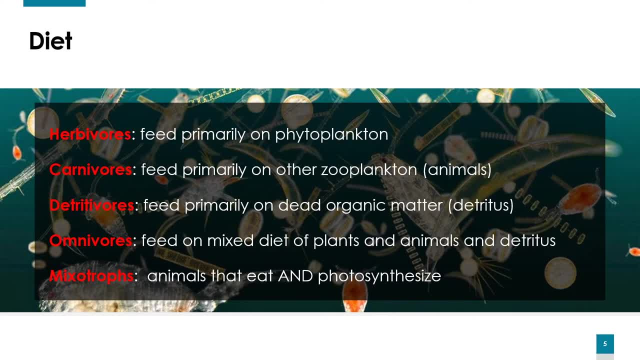 Others are types of zooplankton, And while this is definitely one way to gather nutrients, zooplankton have evolved many different strategies in order to eat and to survive, And so one of those is to actually be herbivores or herbiferous, and feed primarily- excuse me, on phytoplankton. 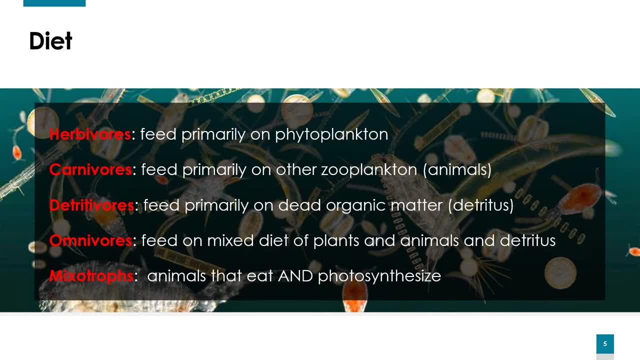 Another one which you're familiar with is carnivores, or, to be carnivorous, Carnivorous zooplankton feed on other types of zooplankton, so other animals, And then we have zooplankton that are detritivores, or they eat primarily detritus, which is the dead organic matter. 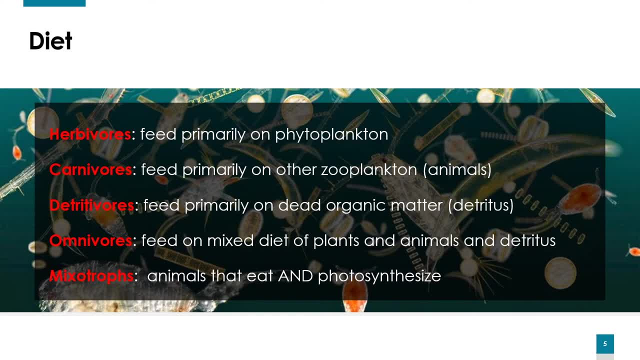 and then we have zooplankton that are dratidivores, or they eat primarily detritus, which is the dead organic matter um that we can. it usually will fall throughout the water column. and then we have zooplankton that will also be omnivorous, and so they feed on a mixed diet of 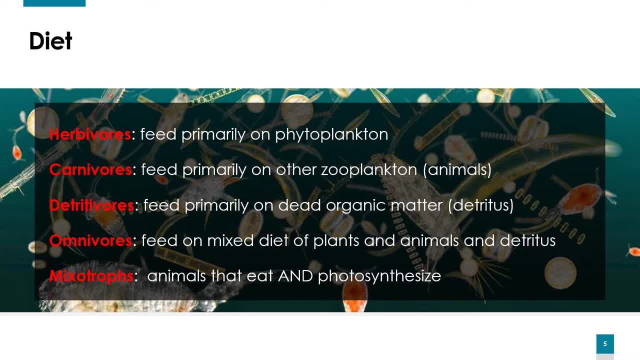 and animals and detritus, so probably one of the least picky eaters out there. so kudos to them, i suppose. and then, lastly, we have our mixotrophs, and so these are very interesting um organisms that they can eat, other zooplankton and also photosynthesize. 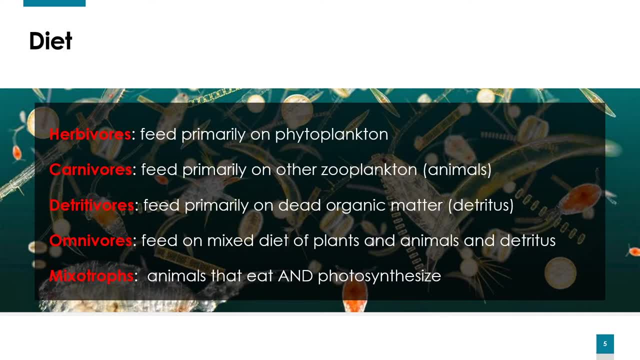 and so examples of mixotrophs might include ciliates or riseria and their mixotrophic um, owing to their ability to retain functional algal organelles or maintenance of their alcohol endo symbionts. and so, um there's just when you think about how zooplankton are able to. 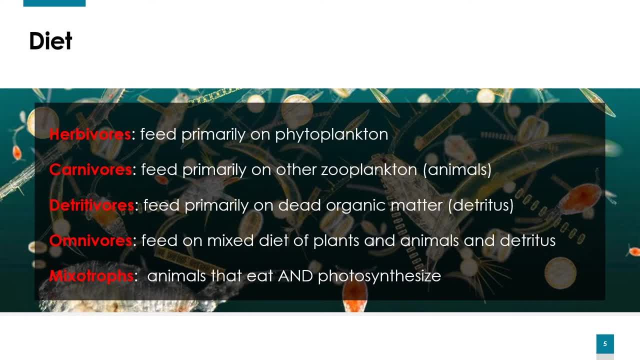 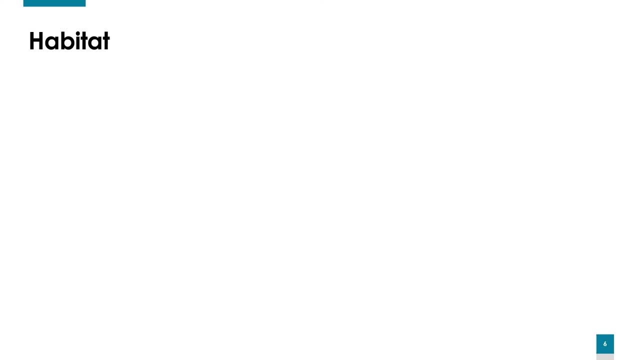 eat and survive. there's just a lot of different ways that they are able to do that. all right. so all of zooplankton can fall into one of two categories: either they are hollow plankton or they are marrow plankton, and so hollow plankton go on here. there we go. hollow plankton are types. 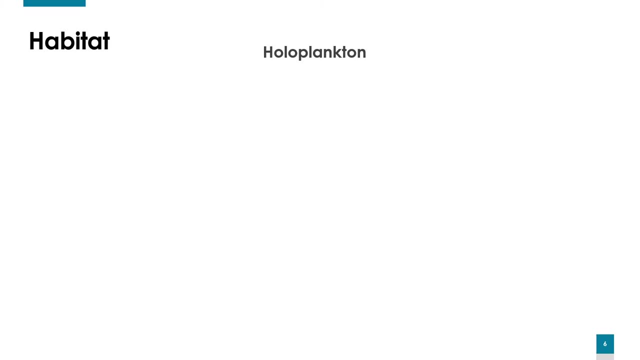 of plankton that will stay in the planktonic state their whole lives and they will drift and drift and drift throughout the epi mesopelagic pelagic zones- and i will expand a little bit more on that later. and so hollow plankton. as you can see here in this image, there's many different types. there's. 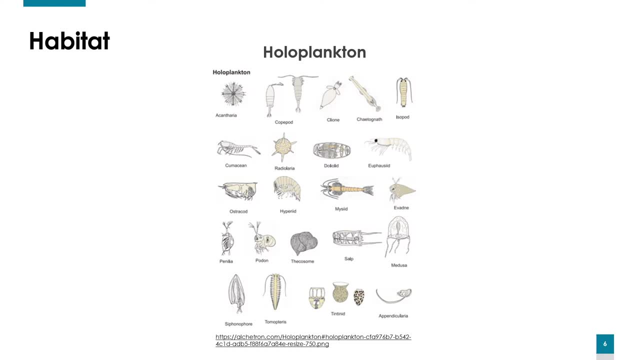 many different types of microplankton and they can range in size from a few micrometers to very, very large. uh, we're talking maybe, uh, cnidarians like jellies or siphonophores, and so hollow plankton, are very important because they serve as a vital food source. 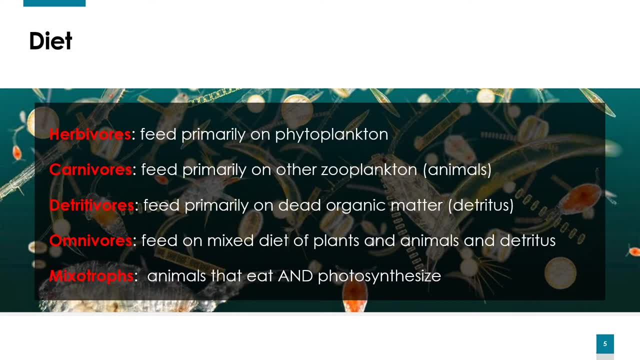 that usually will fall throughout the water column. And then we have zooplankton that will also be omnivorous, And so they feed on a mixed diet of plants And animals and detritus, So probably one of the least picky eaters out there. 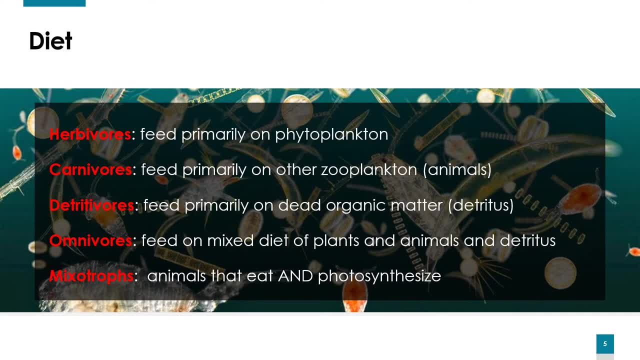 So kudos to them, I suppose. And then, lastly, we have our myxotrophs, And so these are very interesting organisms in that they can eat other zooplankton and also photosynthesize, And so examples of myxotrophs might include ciliates or rhizaria. 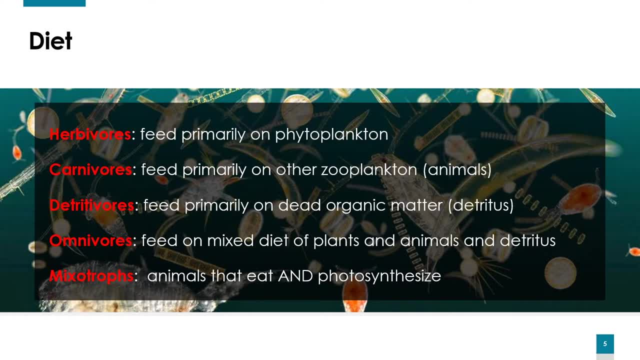 And they're myxotrophic Owing to their ability to retain functional algal organelles or maintenance of their algal endosymbionts. And so there's just when you think about how zooplankton are able to eat and survive. 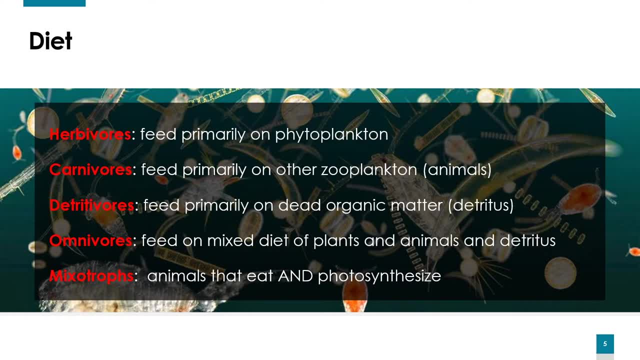 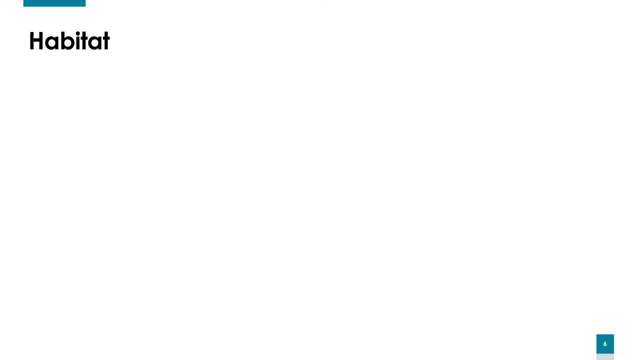 there's just a lot of different ways that they are able to do that. All right, so all of zooplankton can fall into one of two categories: Either they are hollow plankton or they are meroplankton, And so hollow plankton. let me go on here. There we go. Hollow plankton are types of plankton that will stay in the planktonic state their whole lives and they will drift and drift and drift throughout the epi- and mesopelagic zones, And I will expand a little bit more on that later. 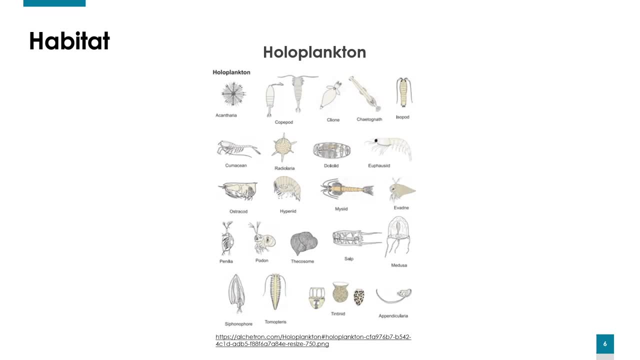 And so hollow plankton, as you can see here in this image, there's many different types. There's lots of different types of hollow plankton, And they can range in size from a few micrometers to very, very large. We're talking, maybe, cnidarians like jellies or siphonophores. 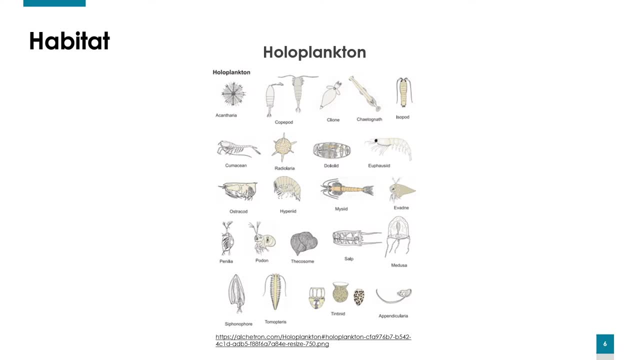 And so hollow plankton are very important because they serve as a vital food source for large organisms like fish or baleen whales. When you think of whales, you might think of like a humpback whale or something And an example. I want to show you some- 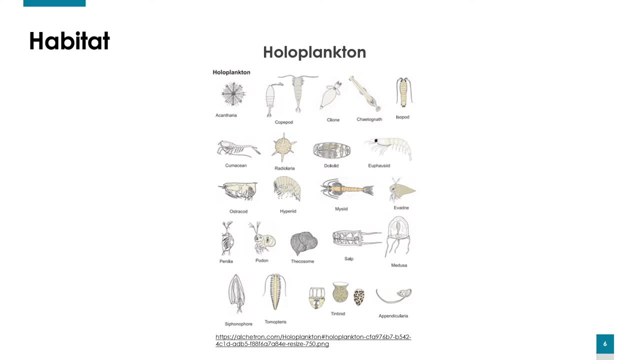 I just want to highlight some of the different types of plankton that I've seen in the samples that I work with. So it can vary between- let me get my pen- It can vary between copepods or between- I've seen doliolids in our samples, definitely seen euphausids. 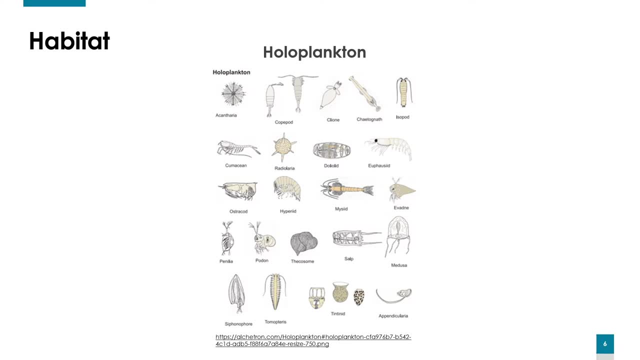 for large organisms like fish or baleen whales. when you think of whales, you might think of like a humpback whale or something, an example. i want to show you some. i just want to highlight some of the different types of plankton that i've seen in the samples that i work with, so it can vary between. let me get my pen. 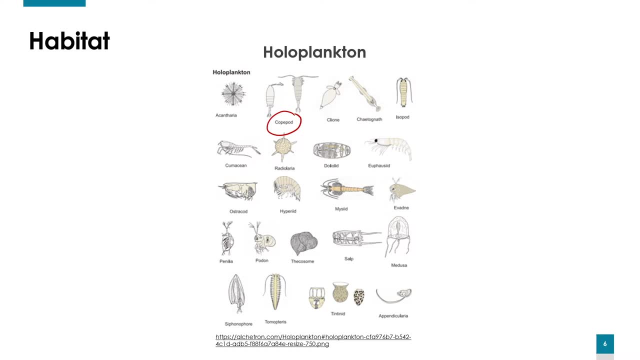 it can vary between copepods or between. i've seen doliolids in our samples, definitely seen euphausids um. i've definitely seen salps. some years we've had lots and lots of salps in our samples um. i've seen siphonophores. pretty often the same goes for appendicularians and again you can see just from. 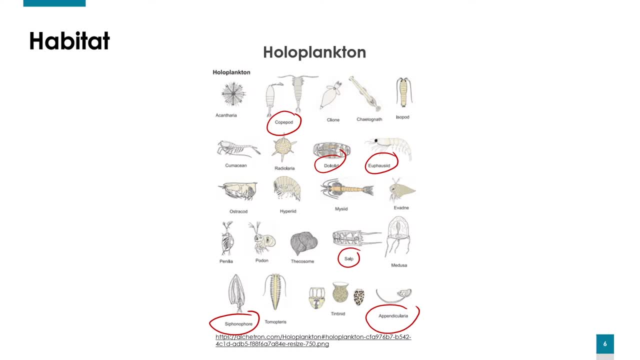 this image that there are many different types of zooplankton that are hollow plankton, and they will stay um very small their whole lives, and so let me go ahead and erase my doodles here. okay, so go ahead and move on to the next one. so the second category that we were talking about are 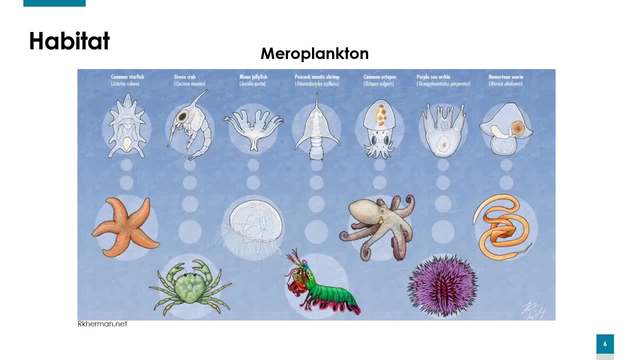 the different types of zooplankton, and so marrow plankton, are types of plankton that um will only stay plankton, and for a part of their lives, and so typically that would mean the early stages of development for these different organisms, and so they start off in the planktonic state. 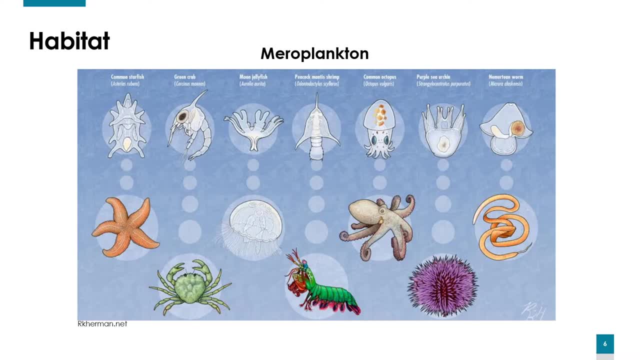 as monopoly i. but then, as they mature and become larger, they will settle in different parts of the ocean. probably have seen before whether it's at the beach or whether it was at an aquarium. all of these organisms you see here, they, they all had to start off. 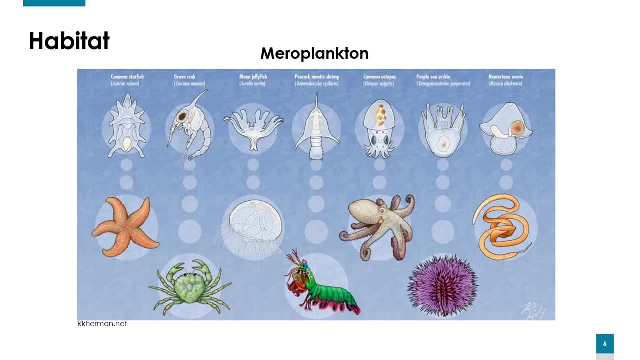 pretty small, and so a common example we might see pen would be the common sea star, although right here it says starfish. that's not what we're supposed to say. another one we might see a lot at the beach would be crabs. here we have the green crab. if you have been to an aquarium recently, you may have had the. 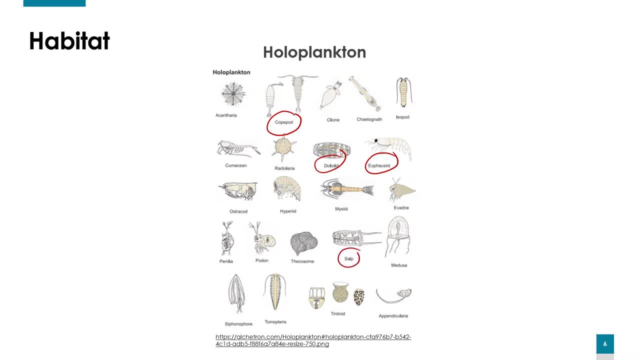 I've definitely seen salps. Some years we've had lots and lots of salps in our samples. I've seen siphonophores. pretty often The same goes for appendicularians, And again you can see just from this image that there are many different types of zooplankton that are hollow plankton. 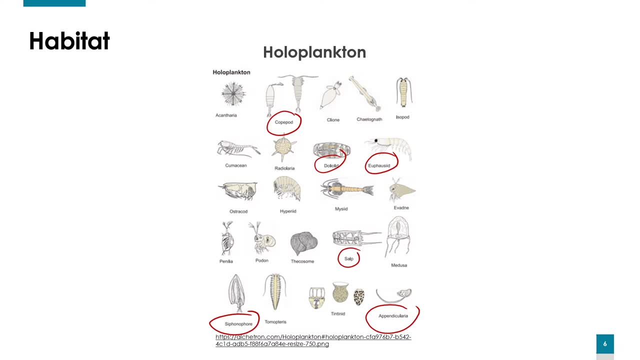 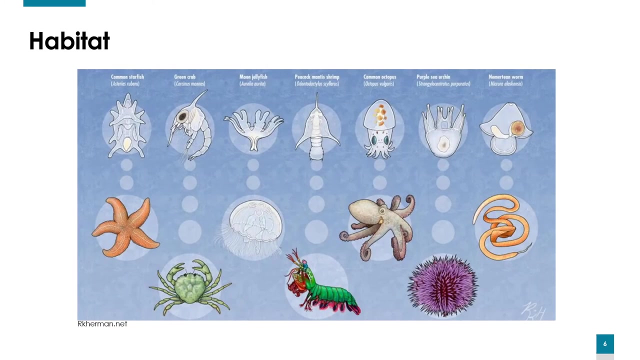 And they will stay very small their whole lives, And so let me go ahead and erase my doodles here, Okay, so go ahead and move on to the next one, And so the second category that we were talking about are marrow plankton. 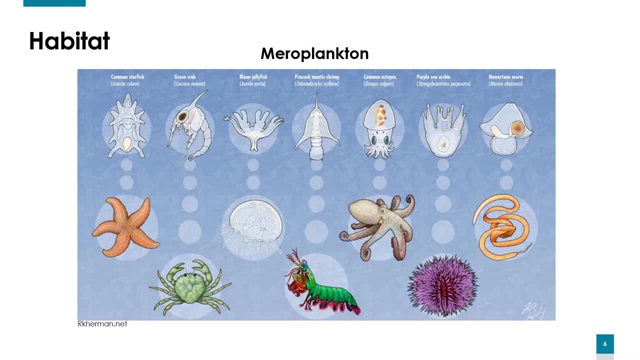 And so marrow plankton are types of plankton that will only stay plankton for a part of their lives, And so typically that would mean the early stages of development for these different organisms. And so they start off in the planktonic state as noplii, but then as they mature and become larger. 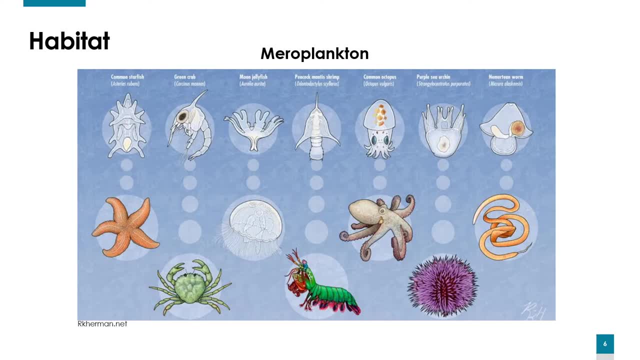 they will settle in different parts of the ocean And a lot of these you probably have seen before, whether it's at the beach or whether it was at an aquarium, All of these organisms you see here. they all had to start off pretty small. 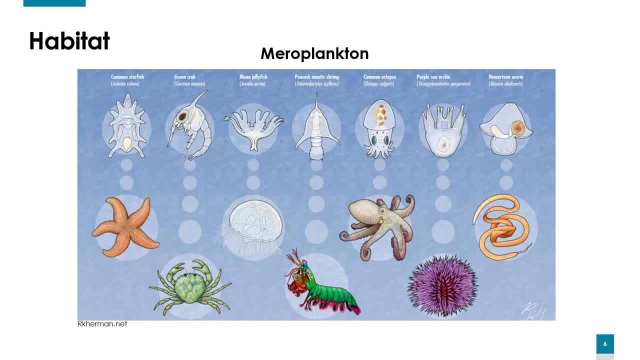 And so a common example we might see: Penn would be the common sea star, although right here it says starfish. That's not what we're supposed to say. Another one we might see a lot at the beach would be crabs. 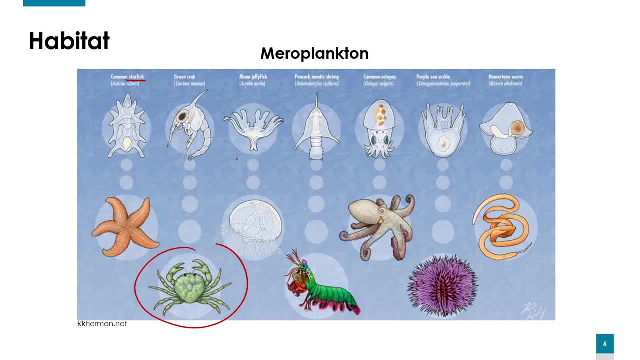 Here we have the green crab. If you have been to an aquarium recently, you may have had the chance to see an octopus- And so all of these organisms had to start off as noplii in the planktonic state, and then, over time, they grew and matured into the organisms you see below. 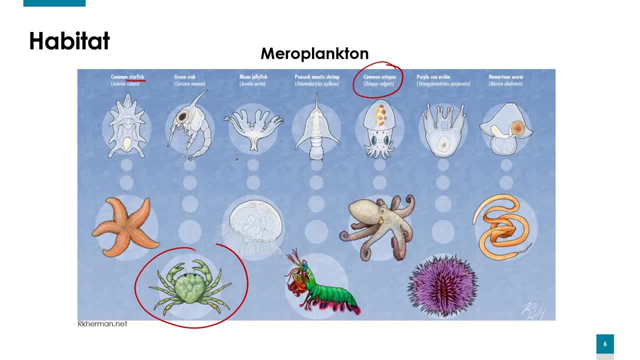 And so these different categories: hollow plankton and marrow plankton. it helps us to be able to better understand the size, different size classifications for the different types of zooplankton and why some stay in the planktonic state and why others mature and grow and become larger. 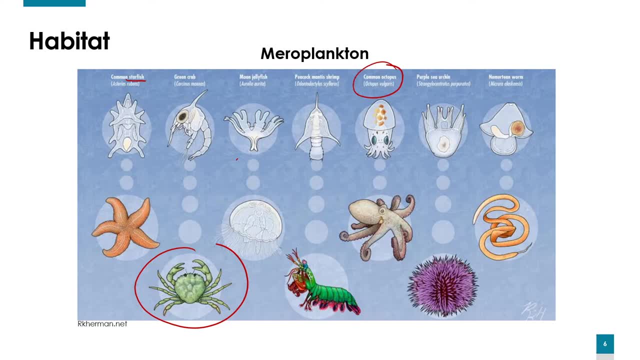 chance to see an octopus, and so all of these organisms had to start off as noplii in the planktonic state and then over time they grew and matured into the organisms you see below, and so these different categories- hollow plankton and marrow plankton- and it helps us to be able to better understand the size. 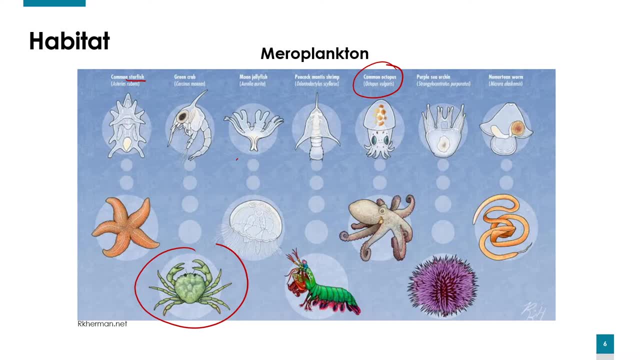 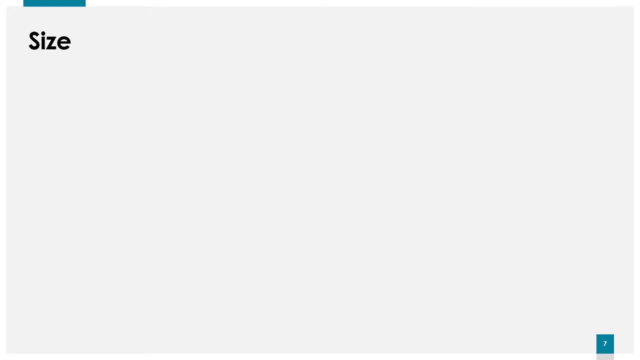 different size classifications for each of these organisms, and so this is a good example for the different types of zooplankton and why some stay in the planktonic state and why others mature and grow and become larger. all right, so zooplankton can also be categorized based by size, and so what we 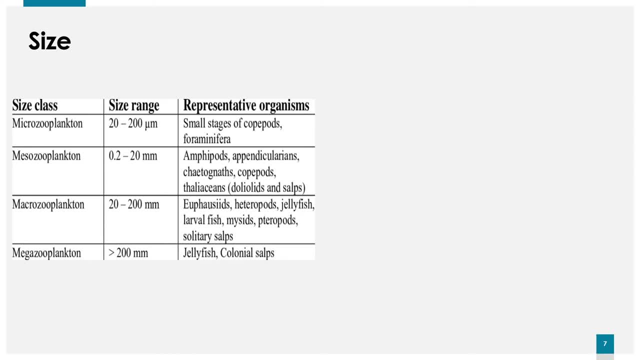 have at this table are four different size classes. before we jump into this table, I want to also talk about a smaller and even smaller size class, and with the larger size class we have an��가plankton, and they're unicellular animals that feed on phytoplankton and are then eaten by other. 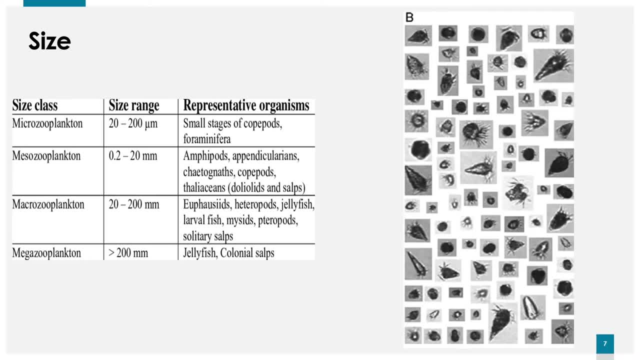 types of zooplankton and their size range can vary from 2 to 20 micrometers, and we see an example of that here and with these images, in order to be taken, they probably had to use a microscope, because my nano zooplankton are so small. 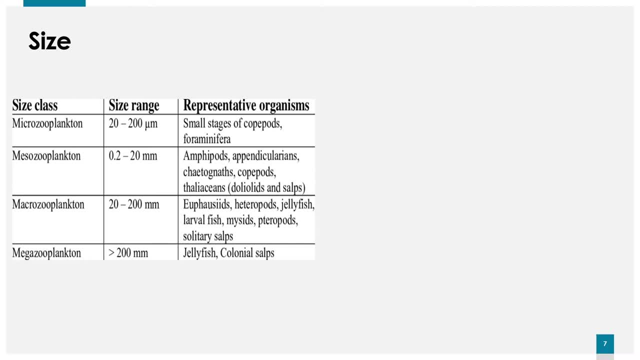 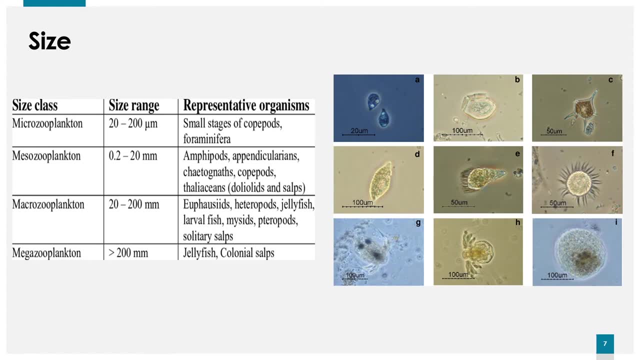 and so now jumping back to the table, we start with microzooplankton and their size range is, for virtual zooplankton, from 20 to 200 micrometers, and different types of organisms that can be represented here would be different stages of copepod, and if we take a look, 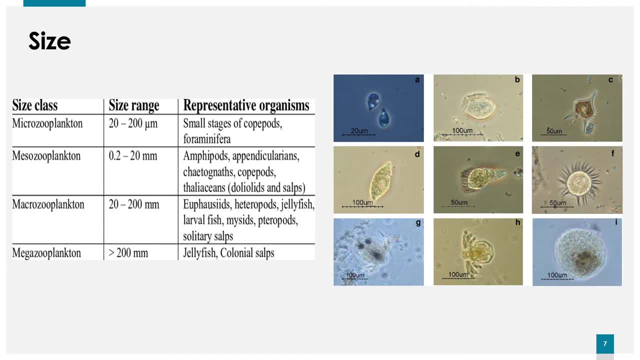 at the bottom of this picture, the bottom row G and H are good examples of two different types of copepod in the anoplyi stage. and then, if we take a look at I here in the bottom right corner, this looks like some type of bivalve. 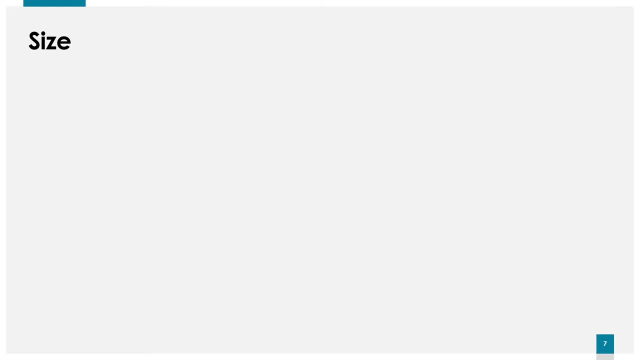 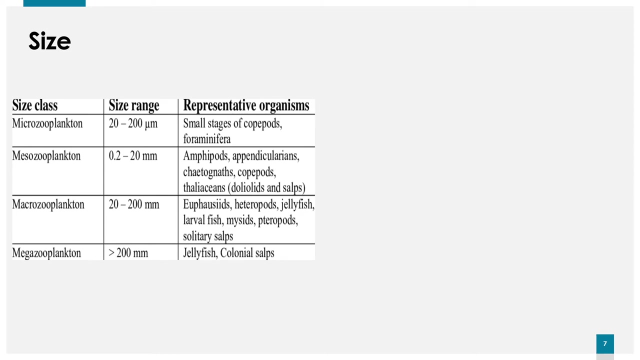 All right, so zooplankton can also be categorized based by size, And so what we have at this table are four different size classes. Before we jump into this table, I want to also talk about a smaller and even smaller size class called nanoplankton. 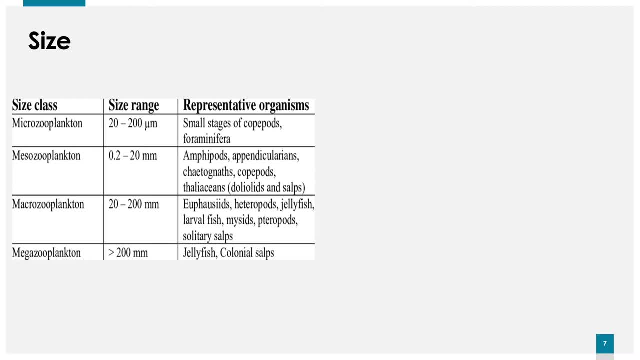 So these are nanoplankton, and they're unicellular animals that feed on phytoplankton and are then eaten by other types of zooplankton, And their size range can vary from 2 to 20 micrometers, And we see an example of that here. 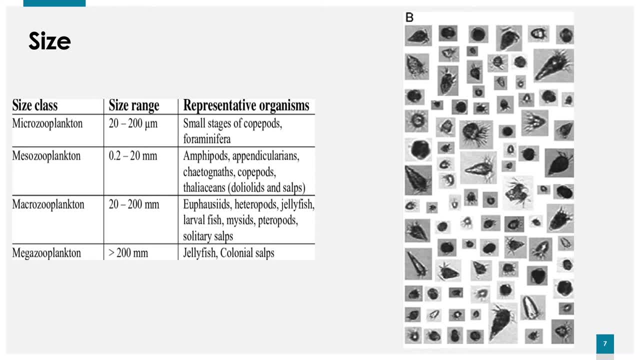 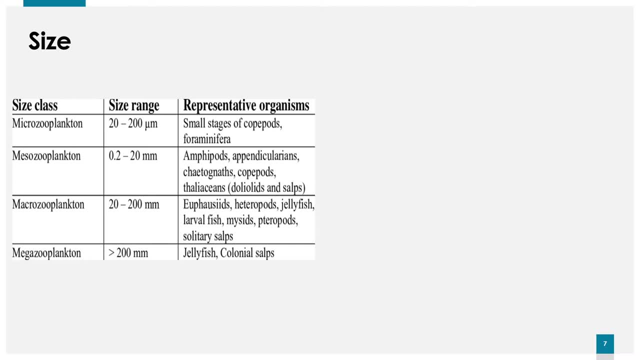 And with these images. in order to be taken, they probably had to use a microscope, because nano zooplankton are so small. And so now, jumping back to the table, we start with micro zooplankton. Their size ranges from 20 to 200 micrometers. 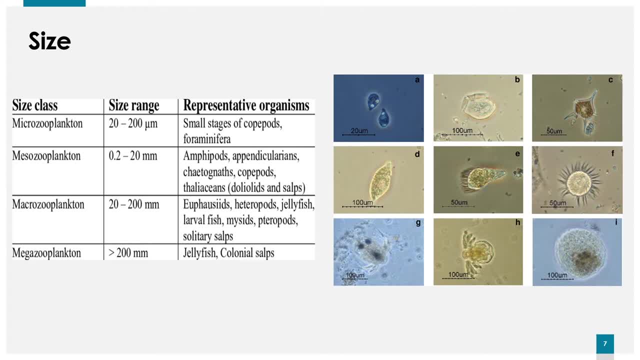 And different types of organisms that can be represented here would be different stages of copepod, And if we take a look at the bottom of this picture, the bottom row G and H are good examples of two different types of copepod in the nopplii stage. 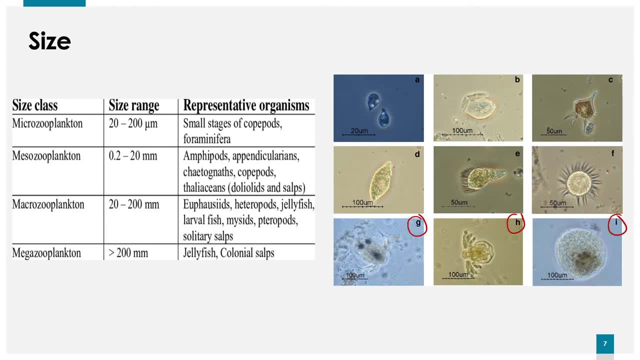 And then if we take a look at I here in the bottom right corner, it's some type of bivalve nopplii in its early stages of development, And so these are pretty good examples to look towards when thinking about the size and what micro zooplankton might look like. 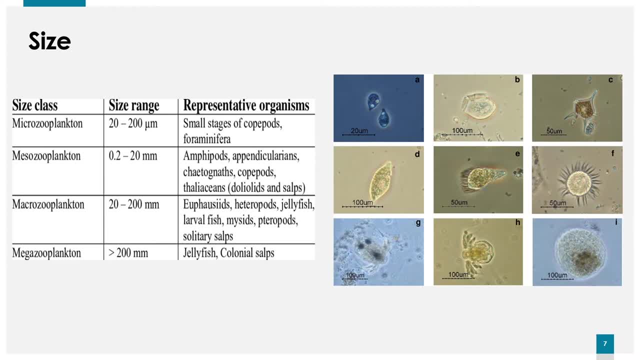 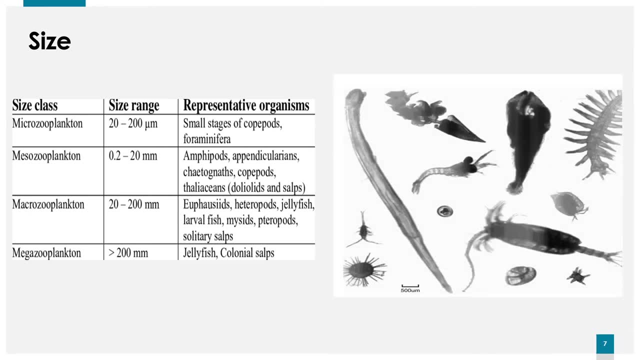 And then let's go ahead and delete our doodles And moving on. Okay so mesozooplankton. they range from 0.2 to 20 millimeters, So we're going up in size a little bit, And different types of organisms within this category could be amphipods. 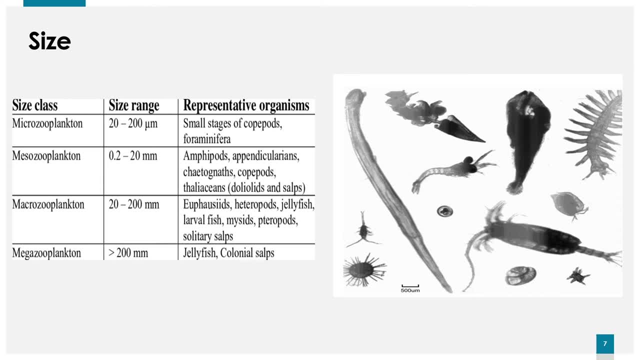 appendicularians, chidignats and copepods, or doliolids and selps, And with organisms in this size class, you can see that the body type can change dramatically, And so again, we have different types of copepod here. 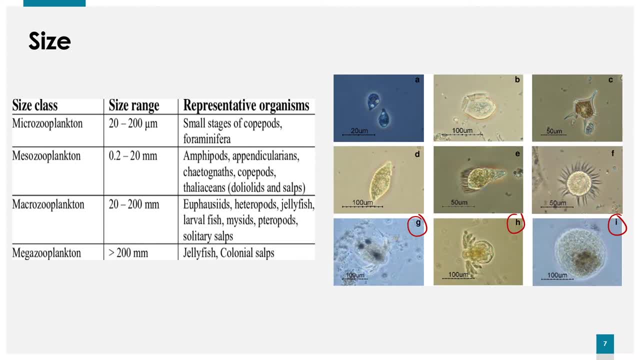 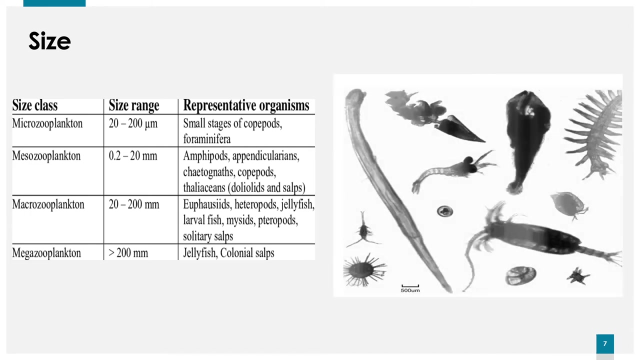 anoplyi in its early stages of development, and so these are pretty good examples to look towards when thinking about the size and what what micro zooplankton might look like. and then let's go ahead and delete our doodles and moving on. okay, so mesozooplankton: they range from 0.2 to 20 millimeters. 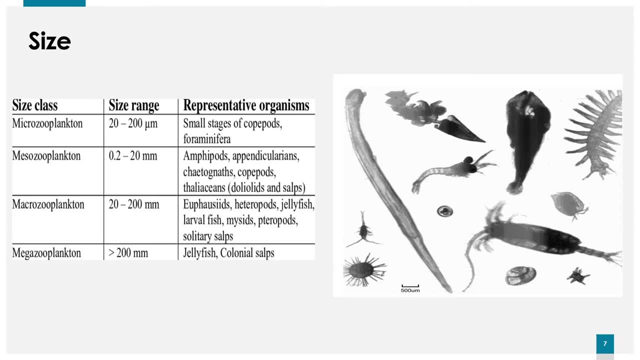 so we're going up in size a little bit and different types of organisms within this category could be amphipods, appendicularians, chidignads and copepods, or doliolids and seps, and with these, with organisms in this size class, you. 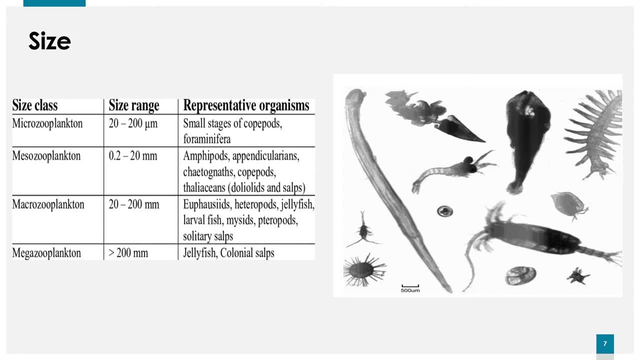 can see that the body type can change dramatically. and so again we have different types of copepod. here we have what looks like some sort of marine worm. We have a ketignath here a euphausid. here so many different shapes, sizes, all included in the mesozooplankton category. 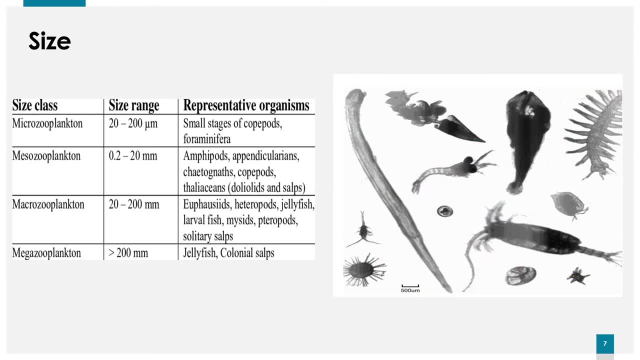 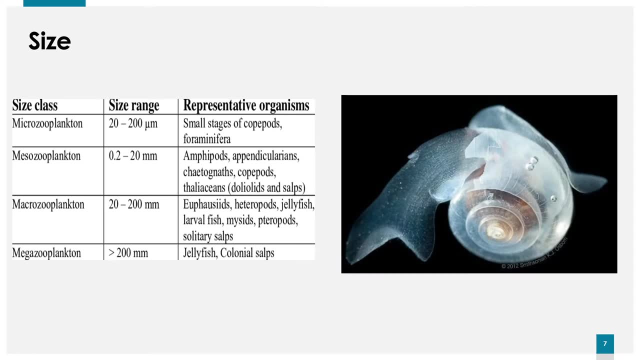 And then go ahead, erase, erase, okay, and moving on. So the next one we have are macrozooplankton and macrozooplankton. their stage or their size can range from 20 to 200 millimeters, so they're getting much bigger. 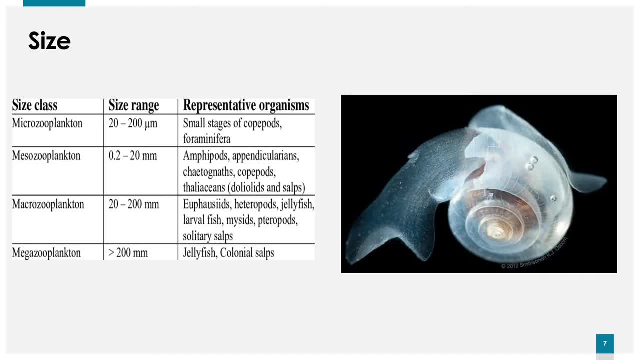 And organisms in this category can include euphausids, heteropods, jellyfish, larval fish, mysids, pteropods and solitary salps, And so what we have an image here on the right is an example of a pteropod called Limacina helicina. 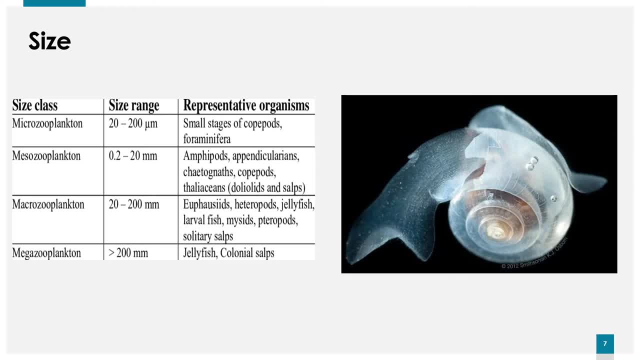 And you can tell here that part of its shell actually has been damaged, And this probably occurred when it was being collected through the net or something, And so, because these shells are very delicate, they're not used to being handled roughly or being tossed around by current. 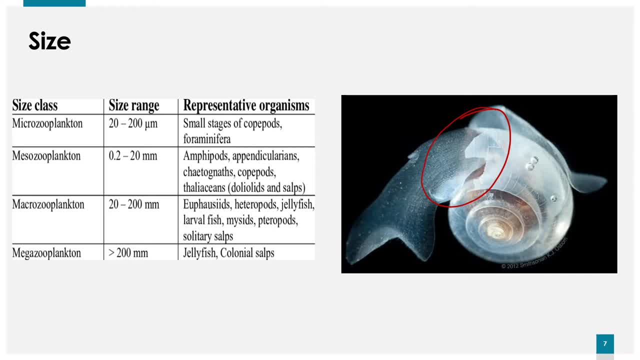 a strong current because they live at a lower depth in the water column. But you can see that the shell is very delicate, So the shell should have extended a little bit further down here. But this is a nice example of what a macrozooplankton might look like. 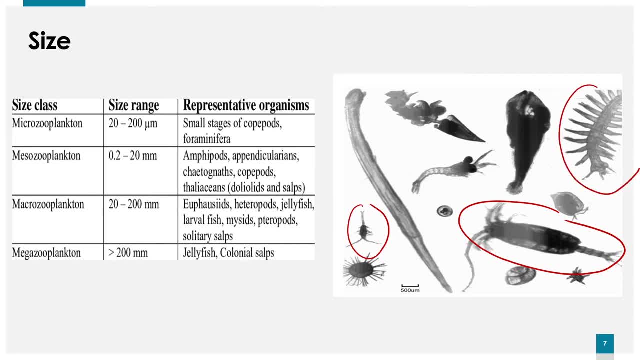 We have what looks like some sort of marine worm. We have a chidignath here, a euphausid here. So many different shapes, sizes, all included in the mesozooplankton category, And then go ahead, erase, erase. 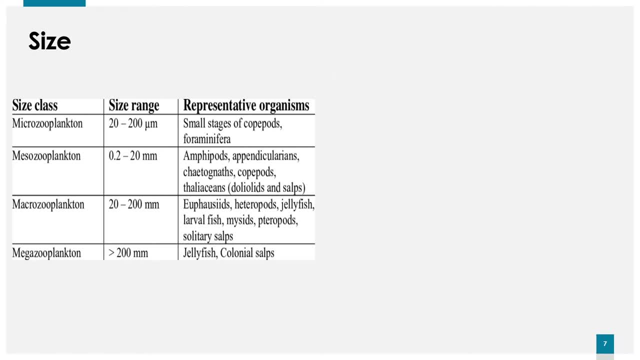 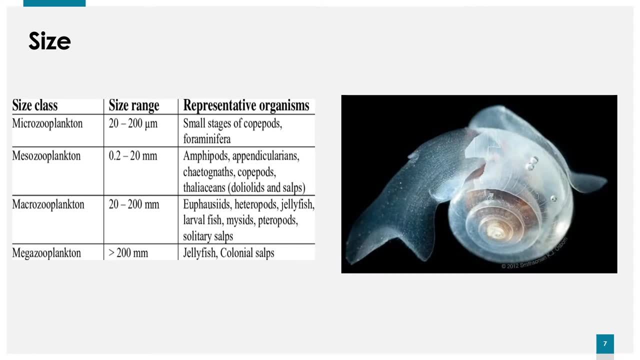 Okay, and moving on. So the next one we have are macro zooplankton And macro zooplankton, their stage or their size can range from 20 to 30 millimeters To 200 millimeters, so they're getting much bigger. 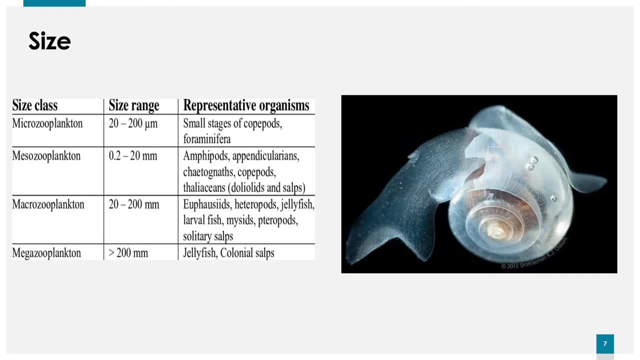 And organisms in this category can include euphausids, heteropods, jellyfish, larval fish, mysids, pteropods and solitary selps, And so what we have an image here on the right is an example of a pteropod called Limacina hellicina. 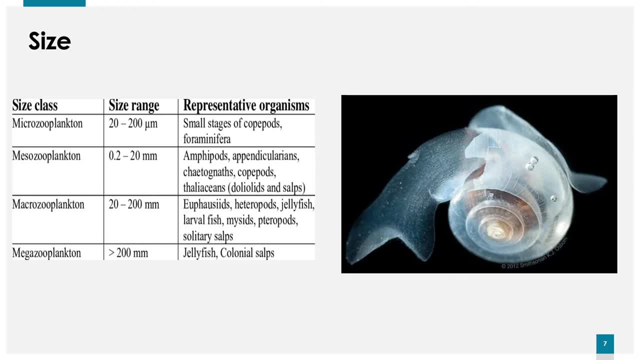 And you can tell here that part of its shell actually has been damaged And this probably occurred when it was being collected through the net or something. And so, because these shells are very delicate, they're not used to being handled roughly or being tossed around by current- a strong current- because they live at a lower depth in the water column. 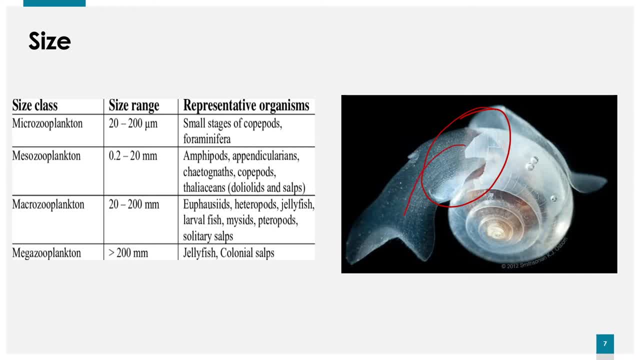 But you can see that the shell should have extended a little bit further down here, But this is a nice example of what a macro zooplankton might look like, And so then, lastly, we'll go to our mega zooplankton. 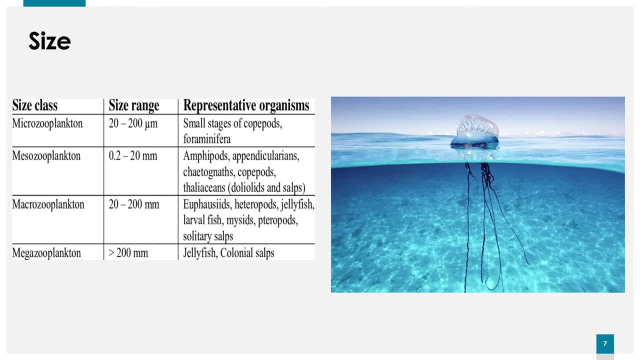 They are pretty much organisms that are greater than 200 millimeters And they can include jellyfish and colonial selps, And in this image here we have a good example, which is called the Portuguese man o' war, which is probably a very popular image, or organisms that we have probably seen in textbooks or on TV, and such. 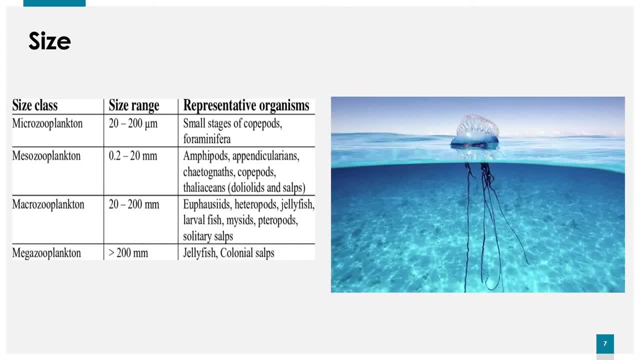 And so then, lastly, we'll go to our megazoplankton. They are pretty much organisms that are greater than 200 millimeters, And they can include jellyfish and colonial salps, And in this image here we have a good example, which is called the Portuguese man o' war. 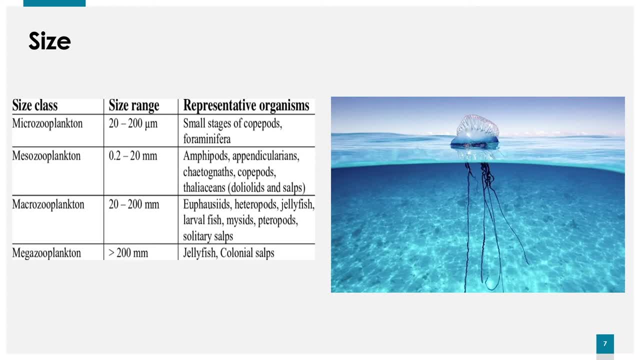 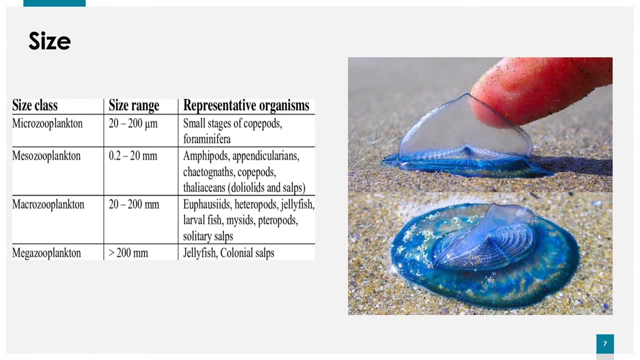 which is probably a very popular image or organisms that we have probably seen in textbooks or on TV and such And then another example that we have are the wind- I'm sorry by the wind- sailor, or Valhalla, Valhalla, And these I have seen wash up ashore in San Diego. 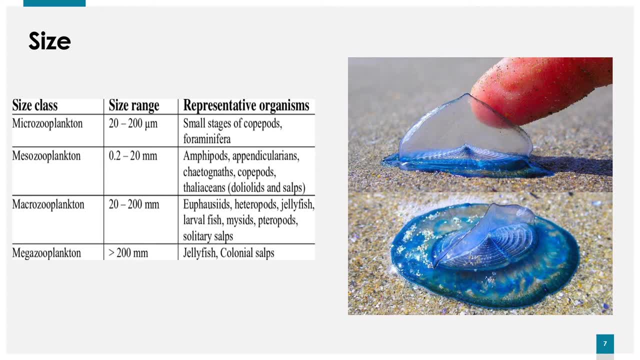 And they've washed up by the tens of thousands And when they dry up they just look like little pieces of blue plastic wrap And they just kind of fly away with the breeze when they dry up And so. but they wash ashore because they use this part of their body like a sail and are propelled along the top of the ocean or the surface ocean from the wind or by the wind. 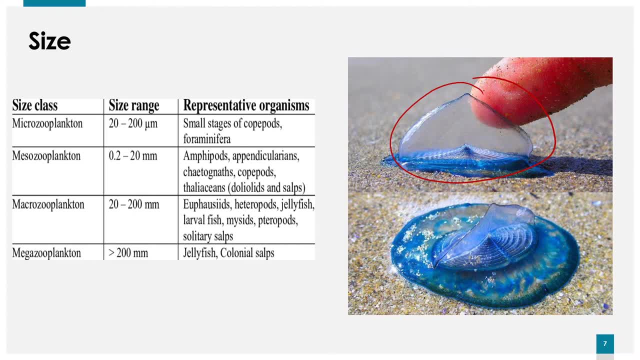 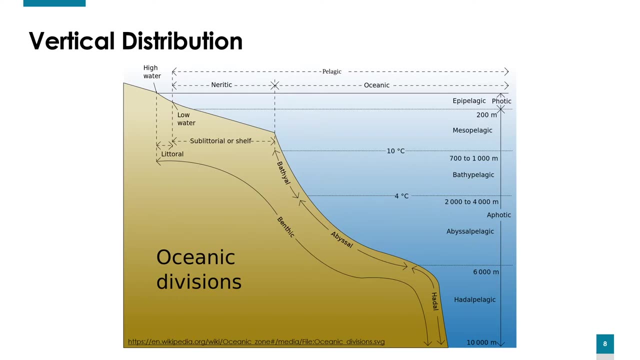 And so when they wash up ashore they can't help it And they just eventually dry up. But these are also good examples of types of megazoplankton Right. So there are many species of zooplankton that live in the euphotic, or on this diagram we have the photic zone of the ocean. 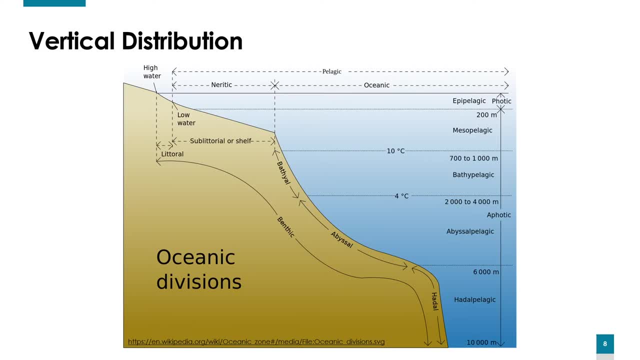 And so what that means is that they live at depths at which Sunlight can penetrate and feeding on phytoplankton, and phytoplankton are restricted to a specific part of the ocean because they photosynthesize, And in order to photosynthesize, they need sunlight. 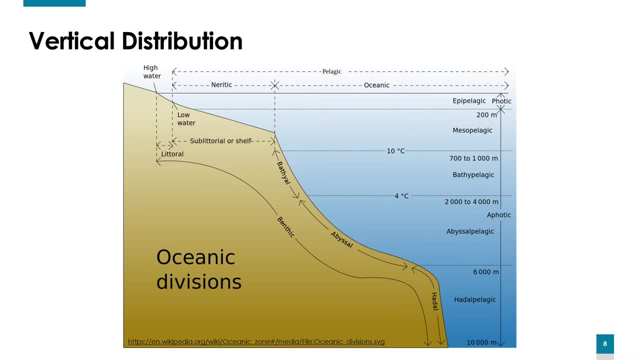 And so in the photic zone We see that that zone is not very deep. We're looking at just right here, Excuse me, And in the marine ecosystem the photic zone can range in depth between maybe roughly 30 meters when you're looking more coastal or inland. 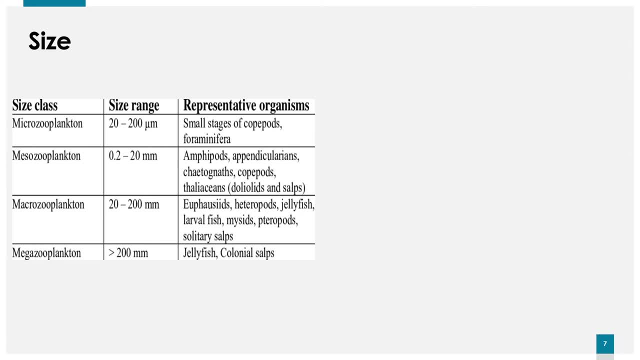 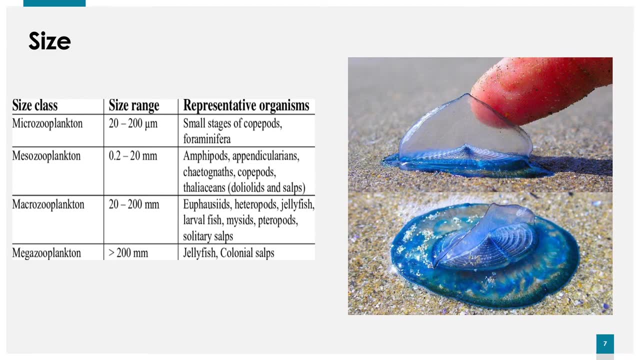 And then another example that we have are the whales. These are by the wind sailor or Villala Villala, And these I have seen wash up ashore in San Diego And they've washed up by the tens of thousands And when they dry up they just look like little pieces of blue plastic wrap. 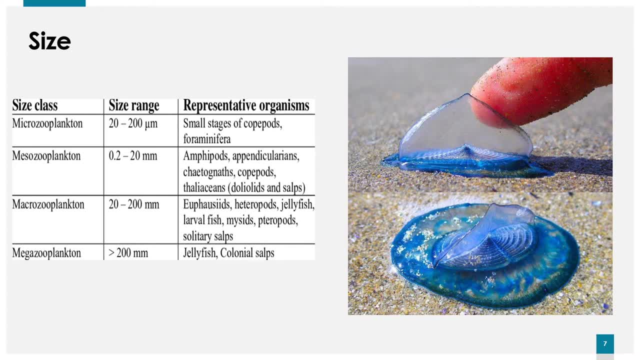 And they just kind of fly away with the breeze when they dry up And so, but they wash ashore because they they use this part of their body like a sail and are propelled along the top of the ocean or the surface of the ocean from the wind or by the wind. 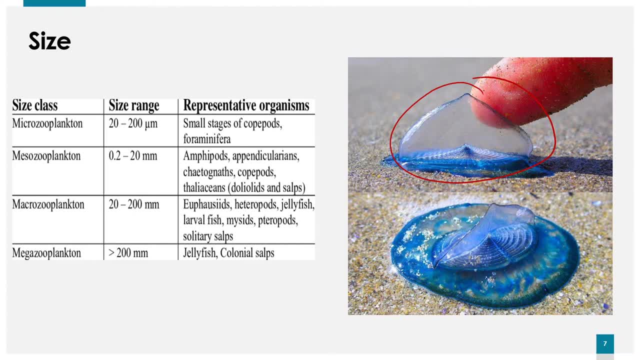 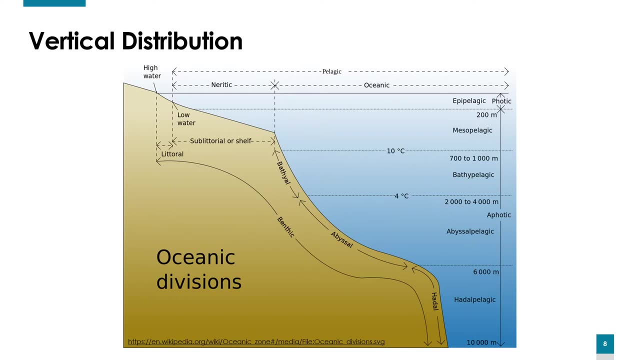 And so when they wash up ashore, they can't help it And they just eventually dry up. But these are also good examples of types of mega zooplankton Right. So there are many species of zooplankton that live in the euphotic or on this diagram. 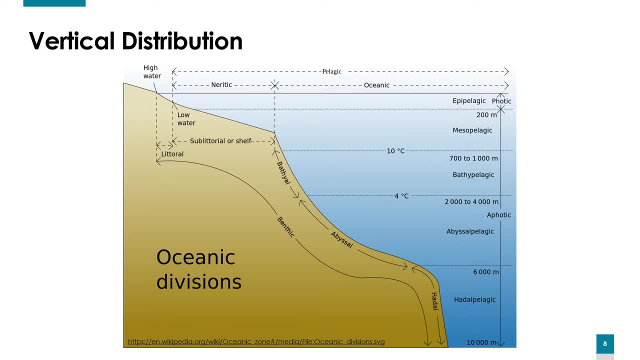 we have the photic zone of the ocean, And so what that means is that they live at depths at which sunlight can penetrate and feeding on phytoplankton, And phytoplankton are restricted to a specific part of the ocean because they photosynthesize. 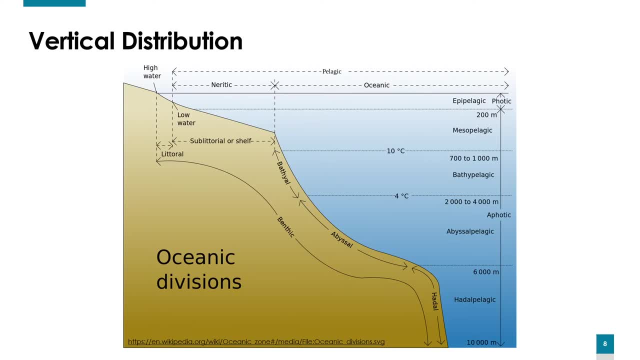 And in order to photosynthesize they need sunlight, And so in the photic zone we see that that zone is not very deep. We're looking at just right here, Excuse me, And in the marine ecosystem the photic zone can range in depth between maybe roughly 30 meters when you're looking more coastal or inland. 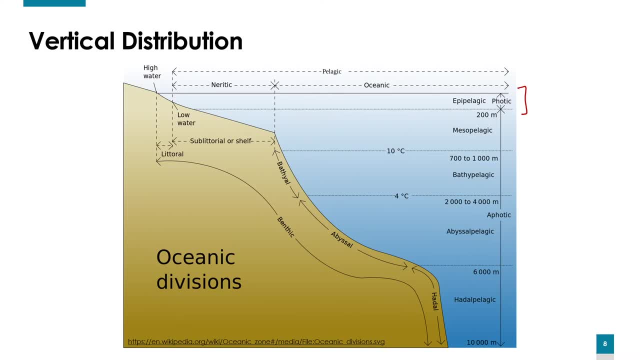 Or when you are further out in the ocean. the photic zone can extend between 100 and 200 meters out in depth, And so many different types of zooplankton will live and thrive within the photic zone. However, zooplankton do live and exist in different parts of the water column and not specifically just photic zone. 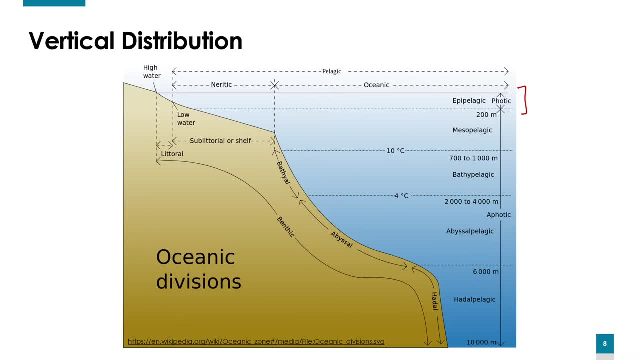 Or when you are further out in the ocean. the photic zone can extend between 100 and 200 meters out in depth, And so many different types of zooplankton will live And thrive within the photic zone. However, zooplankton do live and exist in different parts of the water column and not specifically just photic zone. 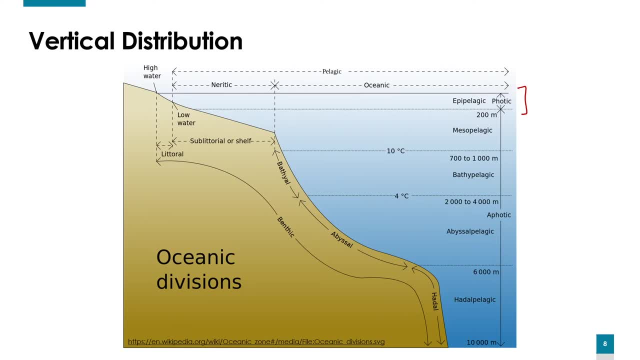 And what we actually learn a little bit later. One of our grad students in the lab that I work in are studying So plankton that live and thrive in the- Use my pen again- Mesopelagic zone. And so there are zooplankton that live down there. 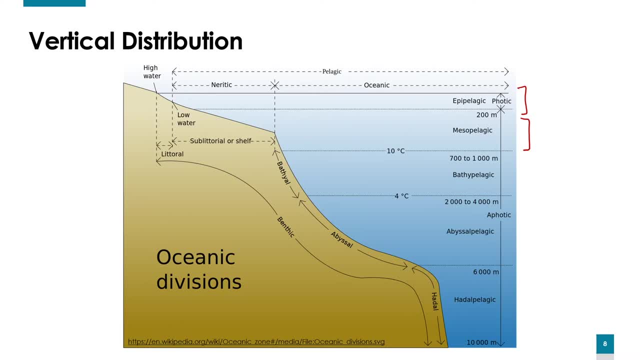 And so When you look at the vertical distribution of these zooplankton and where they live, Many variables go into play on to why they exist at different depths in the water column, and food availability is a key factor, along with oxygen saturation. 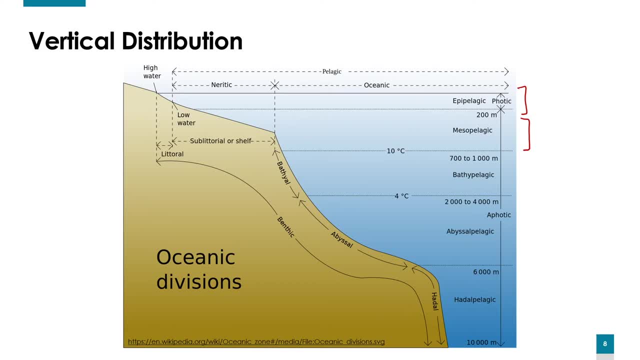 There's another one, The amount of light, Sunlight available is another one, And so, in turbulence, and nutrients, The amount of nutrients available, or others, And so there's many different reasons why zooplankton will exist at various depths within the water column. 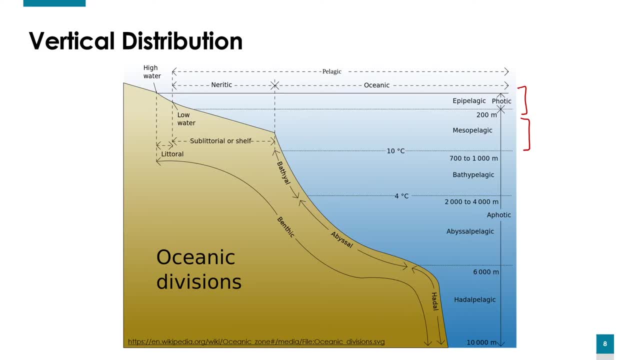 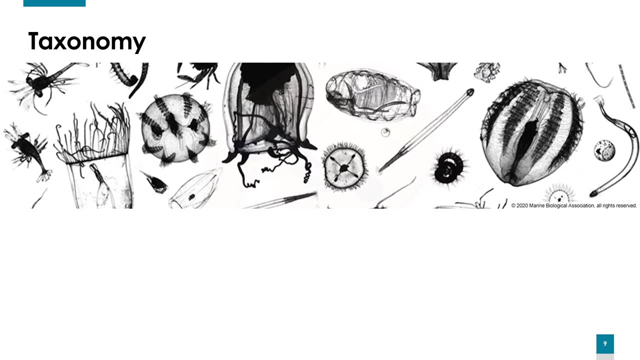 And this is a and could be a really great lecture to expand on later If someone wanted to. Okay, So let's talk about taxonomy and the different phylums And sub phylums of zooplankton And the next couple of slides. 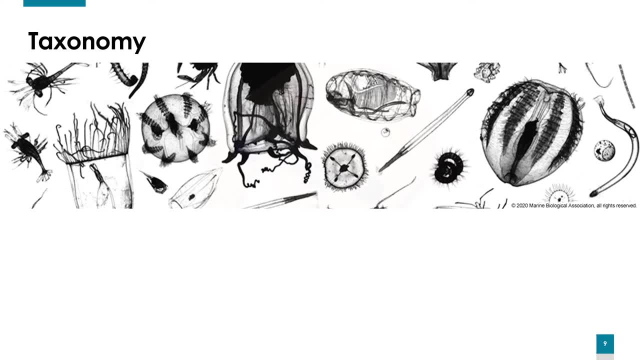 I'll talk about these different groups and show a few examples of what they would look like And examples of the size that they can reach, And so the different groups that we'll be talking about today include Crustaceans And Darien's. 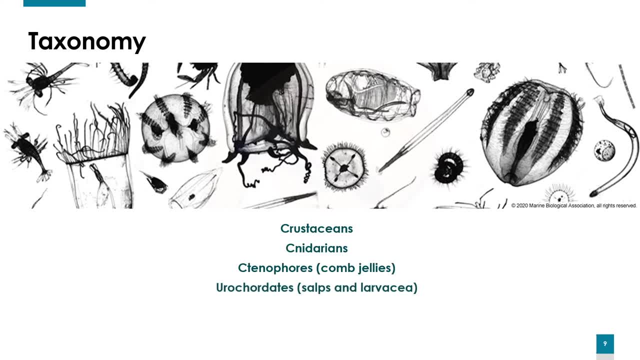 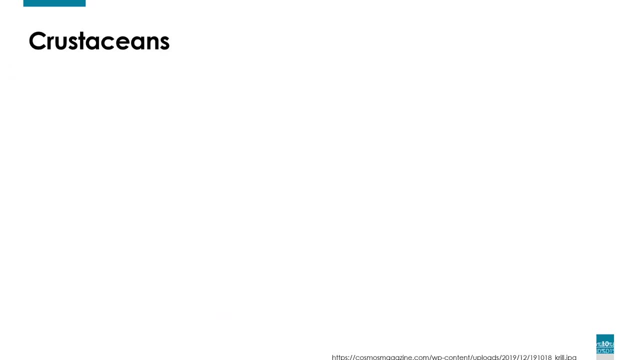 Tina force, Aka, comb jellies Your coordinates. Salts and larvae. Cia Worms could be arrow worms or polykeets, Terrapods, which are planktonic snails And protests. All right. So first up are crustaceans. 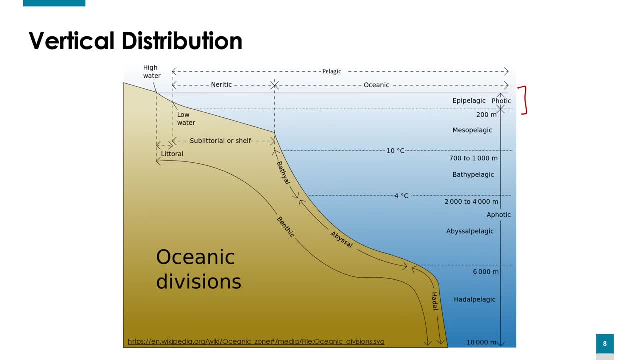 And what we actually learn a little bit later. one of our grad students in the lab that I work in are studying zooplankton that live and thrive in the mesopelagic zone, And so there are zooplankton that live down there. 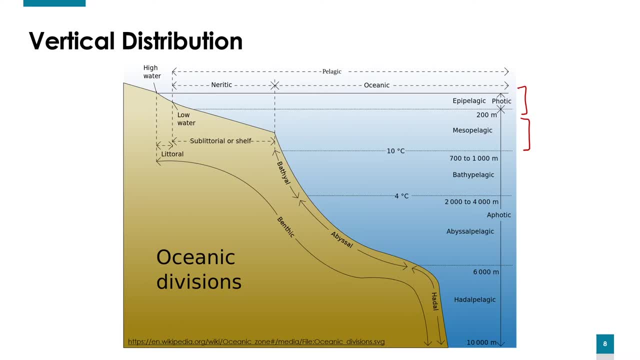 And so when you look at the vertical distribution of these zooplankton and where they live, many variables go into play on to why they exist at different depths in the water column, And food availability is a key factor, along with oxygen saturation is another one. 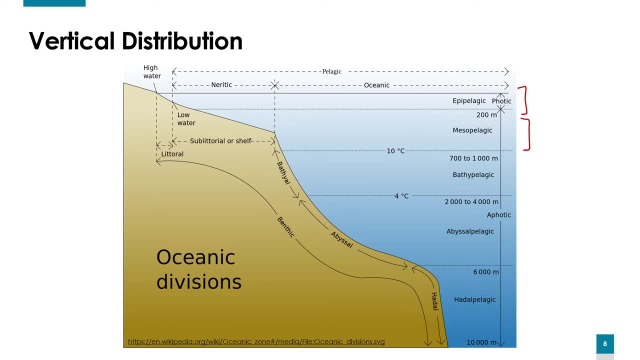 The amount of light- sunlight- available is another one, And so, in turbulence. and nutrients, the amount of nutrients available are others, And so there's many different reasons why zooplankton live, But the fact is that zooplankton will exist at various depths within the water column. 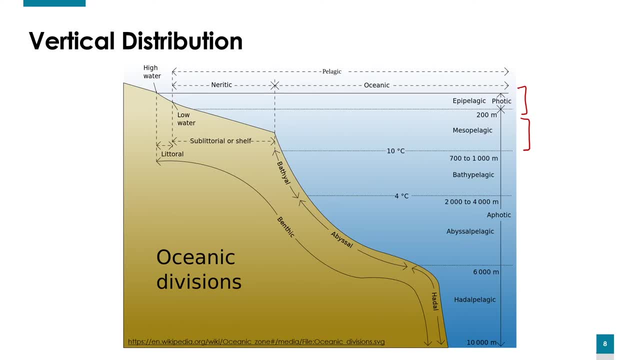 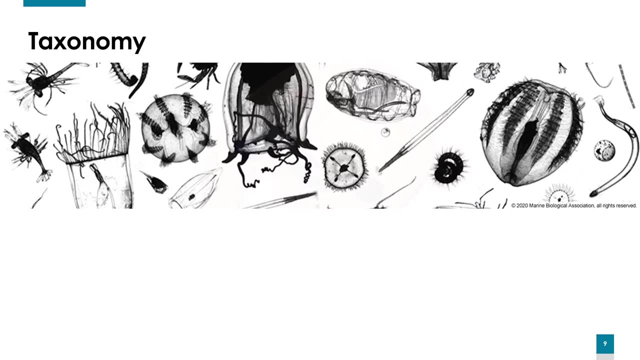 And this could be a really great lecture to expand on later if someone wanted to. Okay, so let's talk about taxonomy and the different phylums and subphylums of zooplankton. In the next couple of slides I'll talk about these different groups and show a few examples of what they would look like. 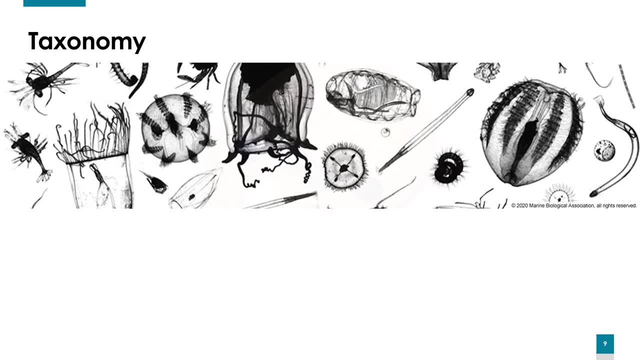 and examples of the size that they can reach. So the different groups that we'll be talking about today include crustaceans, nadarians, ctenophores, aka comb, jellies, uracordates, salps and larvaceae. 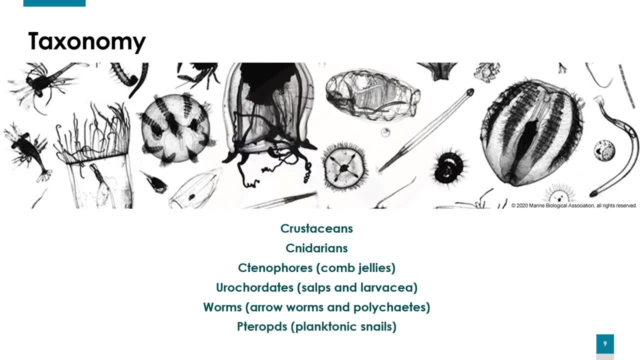 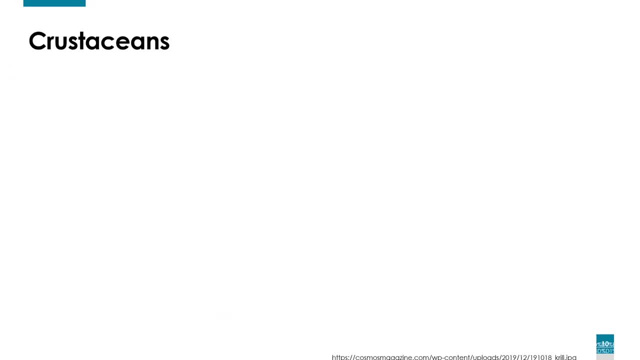 Worms could be arrowworms or polychaetes, Pteropods, which are planktonic snails, And protists. Alright, so first up are crustaceans And crustaceans. they have an external chitin cell. 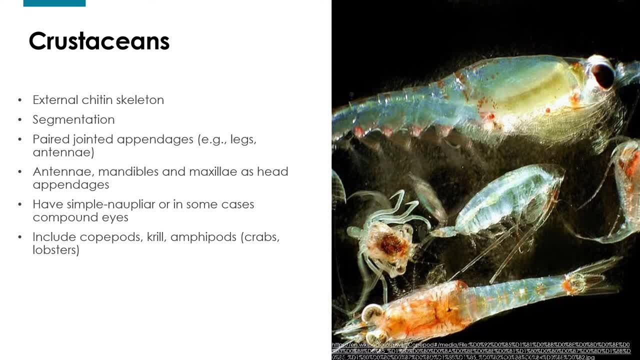 And the word chitin might be familiar for some of you who are bug enthusiasts, Because insects use chitin to create the exoskeleton that they need in order to protect the insides, And then crustaceans also have segmentation that runs along their body. 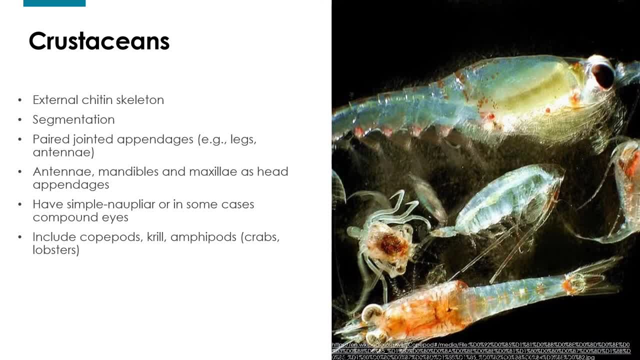 And crustaceans. They have an external chitin skeleton- And the word chitin might be familiar for some of you who are bug enthusiasts, because insects use chitin to create the exoskeleton that they need in order to protect the insides. 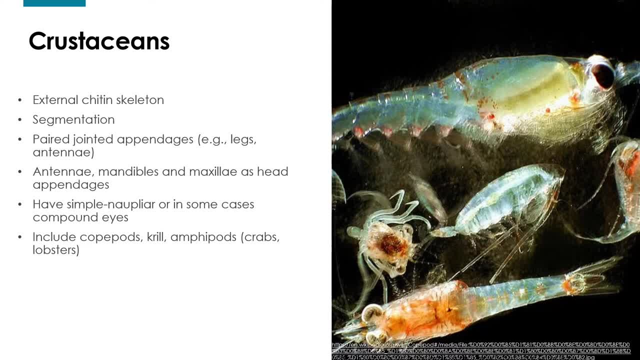 And And then crustaceans also have segmentation that runs along their body. The image here on the right: you can see really nicely the segmentation along the tail. And the segmentation allows for the copepods and krill amphipods to be able to bend and 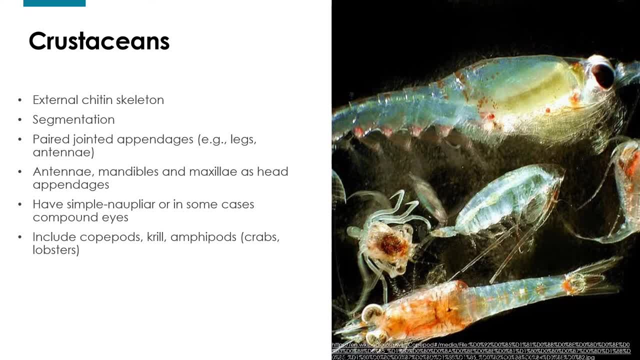 move around in the water. They also consist of paired, jointed appendages, So the legs and the antennae, And along with the antennae are mandibles and maxillae. That, That, That, That, That, That That. 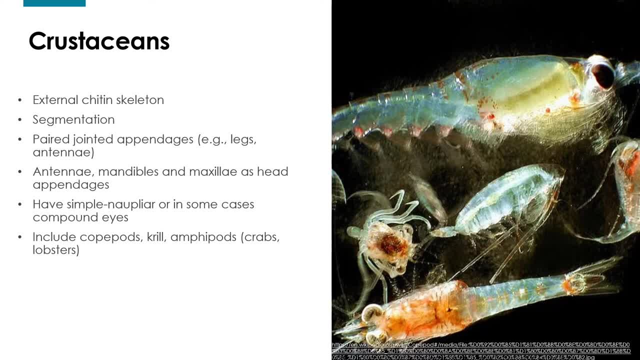 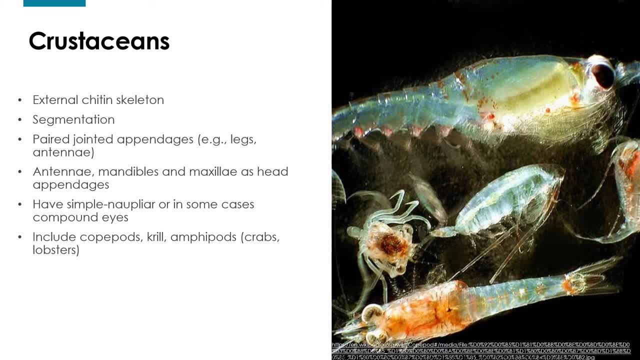 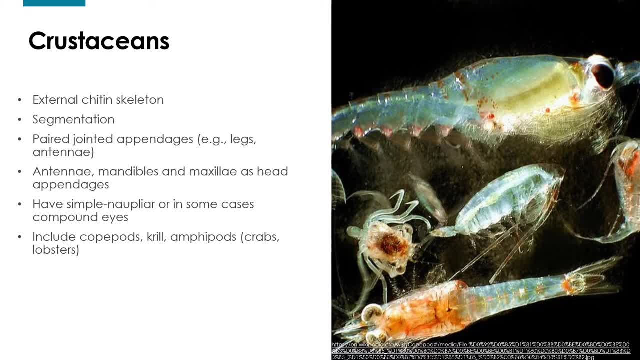 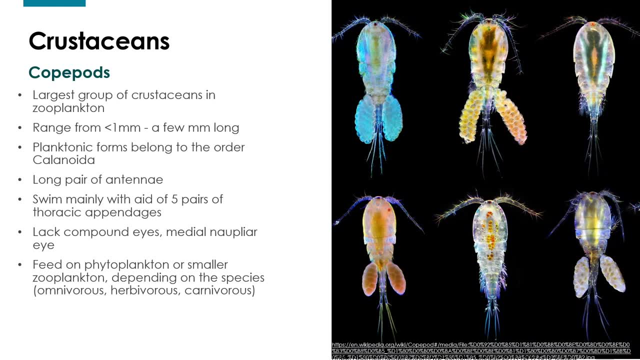 and amphipods, which are crabs and lobsters Next. So one group of crustaceans we'll look at are copepods, and they are the largest group of crustaceans in the zooplankton world and the range of size is around less than a millimeter to around a few millimeters long. 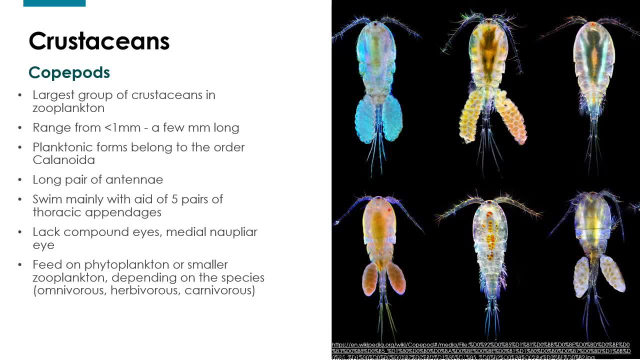 And so planktonic forms belong to the order of calanoida, which I see very often in the samples that I scan. They have a long pair of antennae, which you can see on the image here, and they're very beautiful. They swim mainly with the aid of five pairs of thoracic appendages. 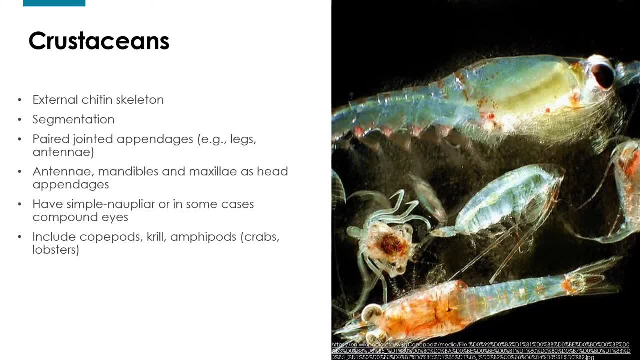 The image here on the right. you can see really nicely the segmentation along the tail. And the segmentation allows for the copepods and krill Amphipods to be able to bend and move around in the water. They also consist of paired, jointed appendages. 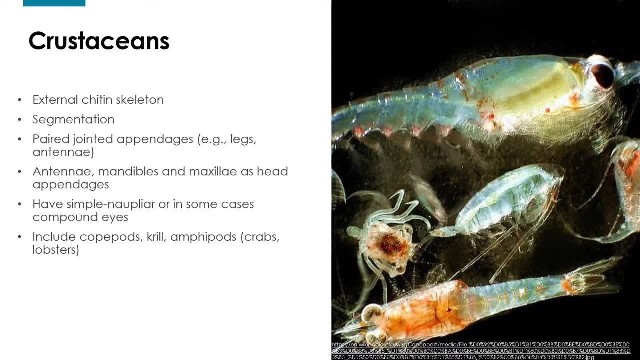 So the legs and the antennae, And along with the antennae are mandibles and maxillae that are part of the head appendages. So the maxillae: they serve to transport food to the mandible But also assist in the filtration- water filtration. 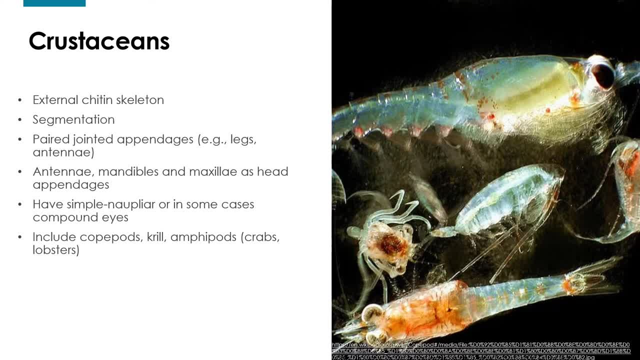 And sometimes also play a role in cleaning and grooming, And so crustaceans have a simple noplar, in some cases compound eyes, And these eyes help with sensing the direction of where sunlight is coming from. And crustaceans include copepods, krill and amphipods, which are crabs and lobsters. 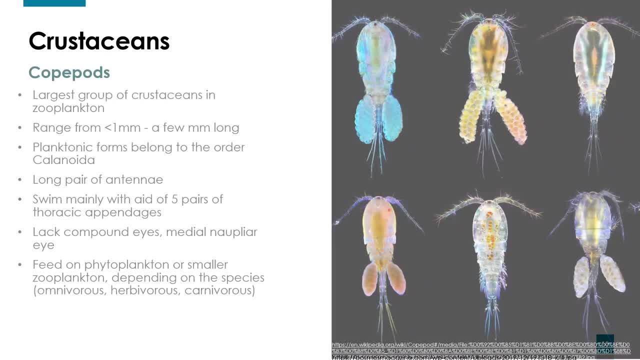 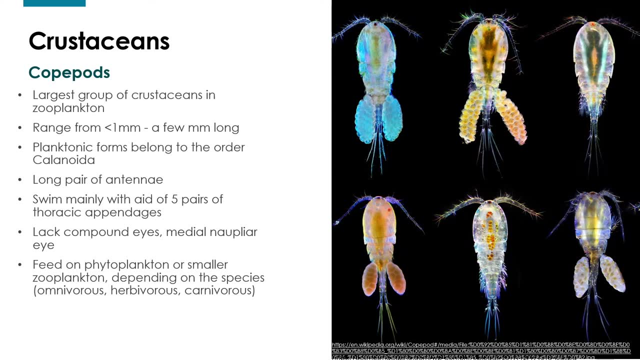 Next. So one group of crustaceans we'll look at are copepods, And they are the largest group of crustaceans in the zooplankton world, And their range of size is around less than a millimeter to around a few millimeters long. 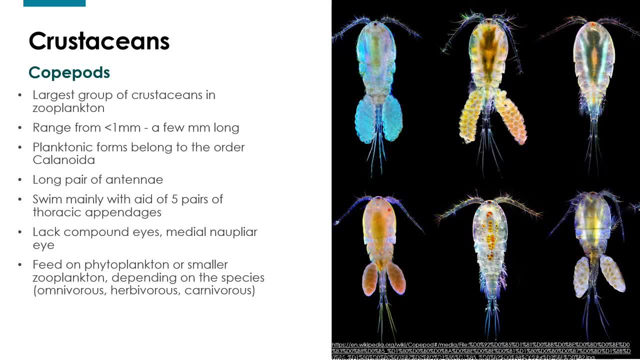 And so planktonic forms belong to the order of calanoida, which I see very often in the samples that I scan. They have a long pair of antennae, which you can see on the image here, and they're very beautiful. 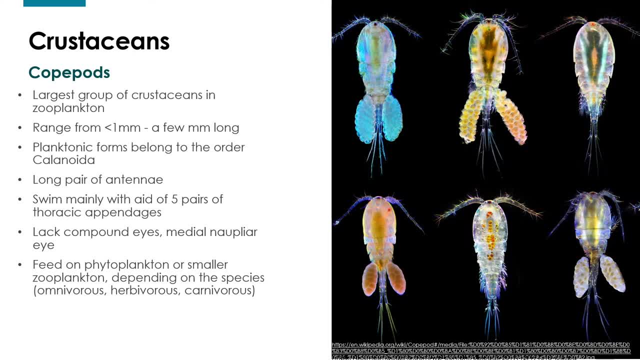 They swim mainly with the aid of five pairs of thoracic appendages And they lack compound eyes, And so they actually have medial noplar eyes. And so what this means? if you look here, this is a good example. The medial noplar eyes are a simple type of eye that consists of three photoreceptor units. 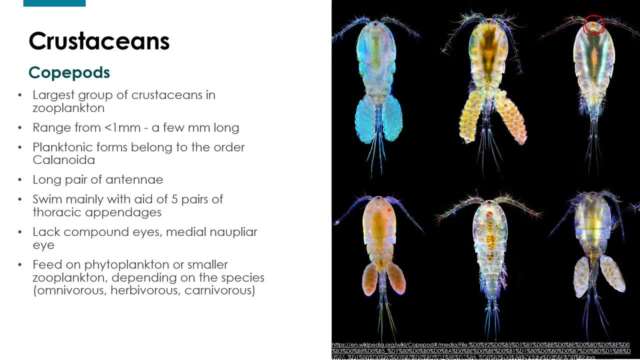 And these units help the copepod be able to tell the direction of light, The direction of where the light is coming from- So again sunlight. And they feed on phytoplankton or smaller zooplankton depending on the species. 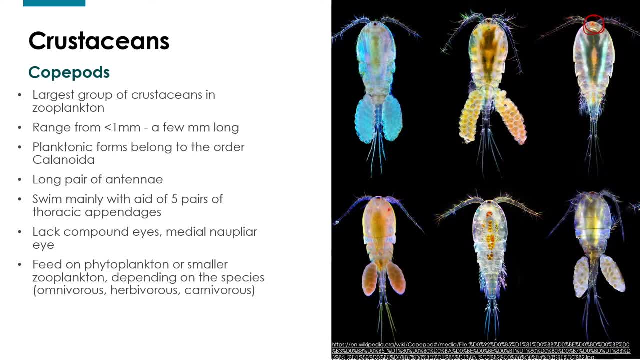 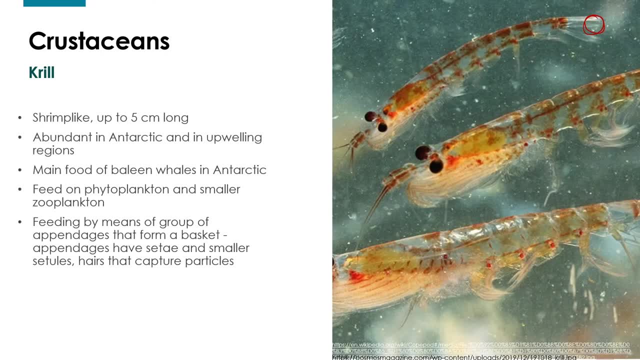 But from what we knew about their diet earlier, they can be omnivorous, herbivorous or carnivorous. Then next group are krill, And so krill are shrimp-like. We probably have seen these a lot, And if you've seen any nature documentaries or like Planet Earth and stuff- 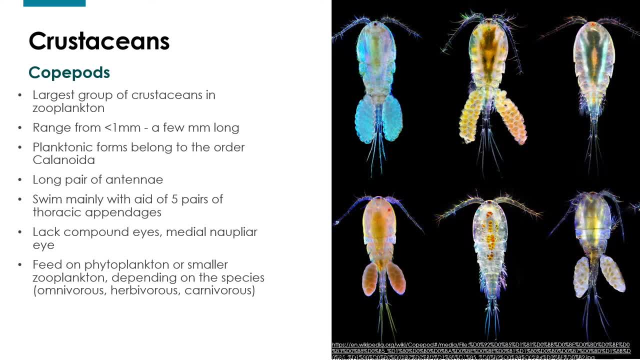 and they lack compound eyes, and so they actually have medial-nopular eyes, And so what this means. if you look here, this is a good example. The medial-nopular eyes, um, are a simple type of eye that consists of three photoreceptor units, and these units help. 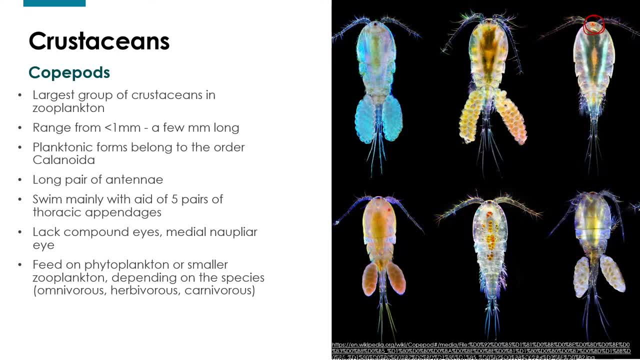 the copepod be able to tell the direction of where the light is coming from- So again sunlight- And they feed on phytoplankton or smaller zooplankton depending on the species, but from what we knew about their diet earlier, they can be omnivorous, herbivorous or carnivorous. 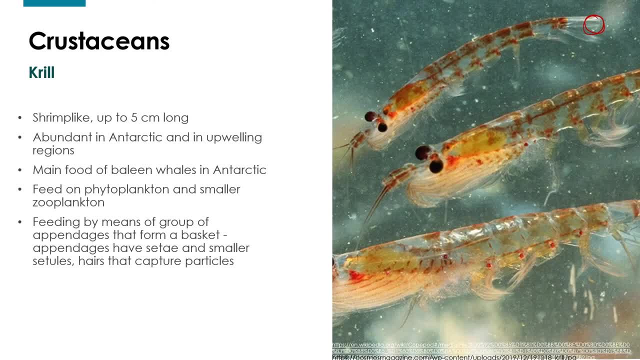 And then next group are krill, And so krill are shrimp-like. We probably have seen these a lot, and if you've seen any nature documentaries or like Planet Earth and stuff, you've probably seen those giant swarms of krill in the ocean and the majestic baleen whale jumping through. 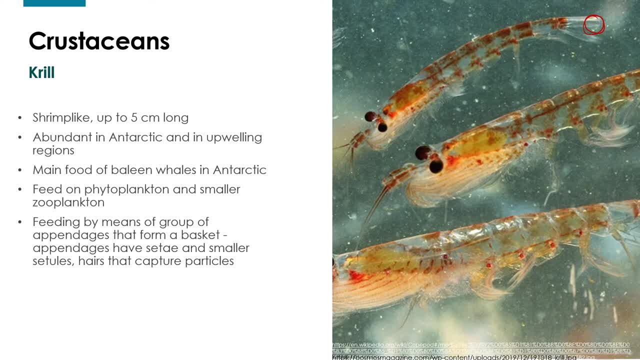 swimming through the ocean to gobble up all of the krill right. So krill are a very important food source for many animals in the ocean and they are abundant in the ocean and they are abundant in the ocean. They are abundant in the Antarctic and in upwelling regions. so this is also a main reason why many 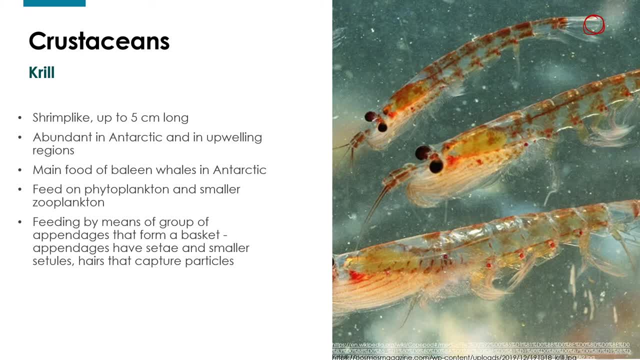 large marine animals will migrate to the Antarctic or to colder regions because they're looking for this krill to eat, And so, again, they're the main food of baleen whales in the Antarctic. Krill feed on phytoplankton and other types of zooplankton, and they feed by means of a group of appendages. 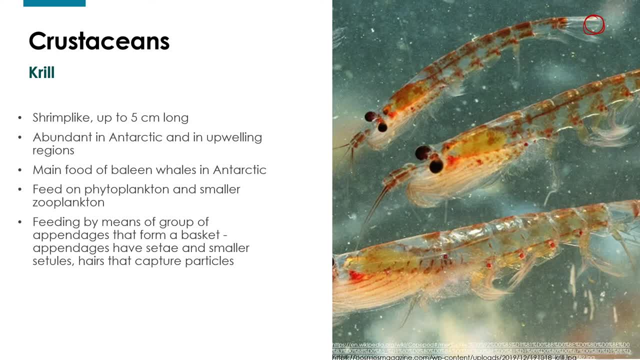 that form a basket, And so these appendages will help them move and filter water towards their mandibles so that they can quickly feed in a small space around them, versus having to venture out far swim further to find their prey. They just kind of swoop in and draw the water in and filter and draw the 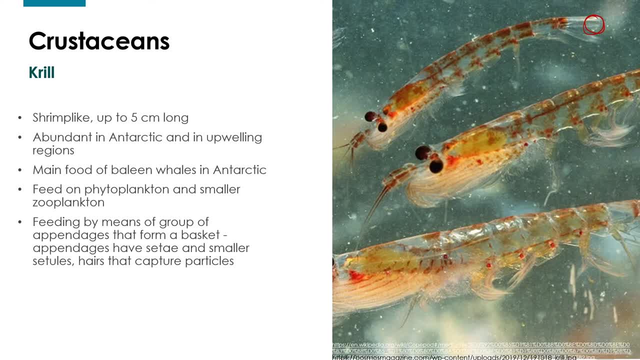 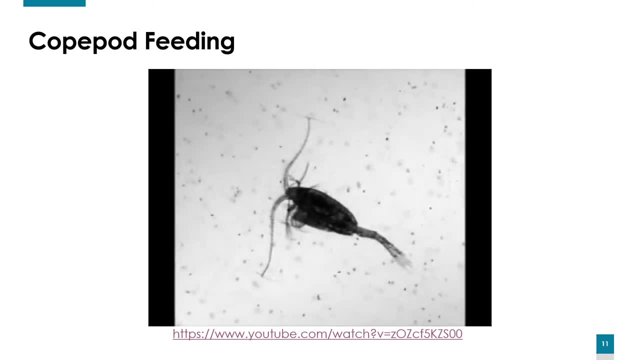 water into their mandibles to feed. So what I wanted to show you quickly was a video of a particular type of copepod. It's called Matridia longa, And in this video what's happening is that- and it's a slow-mo, which is good, because you really get to see it in action- 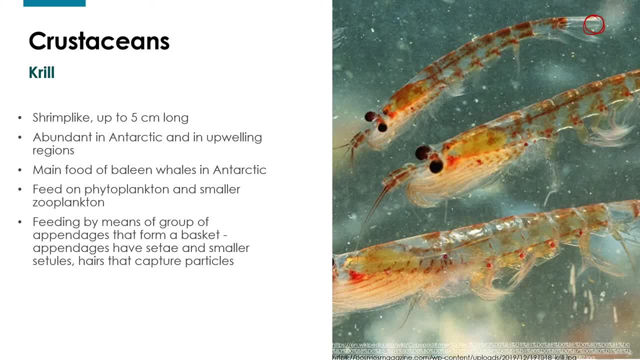 you've probably seen those giant swarms of krill in the ocean And the majestic baleen whale jumping through, swimming through the ocean to gobble up all of the krill right. So krill are a very important food source for many animals in the ocean. 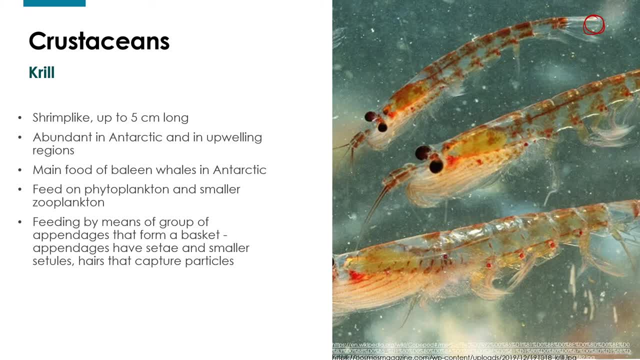 And they are abundant in the Antarctic and in upwelling regions. So this is also a main reason why many large marine animals will migrate to the Antarctic Or to colder regions, because they're looking for this krill to eat, And so, again, they're the main food of baleen whales in the Antarctic. 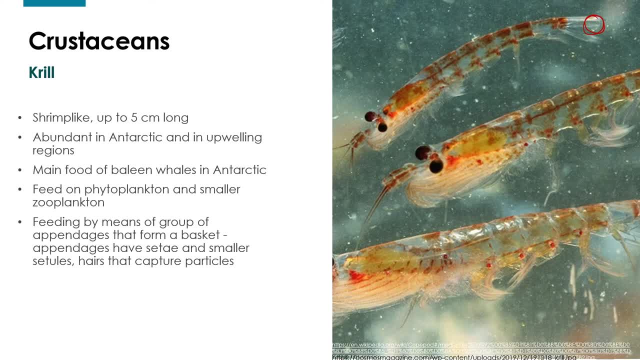 Krill feed on phytoplankton and other types of zooplankton, And they feed by means of a group of appendages that form a basket, And so these appendages will help them move and filter water towards their mandibles so that they can quickly feed in a small environment. 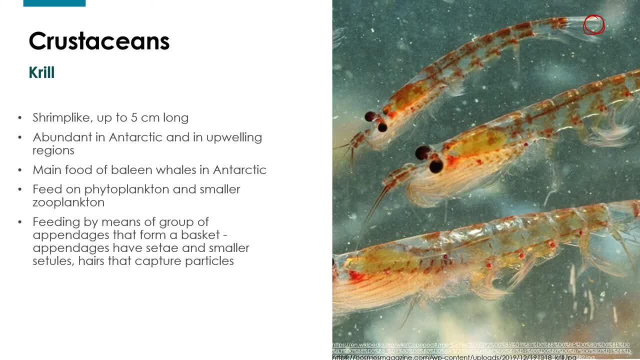 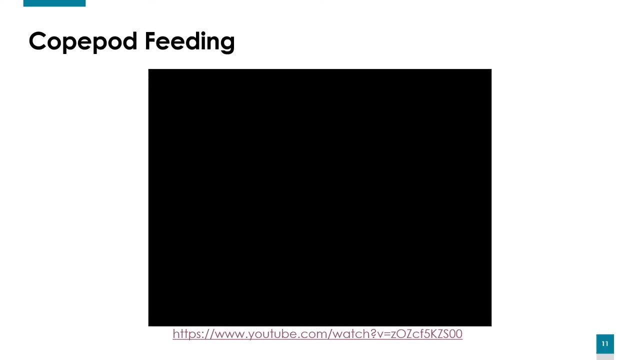 A small space around them versus having to venture out far, swim further to find their prey. They just kind of swoop in and draw the water in and filter and draw the water into their mandibles to feed. Okay, so what I wanted to show you quickly was a video of a particular type of copepod. 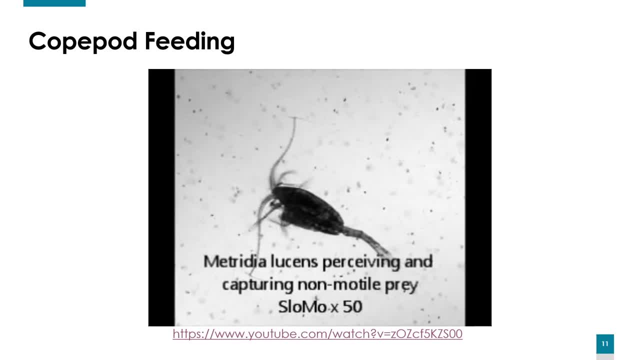 It's called metridia longa And in this video what's happening is that- and it's a slow-mo, which is good because you really get to see it in action- It detects the phytoplankton And you should see it coming up just right here. 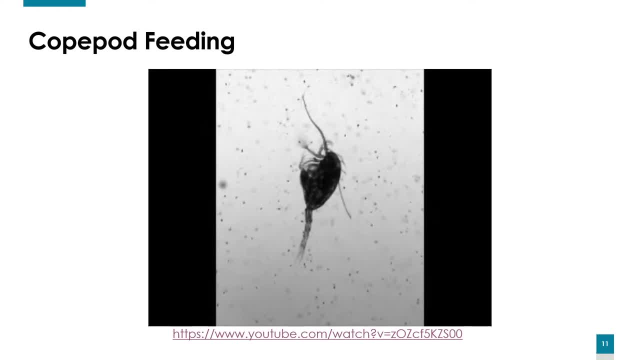 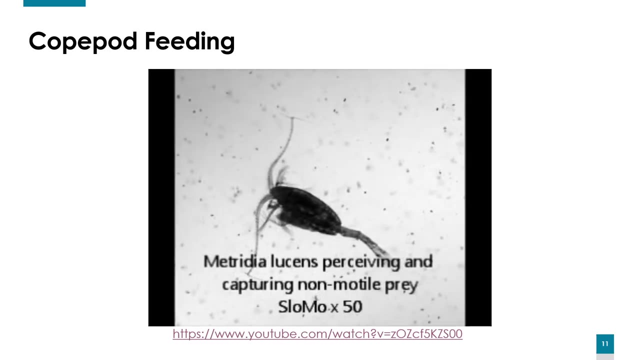 So what happens after it detects the phytoplankton is that it triggers what's called an attack response. And so the copepod. what it's going to do is it creates a suction to draw in. You can see it's using all of its appendages to draw in water and phytoplankton in its mouth to feed. 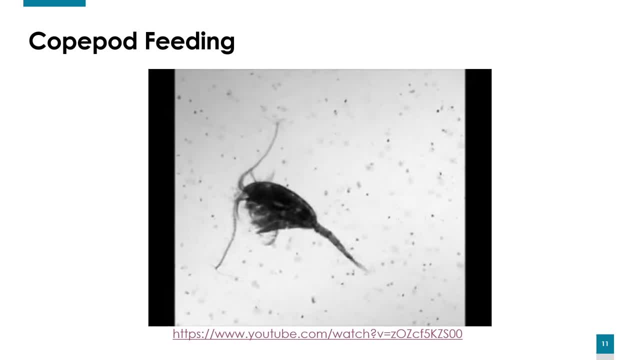 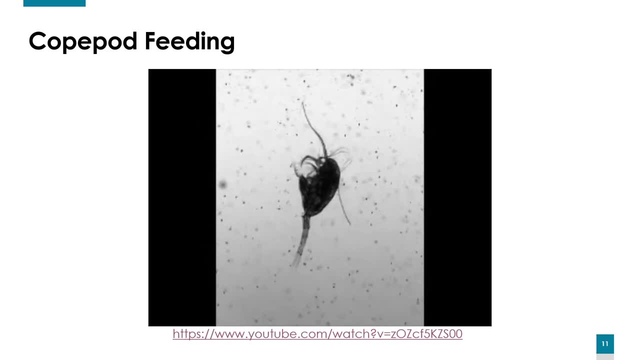 So a single copepod can consume up to 373,000 phytoplanktons per day And they generally have to clear the equivalent to about a million times their own body volume of water every day to cover just their nutritional needs. And when you think about how much time that takes and what that process would look like, 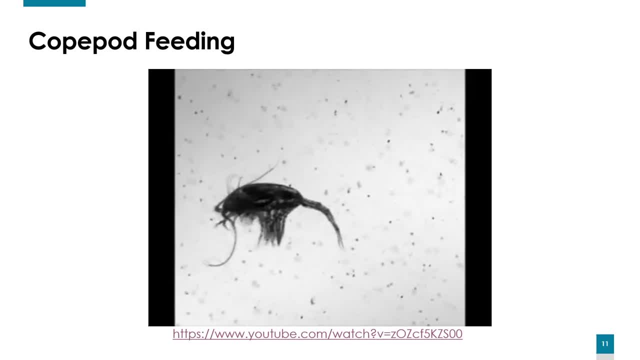 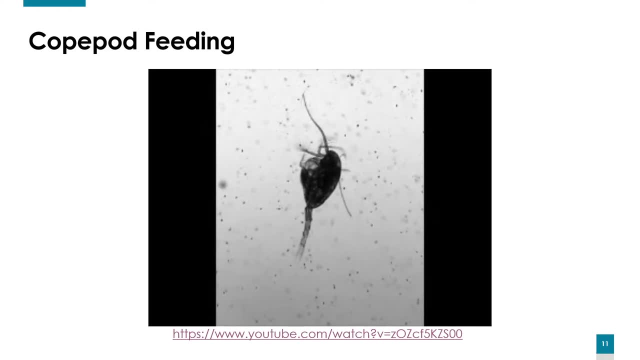 it detects the phytoplankton, And you should see it coming up just right here. So what happens after it detects the phytoplankton is that it triggers what's called an attack response, And so the copepod. what it's going to do is it? 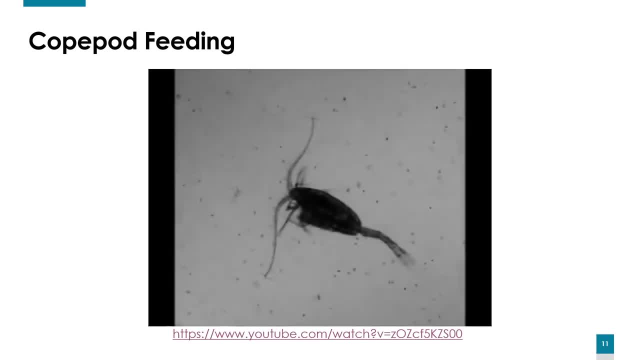 creates a suction to draw in. You can see it's using all of its appendages to draw in water and phytoplankton in its mouth to feed, And so a single copepod can consume up to 373,000 phytoplanktons per day. 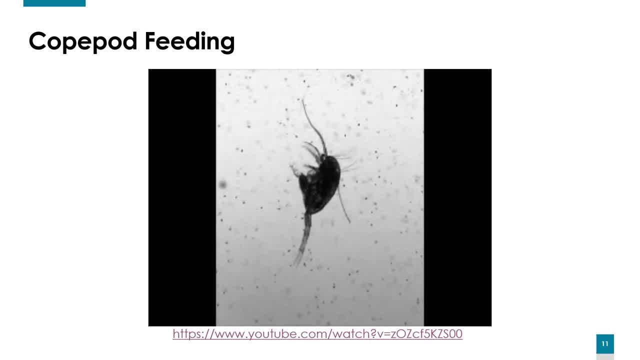 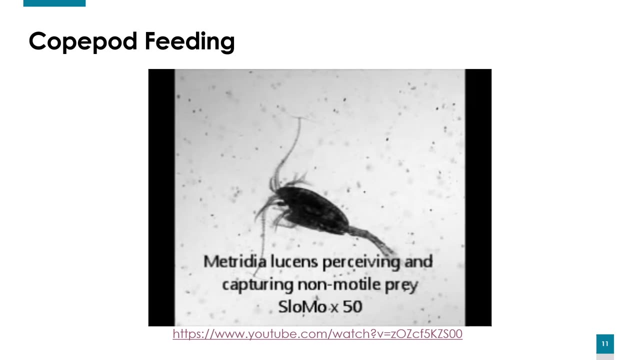 And they generally have to clear the equivalent to about a million times their own body volume of water every day to cover just their nutritional needs. And when you think about how much time that takes and what that process would look like, it is pretty, pretty crazy. 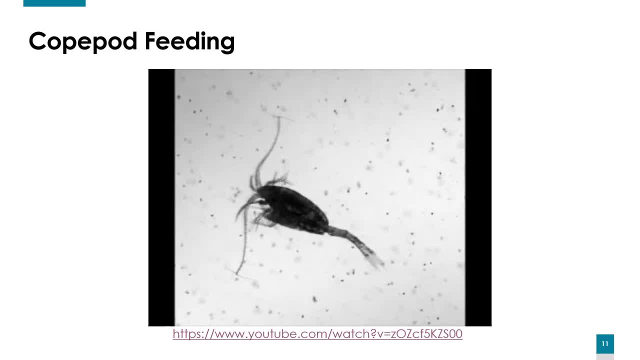 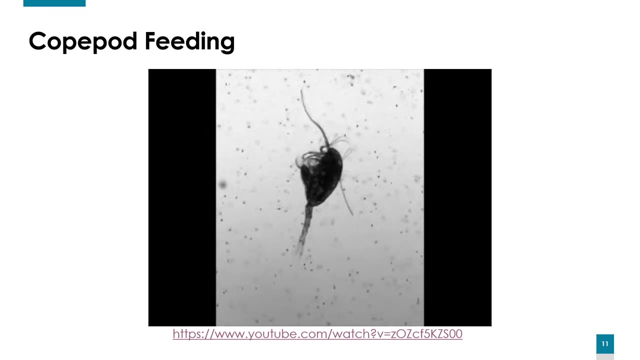 And just imagining how humans would have to sustain themselves. we had to do. that would be a lot of food, And so copepods spend a lot of their time feeding and trying to find food, And so the because they are drifters and they are not able to move around, say, like a fish would, in order to find its food. 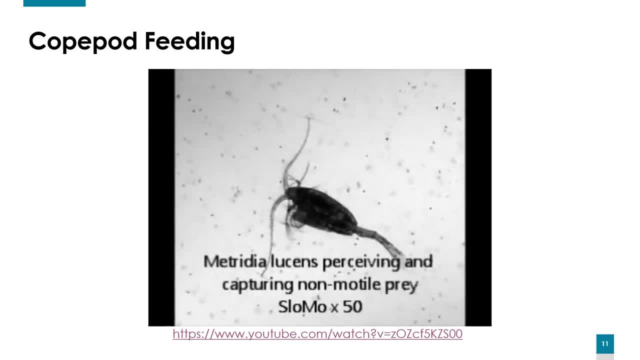 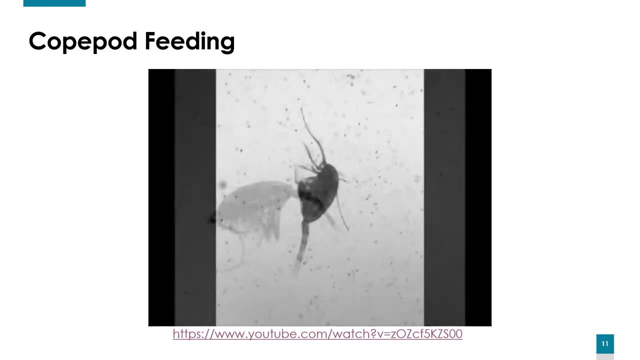 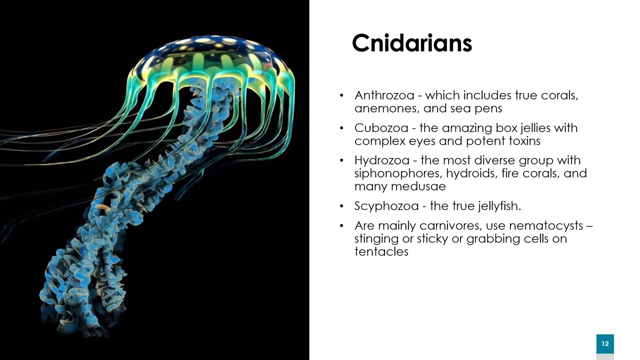 utilize immediately what's surrounding them, And so any advantage to be able to detect phytoplankton or other types of zooplankton and quickly grab and eat them. it would be advantageous to their survival. All right Cnidarians, So Cnidarians are. there are more than 9,000 living species. 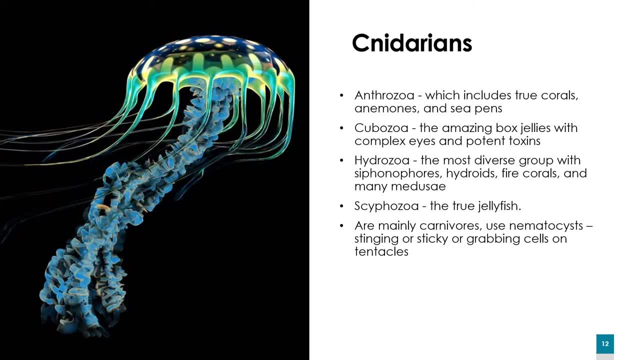 in this group, and they inhabit all marine and some freshwater environments, And these organisms are most abundant, though, and diverse. You'll see a lot of diversity in tropical waters, And Cnidarians are radially symmetrical, so similar parts are arranged. 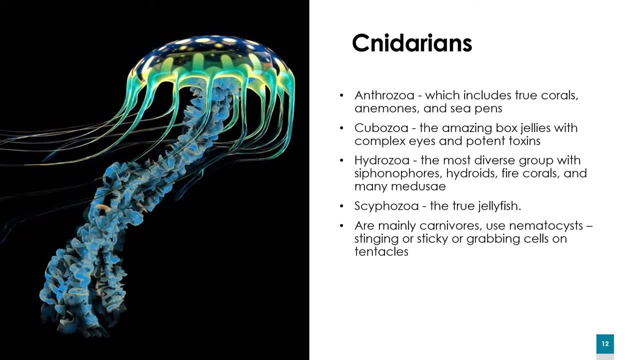 symmetrically around a central disc and they lack cephalization, or like a concentration of sensory organs in the head. We'd say maybe like the bell of, like a jellyfish, for example, And with Cnidarians their bodies have two cell layers rather than three. 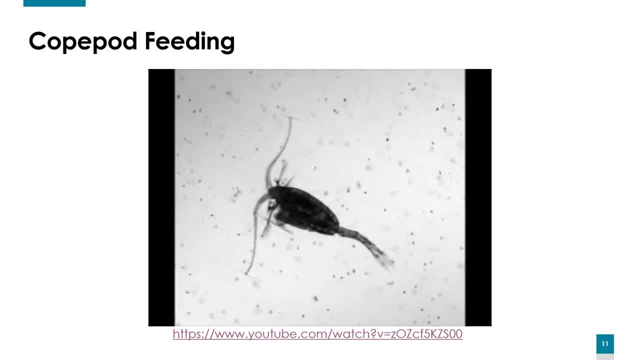 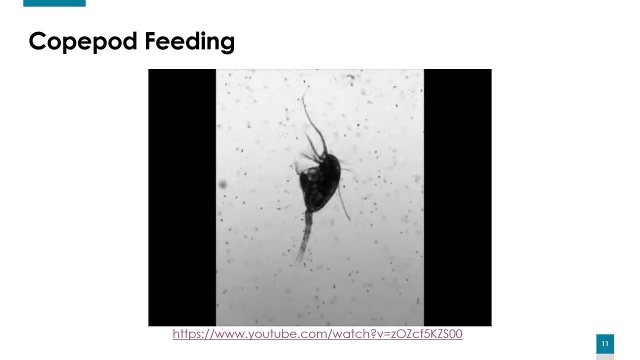 it is pretty, pretty crazy Just imagining how humans would have to sustain themselves. We had to do that. It would be a lot of food, And so copepods spend a lot of their time feeding and trying to find food. And so because they are drifters and they are not able to move around, 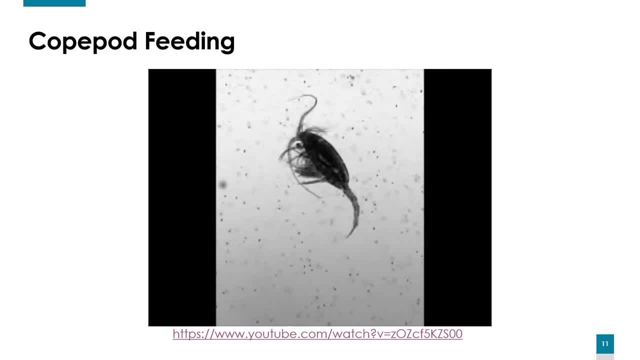 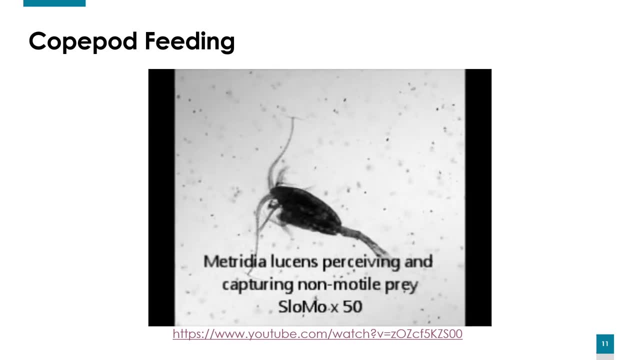 say, like a fish would, in order to find its food, it has to really utilize immediately what's surrounding them, And so any advantage to be able to detect phytoplankton or other types of food or other types of zooplankton and quickly grab and eat them. 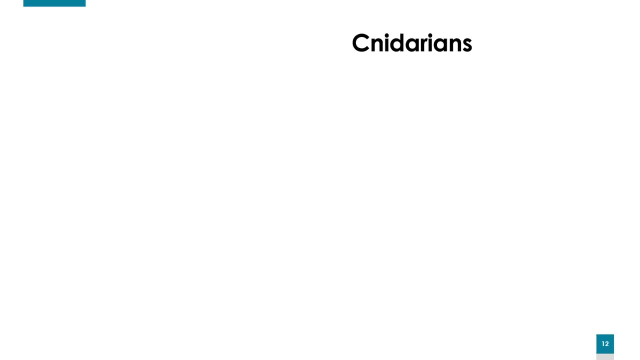 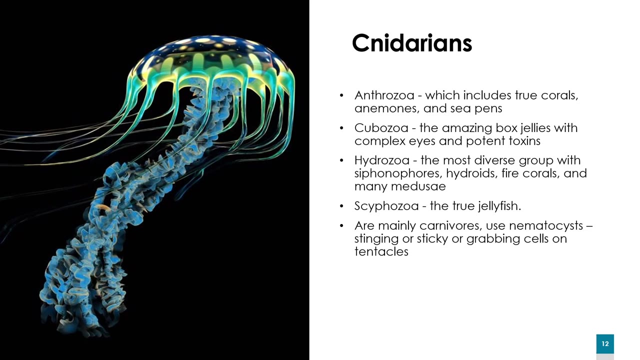 it would be advantageous to their survival. All right, Cnidarians. So Cnidarians are. there are more than 9,000 living species in this group, And they inhabit all marine and some freshwater environments, And these organisms are most abundant, though, and diverse. 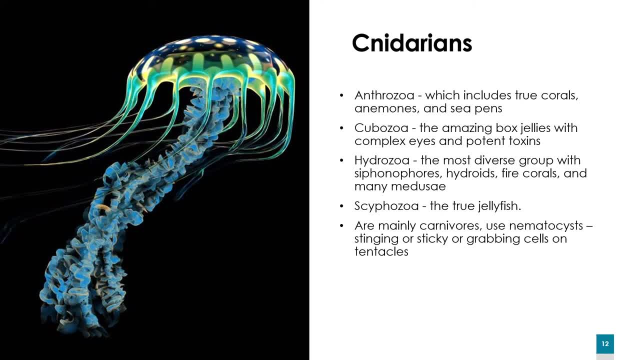 You'll see a lot of diversity. They live in tropical waters And Cnidarians are radially symmetrical, So similar parts are arranged symmetrically around a central disc And they lack cephalization or like a concentration of sensory organs in the head. 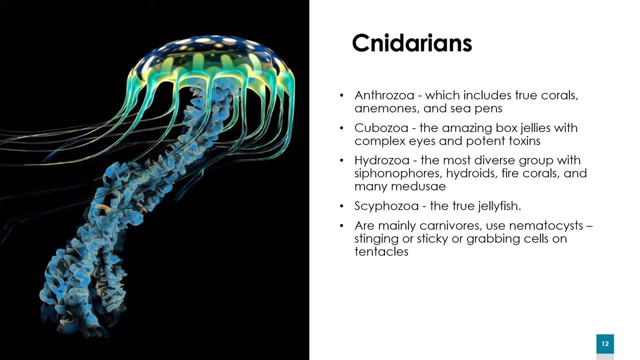 We'd say maybe like the bell of, like a jellyfish, for example. And with Cnidarians their bodies have two cell layers or three cells, And all Cnidarians have what's called nematocysts, which are long, thin, coiled stingers, almost like barbs. 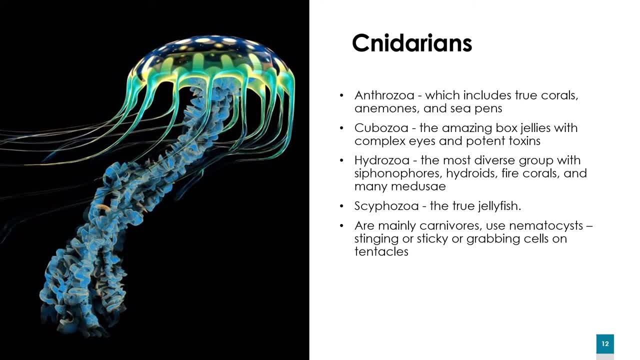 And they can. these barbs inject their prey or some you know helpless swimmer or surfer with venom, And so these tiny darts are propelled out of a special cell And they're used to attack or defend itself from animals larger than itself, or to catch its next dinner. 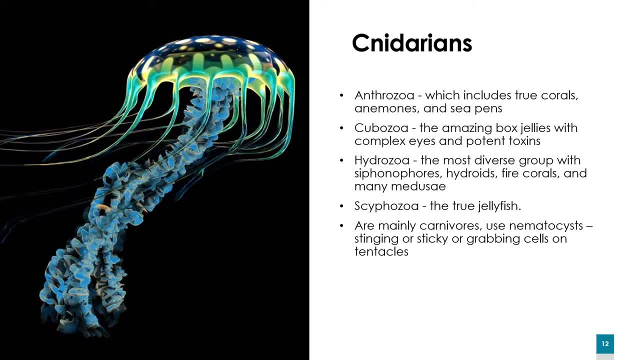 And so Cnidarians can be broken down into four major groups: Anthrozoa, which includes true corals, anemones and sea pens. You have Cubozoa, the amazing box jellyfish R1, or box jellies, excuse me. 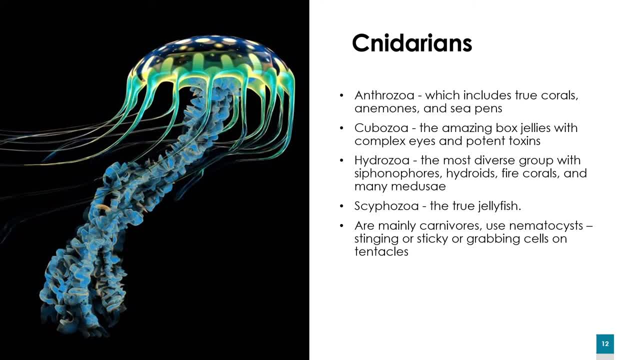 And all Cnidarians have what's called nematocysts, which are long, thin coiled stingers, almost like barbs, And they can, these barbs, inject their prey, or some suspect, You know, helpless swimmer or surfer with venom, And so these tiny darts are propelled. 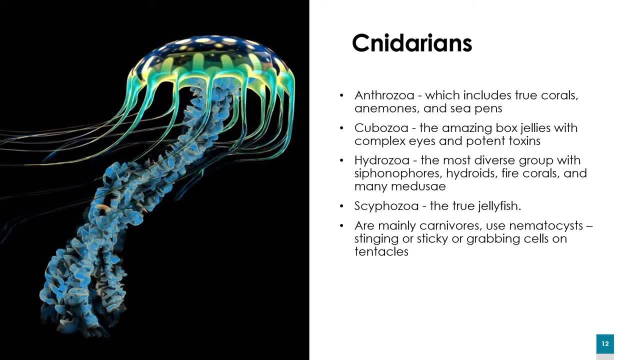 out of a special cell and they're used to attack or defend itself from animals harder than itself, or to catch its next dinner. And so Cnidarians can be broken down into four major groups: Anthrozoa, which includes true corals, anemones and sea pens. You have Cubozoa. 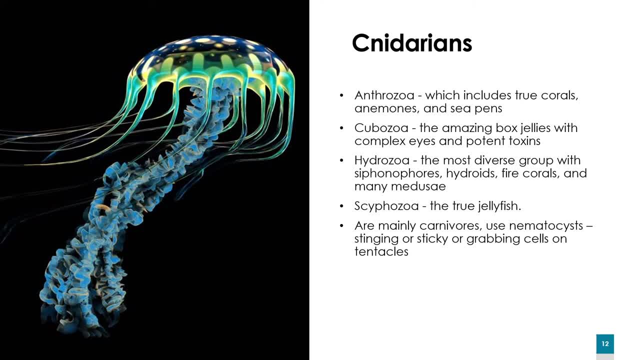 the amazing box jellyfish, Our one or box jellies, excuse me. And next you have Hydrozoa. They're the most diverse group within siphonophores: hydroids, fire corals and many different types of medusae. And then you have 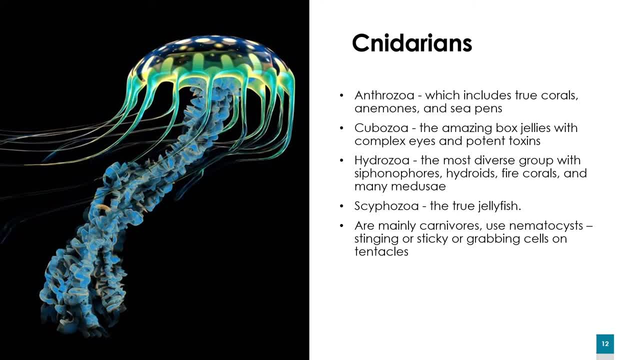 the Siphizoas, or the true jellyfish, And many Cnidarians, are mostly carnivorous And, again, they use nematocysts or stinging cells to catch and grab their prey. And these are probably some of the most familiar for a lot of people when they think of the 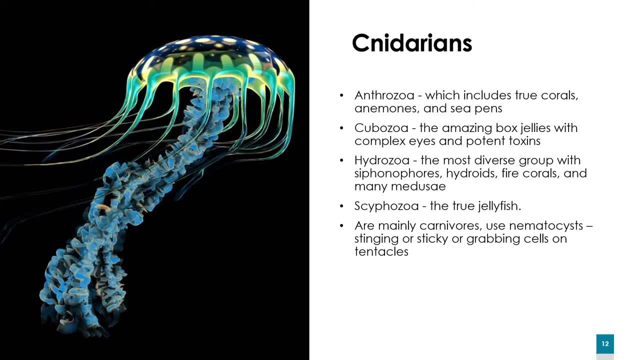 ocean or visiting the aquarium, They'll think, oh, I want to see the jellyfish, I want to see the jellyfish. And so a lot of us have experience at least visiting and seeing these in aquariums, and maybe some of us have experience being stung by a couple of these guys. 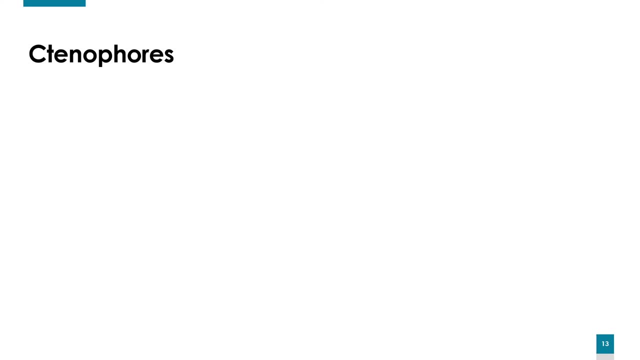 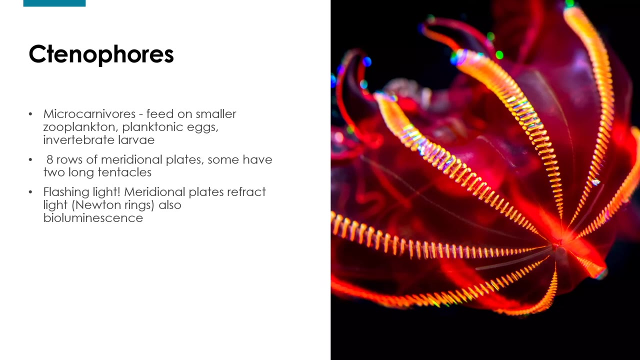 So Cnidophores, they are boobies, Microcarnivores. they like to feed on smaller zooplankton and planktonic eggs and invertebrate larvae. They have eight rows of meridional plates and some have two long tentacles, And so these. 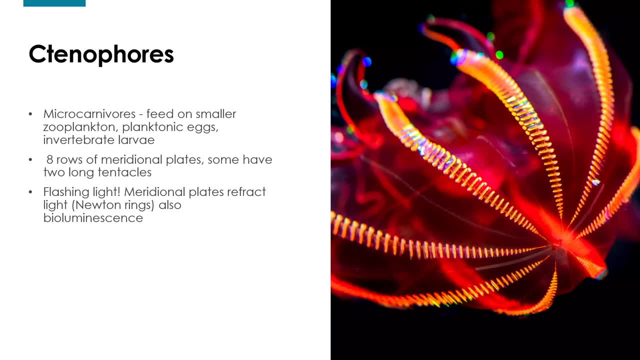 comb rows are fused cilia that are arranged along the sides again of the Cnidophore And they're clearly visible, like we can see in the image on the right, And the cilia they beat together in unison and propel. It helps propel the Cnidophore And they're very, very, very very. 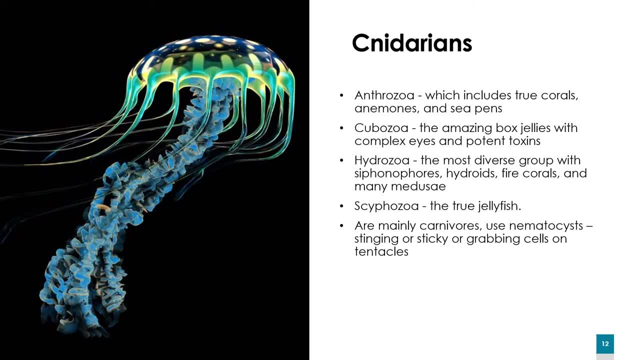 And next you have Hydrozoa. They're the most diverse group within siphonophores: hydroids, fire corals and many different types of medusae. And then you have the Siphozoa, or the true jellyfish. 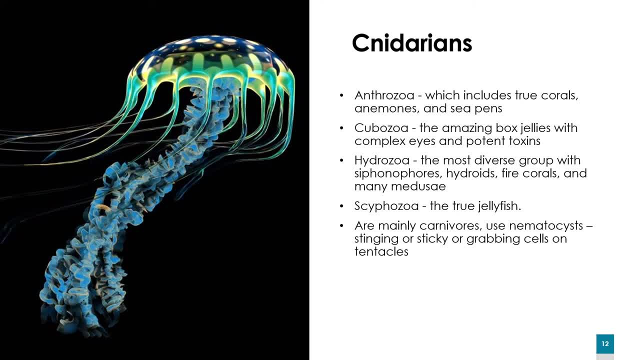 And many Cnidarians are mostly carnivorous And again, they use nematocysts or stinging cells to catch and grab their prey. And these are probably some of the most familiar for a lot of people when they think of the ocean or visiting the aquarium. 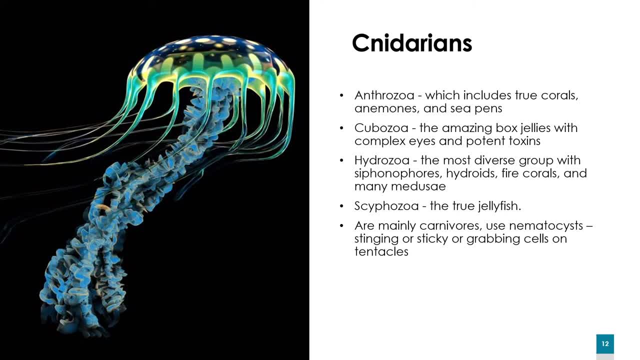 They'll think, oh, I want to see the jellyfish, I want to see the jellyfish, And so a lot of us have experience at least visiting and seeing these in aquariums, And maybe some of us have experience being stung by a couple of these guys. 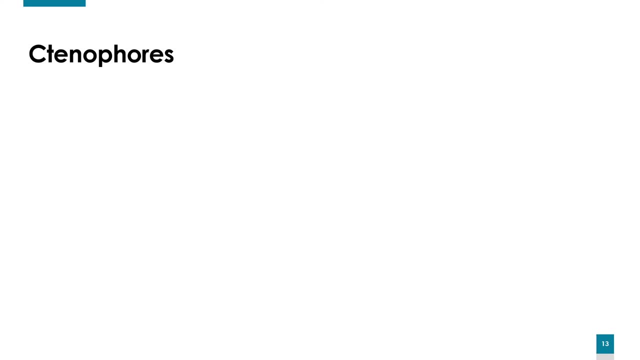 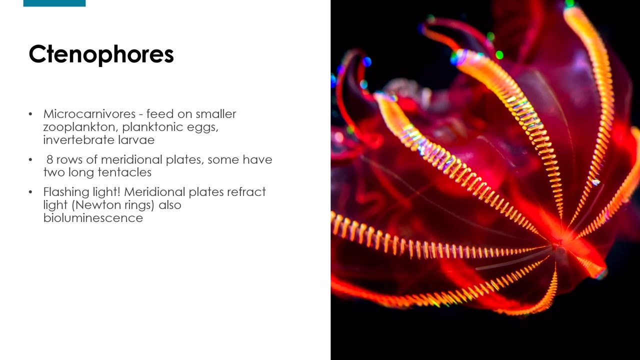 So ctenophores. they are boop microcarnivores. They like to feed on smaller zooplankton and planktonic eggs and invertebrate larvae. They have eight rows of meridional plates and some have two long tentacles. 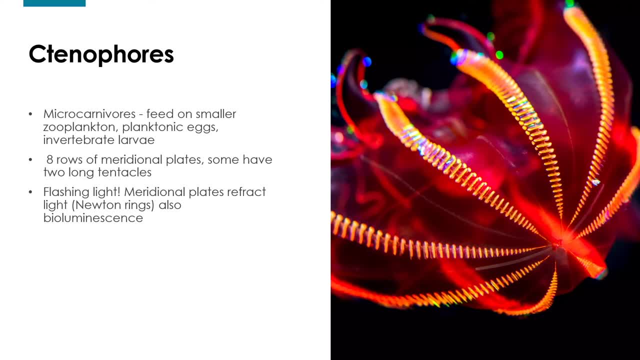 And so these comb rows are fused cilia that are arranged along the sides again of the ctenophore, And they're clearly visible, like we can see in the image on the right, And the cilia they beat together in unison. 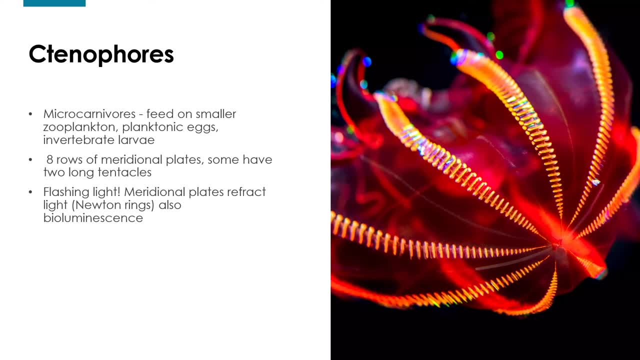 and it helps propel the ctenophore in the water. And some species of ctenophore will actually move with a flapping motion or like undulations of the body. And, yes, many ctenophores can have two long tentacles. 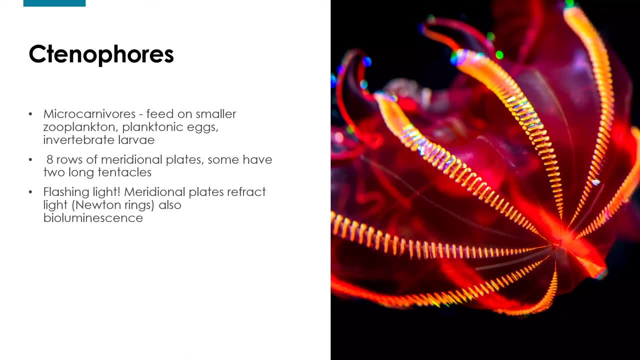 on their body, but some also just lack tentacles completely And, unlike cnidarians, which have stinging cells, or nematocysts, ctenophores do not. Instead, they possess sticky cells called coloblasts to catch and to hold onto their prey. 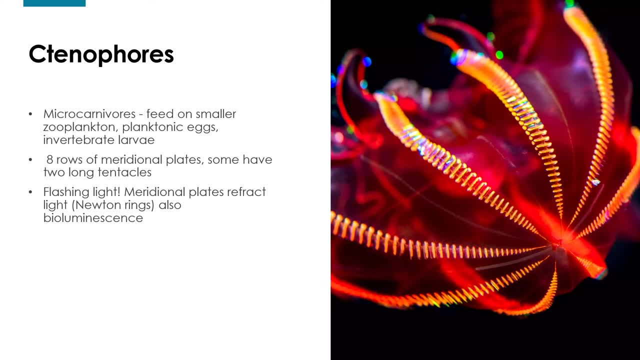 And one of the most interesting things about ctenophores is that they are able to produce this light scattering effect by beating the eight rows of cilia on their body, And when you see the cilia moving, it appears almost like a rainbow, a transition of color. 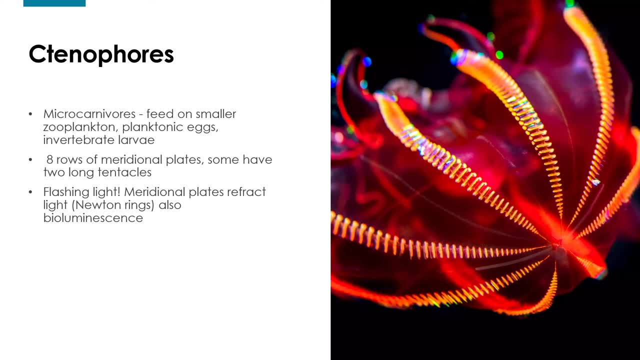 active in this area and they'll fight when the other Cnidophore gets in touch with the other Cnidophore that has already formed the secondary shell. So you'll see the Cnidophores moving, but they're still a variety of different species And so the origin of the Cnidophore. 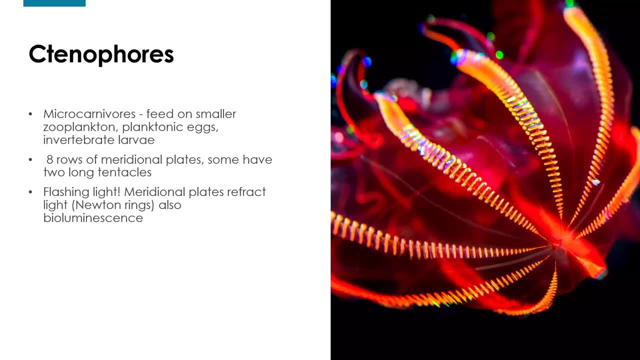 in this area is found in the native water, And so they're very, very, very active. They can be really active. they can be very invasive. So this is an example of the Cnidophore that I have in the water And some species of Cnidophores. 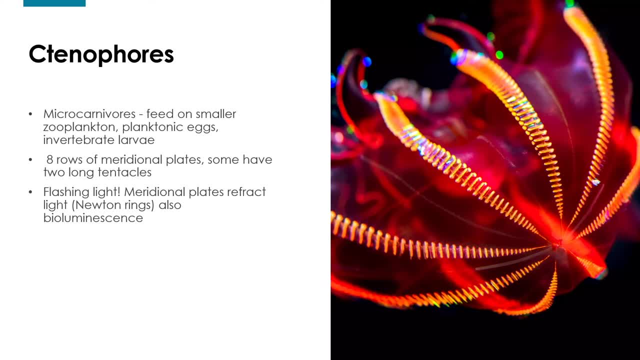 Tinnifors do not. Instead, they possess sticky cells called coloblasts to catch and to hold on to their prey. One of the most interesting things about tinnifors is that they are able to produce this light scattering effect by beating the eight rows of. 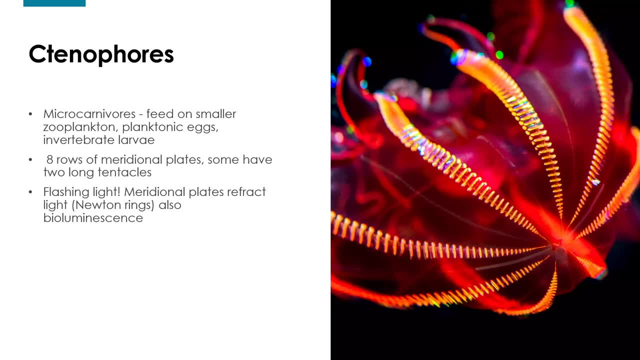 cilia on their body. When you see the cilia moving, it appears almost like a rainbow, a transition of color, and it's really beautiful. I'll show you in the next slide a video of this. Most people assume that with tinnifors, that bioluminescence is also the same. 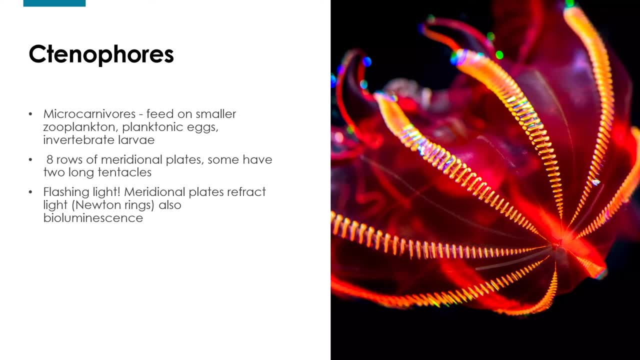 rainbow effect that you might see, but actually the colors that you will typically see will not be the same as the tinnifors that you might see when you see bioluminescence. The tinnifors that you see with bioluminescence would be: 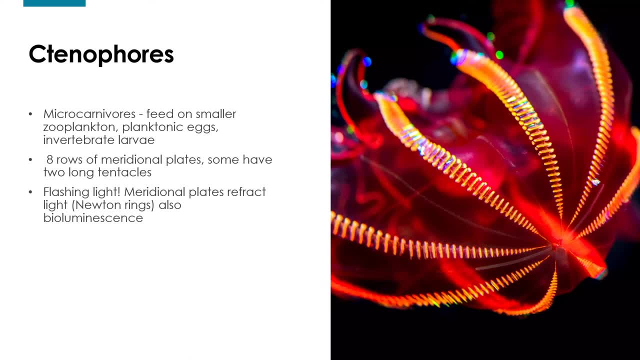 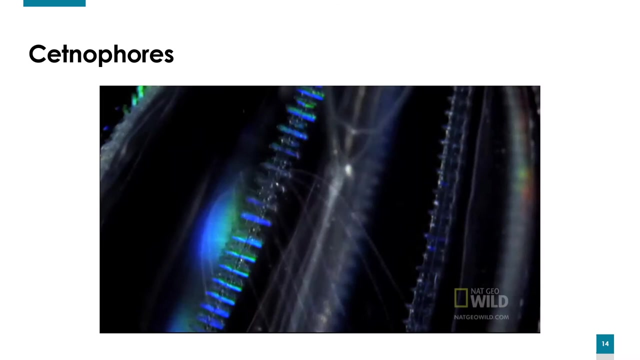 green and blue, and so not all tinnifors can produce bioluminescence. but when you do see bioluminescence occurring in tinnifors, it can only occur in pitch black or in darkness. In the next video I just want to show a good 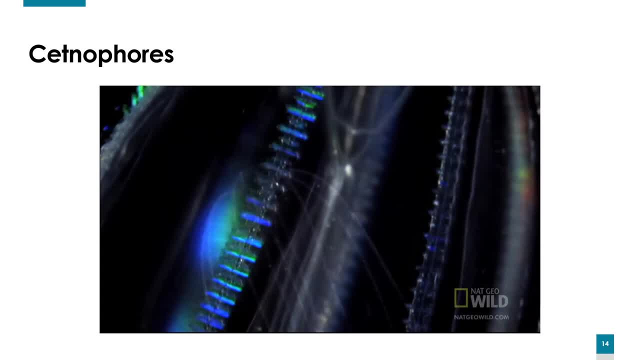 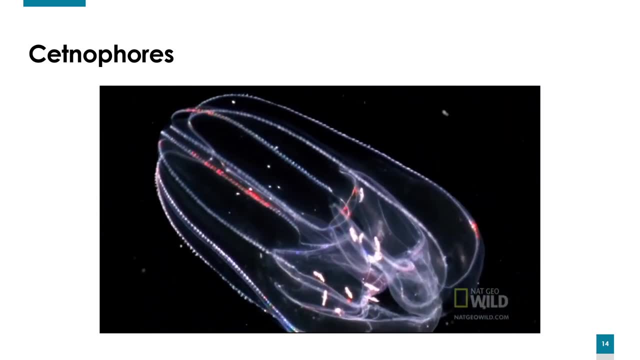 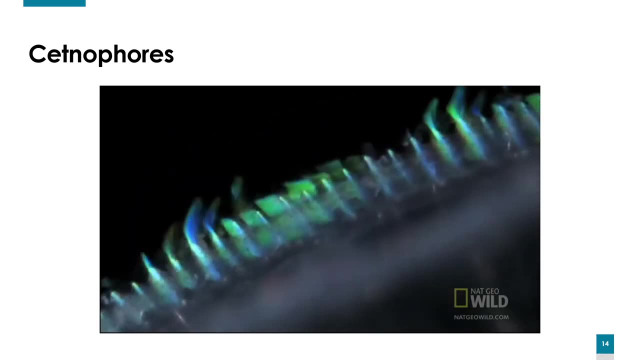 example of what the tinnifors can do. The tinnifors look like when they are beating the cilia, and you can see this rainbow color effect happening here. Yes, you can see it running all along down here on this one. Let me see if I can. ah, yes, there we go and you get a much. 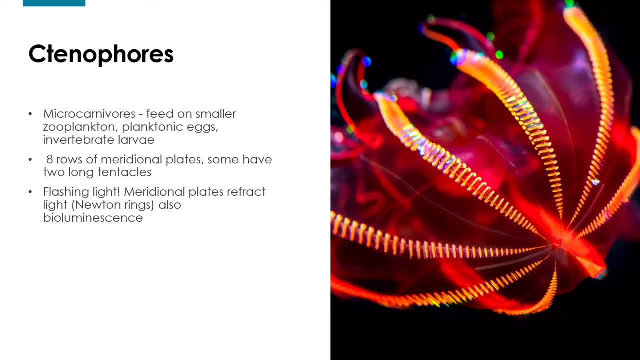 and it's really beautiful And I'll show you in the next slide of video of this. And most people assume that with ctenophores that bioluminescence is also the same rainbow effect that you might see, but actually the colors that you will typically see with bioluminescence. 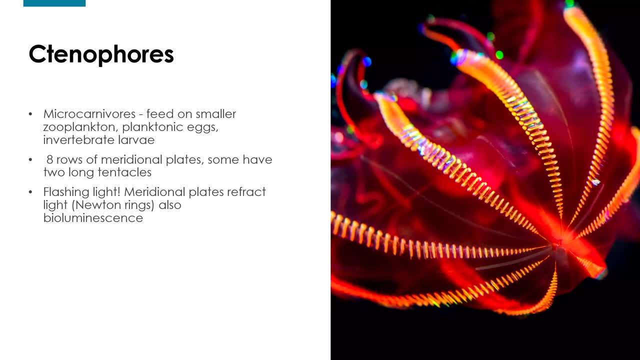 would be green and blue, And so not all ctenophores can produce bioluminescence. but when you do see bioluminescence, it's occurring. in ctenophores, It can only occur in pitch black or in darkness. 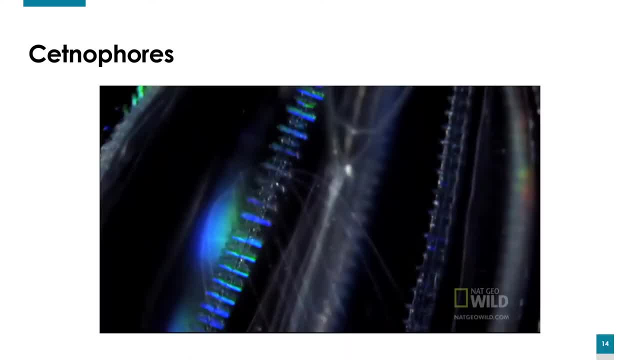 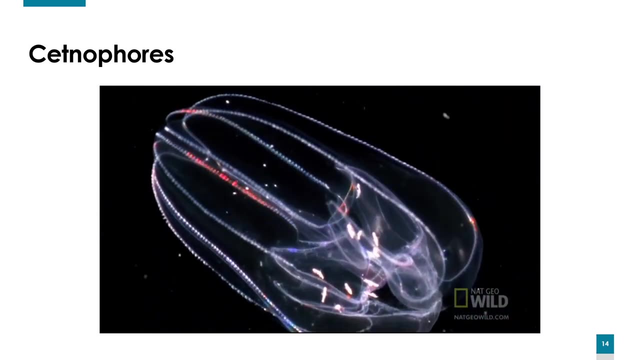 And so let's see in the next video. I just want to show a good example of what the ctenophores look like when they are beating the cilia, and you can see this rainbow color effect happening here. Yes, you can see it running all along down here on this gun. 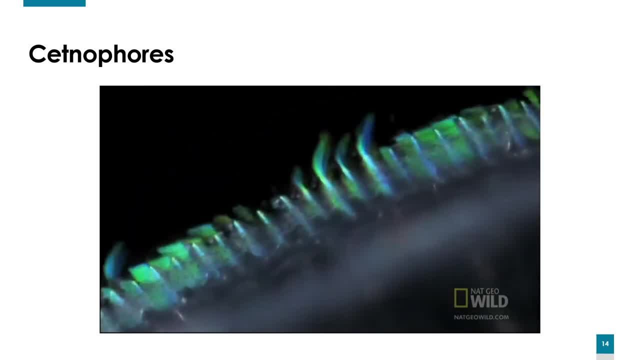 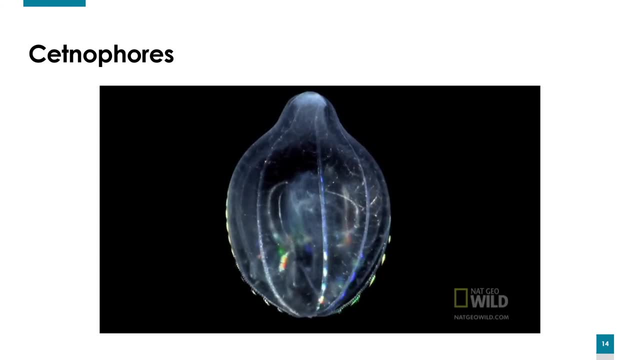 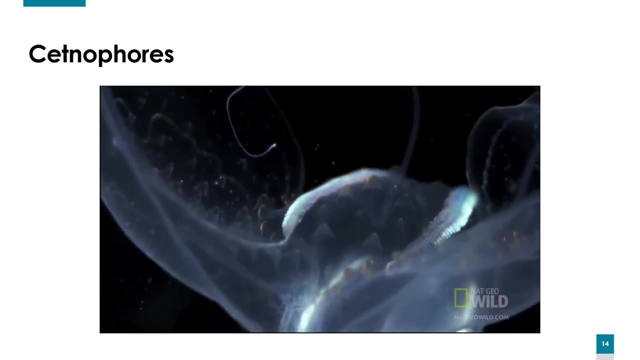 I'm going to see if I can. Ah, yes, there we go and you get a much better up-close. look on what that process looks like, And when you see these up close, they are moving so quickly and they look very beautiful in their environment. 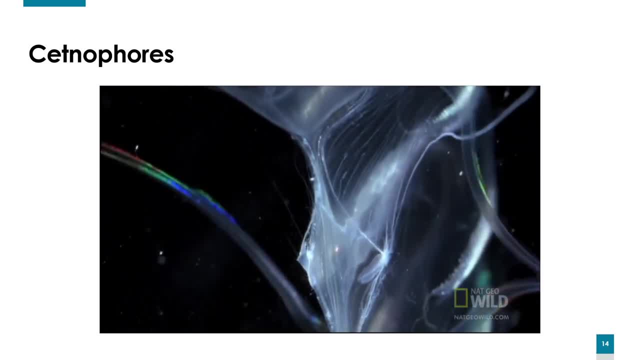 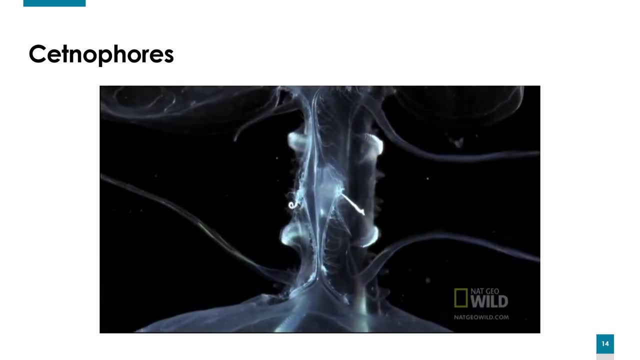 And in most aquariums, when they're trying to display ctenophores, they will try to display them in a darker tank or a tank that has less light, so that you really can see the different colors that are on the ctenophores. 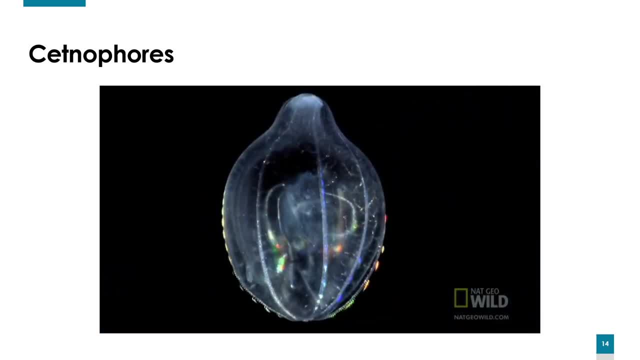 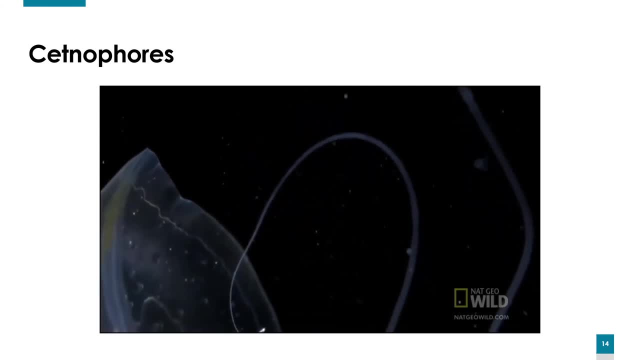 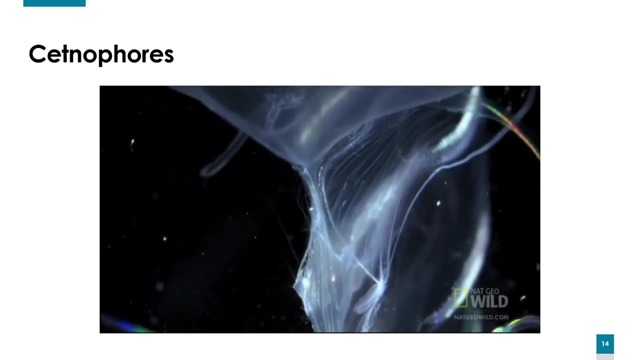 better up-close look on what that process looks like And when you see these up close, they are moving so quickly and they look very beautiful in their environment And in most aquariums. when they're trying to display tinnifors, they will try to. 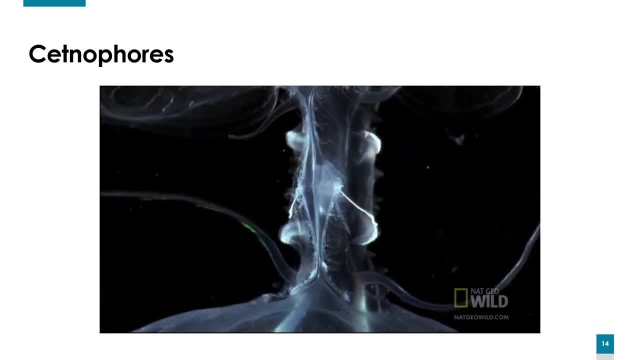 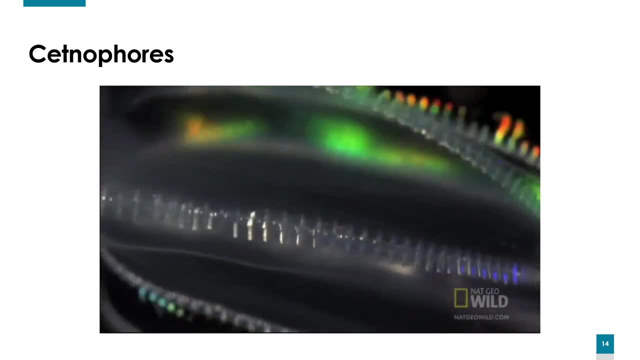 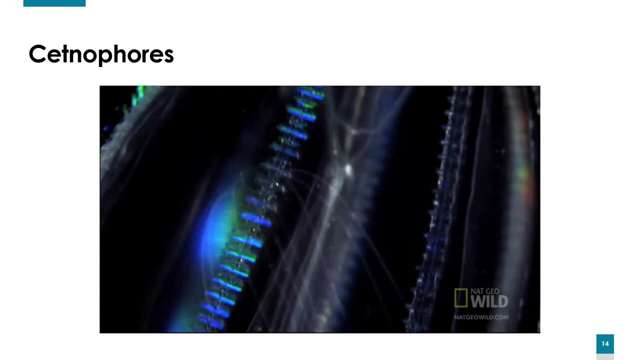 display them in a darker tank or a tank that has less light, so that you really can see the different colors that are on the tinnifors. So this is a nice video to showcase and highlight that. Thank you so much for watching and I'll see you in the next video. 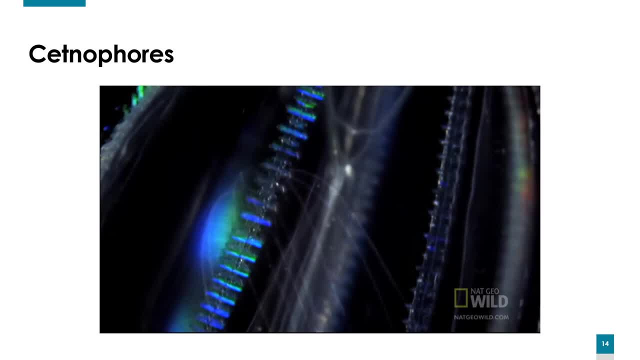 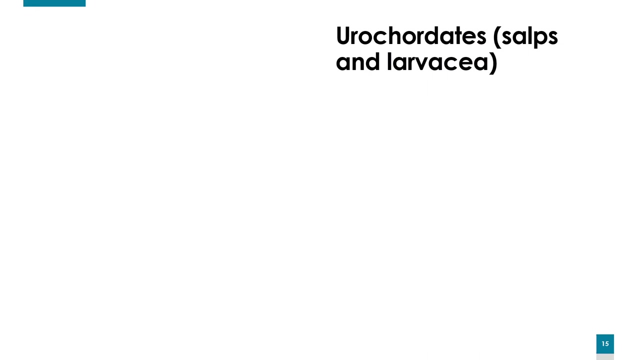 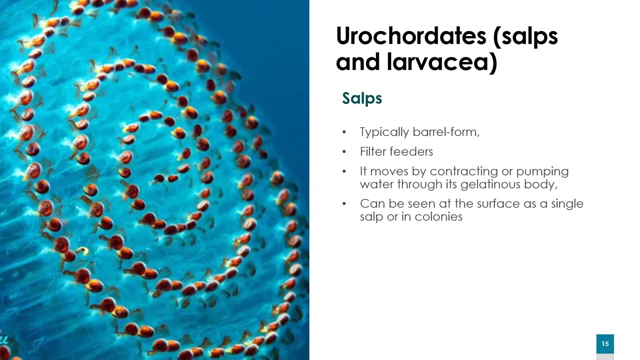 Subtitles by the Amaraorg community: community. Subtitles by the Amaraorg community. Alright, so up next we have Urochordates, which will include Salps and Lavraciae Click And so Salps: they're typically barrel-like in form and they are filter. 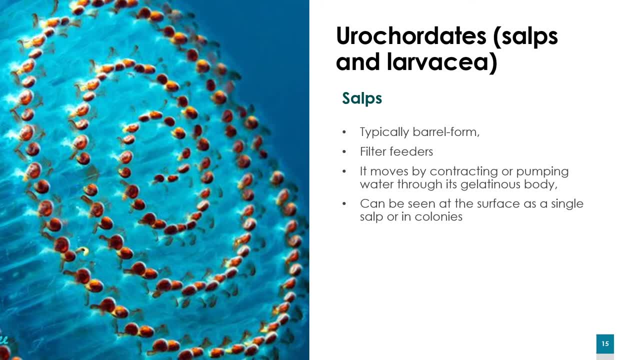 feeders, excuse me, and they move by contracting or pumping water through their body. so, in order to propel them through the water- And they can be seen typically at the surface as a single Salp, or you can see them in these massive, massive colonies- And so their 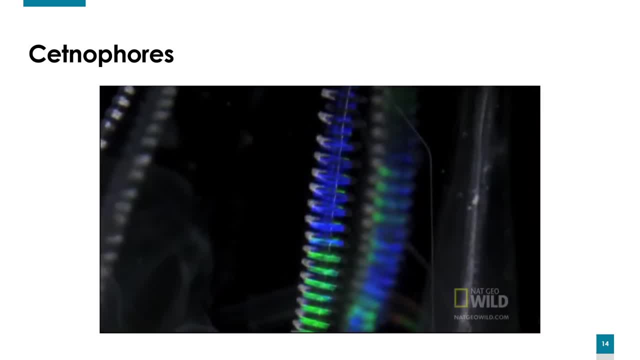 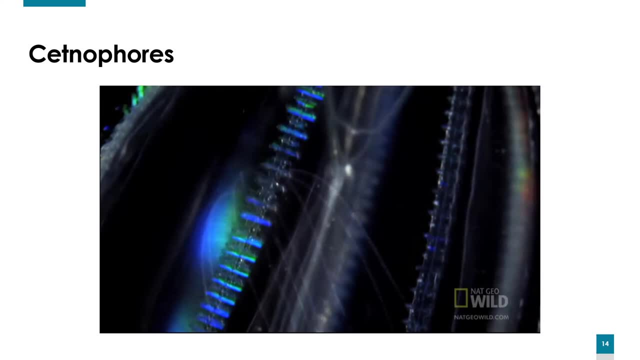 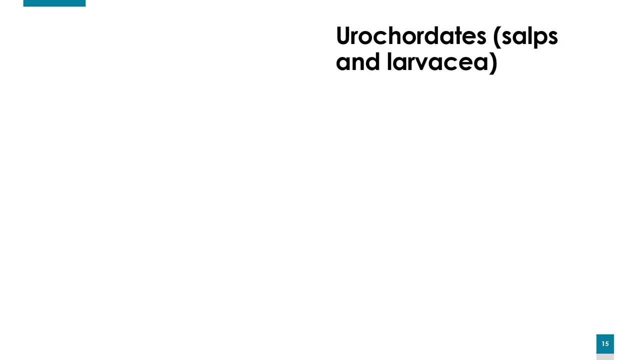 So this is a nice video to showcase and highlight that. Thank you for watching. See you next time. Bye. Subtitles by the Amaraorg community, wwwamaraorg. Okay, so up next we have Urochordates, which will include salps and Lavrasiae. 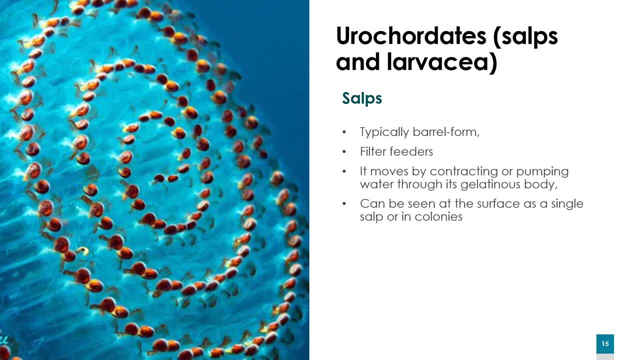 Click And so salps. they're typically barrel-like in form and they are filter feeders, excuse me, and they move by contracting or pumping water through their body. so in order to propel them through the water, And they can be seen, typically at the surface. 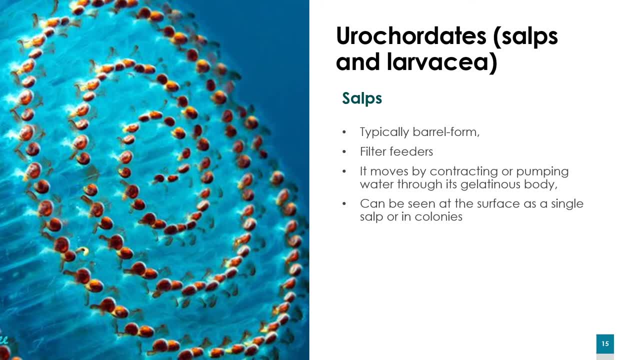 as a single salp, or you can see them in these massive, massive colonies, And so their most abundant concentrations of salps are typically found within the Southern Ocean, near Antarctica, And we've seen a lot of these salps of salps in our samples within the last couple of years. 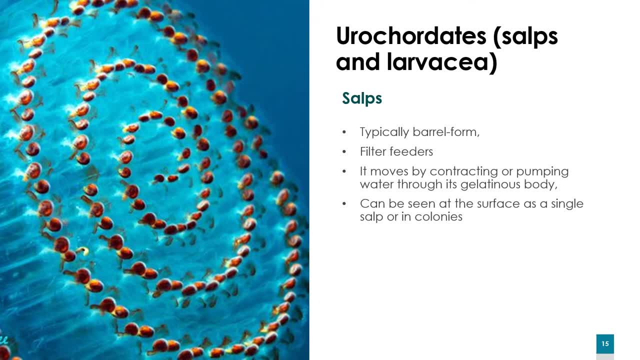 most abundant concentrations of Salps are typically found within the Southern Ocean, near Antarctica, And we've seen a lot of these Salps of Salps in our samples within the last couple of years, And this is noteworthy because typically we don't see Salps this far north. 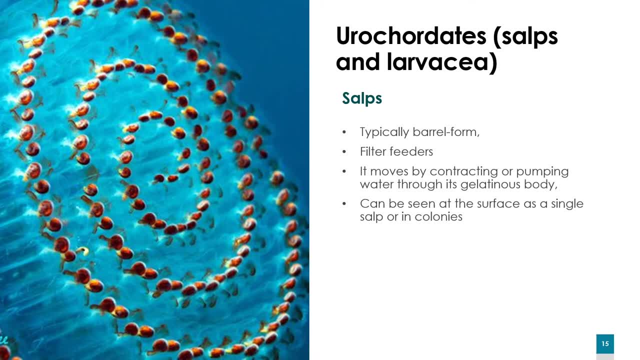 especially along in San Diego or near San Diego, And so there's been a lot of interest recently on why this is and how this will affect local zooplankton populations in the future. And so next we have Lavraciae, and so they are. 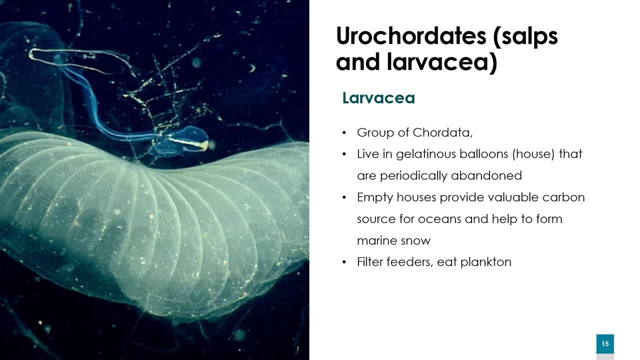 from the group Chordata, and they live in gelatinous balloons, or what we call houses, And the Lavraciae could also be called appendicularians, and they will periodically leave or abandon their house in order to feed, And so they are. 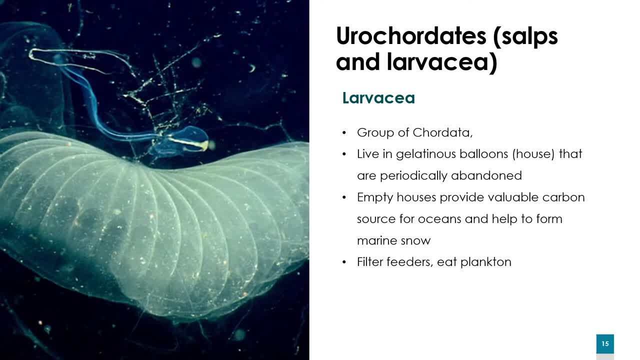 mostly transparent and they are filter feeders and they do eat other types of plankton or zooplankton, And so the house portion of the appendicularian, or Lavraciae, is characterized by two openings, and they're located on opposite ends of the structure of the 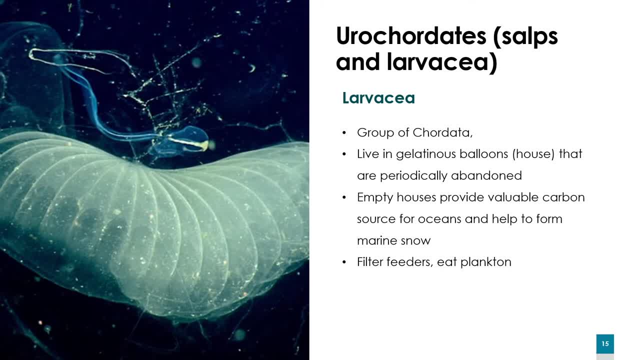 house and they enclose the trunk and the body, And so with the Lavracian they can propel the house forward through the water by beating it its tail, And by beating its tail it produces a current that pretty much pulls the water through and then forward, or through the opening of the house And then 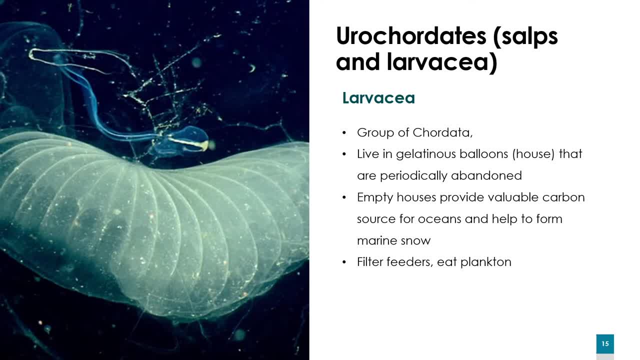 it pushes the water back out through the back end of the house, And so what this does is it allows for the microscopic food particles to pass through and become captured, And then it allows for carbonation and photosynthesis and so forth through the alive now чтоб becoming captured, And then en这是. 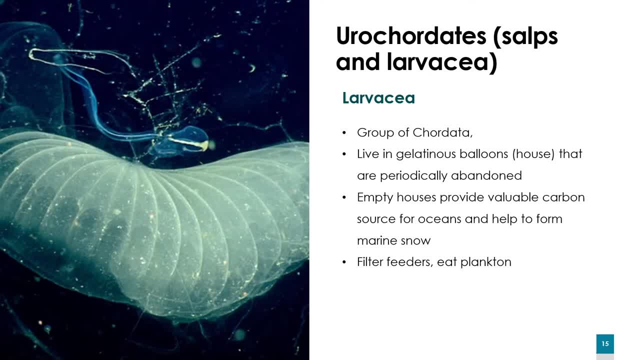 It black Люان. 우리 elders luy ole remarkettenskt. i vraag of owna leny, 你怎会 for the Lavarcian to eat and then move on? And basically, what happens is that these organisms will consistently create and abandon houses. 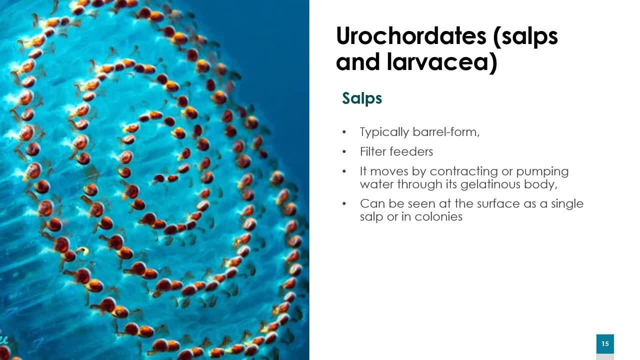 And this is noteworthy because typically we don't see salps this far north, especially along in San Diego or near San Diego, And so there's been a lot of interest recently on why this is and how this will affect local zooplankton populations. 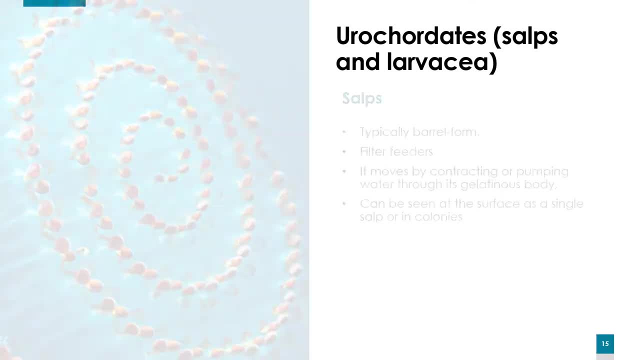 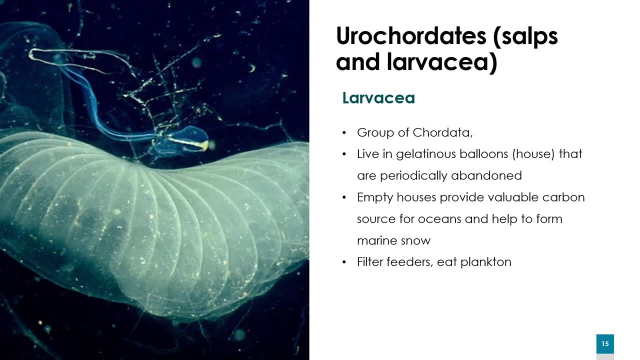 in the future. And so next we have Lavrasiae, And so they are from the group Chordata and they live in gelatinous balloons, or what we call houses, And the Lavrasiae could also be called appendicularians. 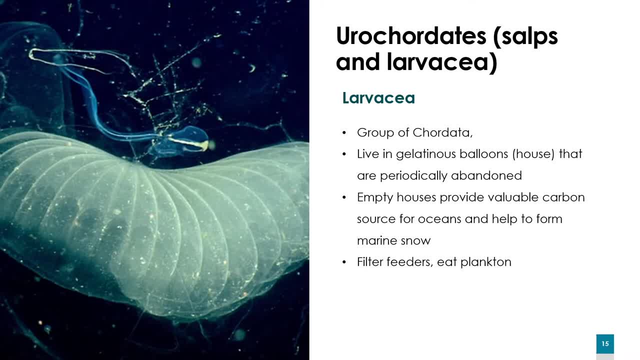 and they will periodically leave or abandon their house in order to feed, And so they are mostly transparent and they are filter feeders and they do eat other types of plankton or zooplankton, And so the house portion of the appendicular. 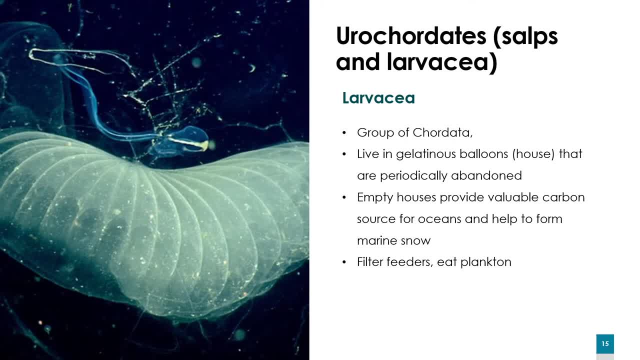 like appendicularian, excuse me, or Lavrasiae is characterized by two openings and they're located on the opposite ends of the structure of the house and they enclose the trunk and the body, And so, with the Lavrasiae, 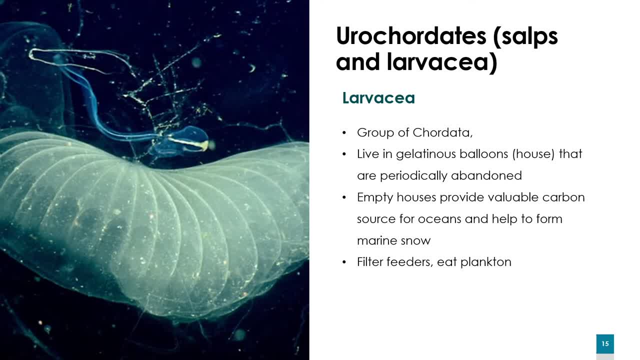 they can propel the house forward through the water by beating its tail. And by beating its tail it produces a current that pretty much pulls the water through and then forward, or through the opening- excuse me- of the house, And then it pushes the water back out. 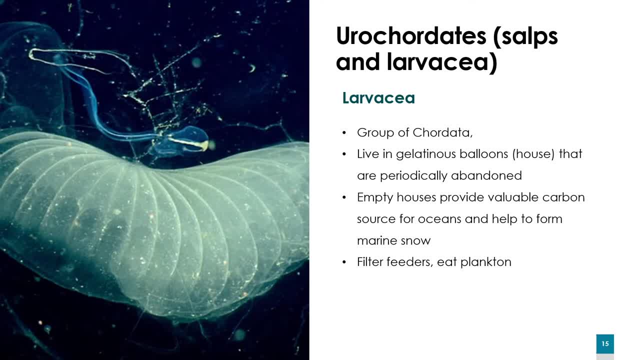 through the back end of the house, And so what this does is it allows for the microscopic food particles to pass through and become captured, and then it allows for the Lavrasiae to eat and and then move on, And basically what happens is that 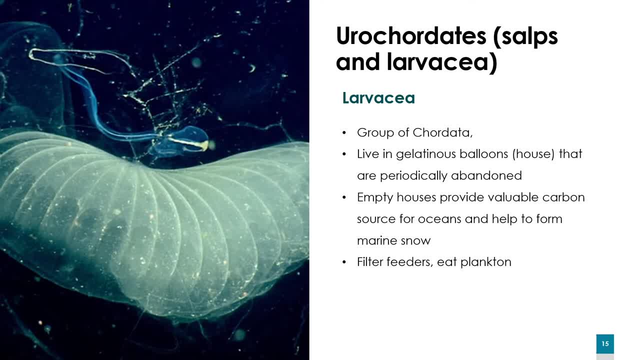 these organisms will consistently create and abandon houses several times each day, And this is important because these empty houses provide valuable carbon source for oceans and to help produce marine snow that other types of zooplankton at lower depths in the in the water column feed on. 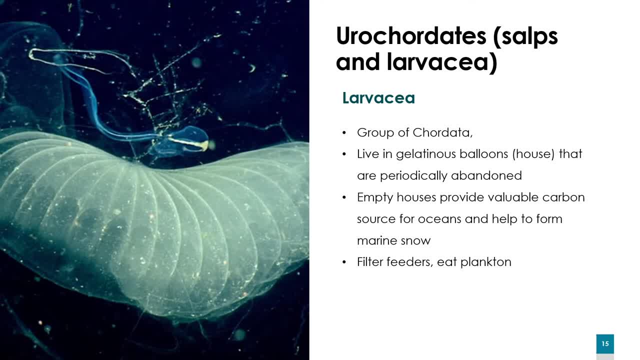 several times each day, And this is important because these empty houses provide valuable carbon source for oceans and to help produce marine snow that other types of zooplankton at lower depths in the water column feed on for their source of food and nutrition. So these Lavarcians are pretty cool. 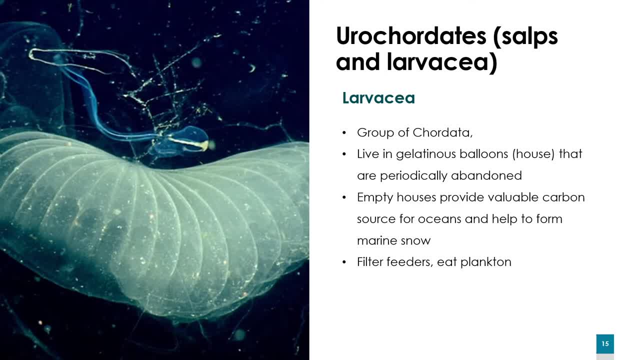 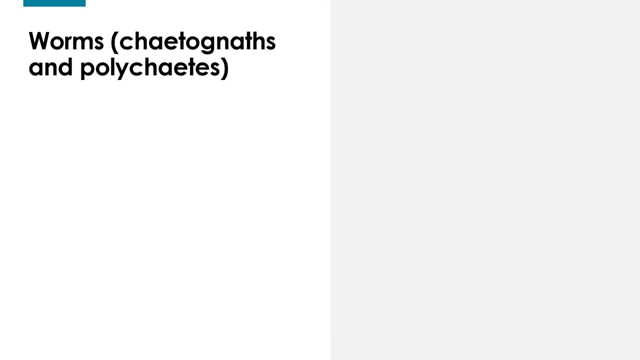 and not much footage is recorded on their feeding behavior. So it's always really neat, when we do have that footage, to observe how they react in their natural environment. For this next slide, we're gonna be talking about worms, which will include chitignaths. 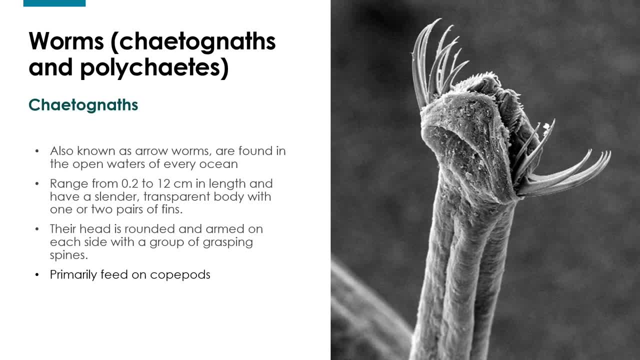 and polychaetes, And so with chitignaths. this image, by the way, is so cool. They are also known as arrow worms, and they can be found in open waters of pretty much every ocean, And they range from around 0.2 to 12 centimeters in length. 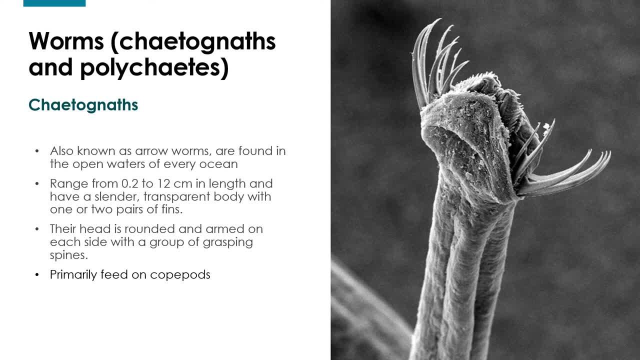 and they have a slender, transparent body with one or two pairs of fins, And so their head is rounded, as you can see in this picture, and armed with, on each side, a group of grasping spines, And they use these spines to hunt, primarily on copepods. 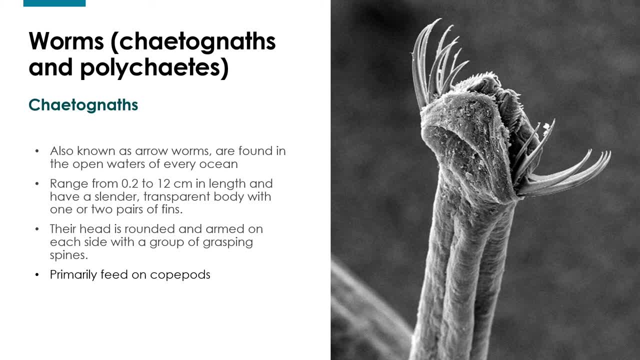 And so they rely on the tufts of these tiny hairs- and you can kind of see it in this picture here on their head- to recognize the vibrations produced by their prey. And so what the chitignaths will do is they'll use the hairs and actually snatch up the prey. 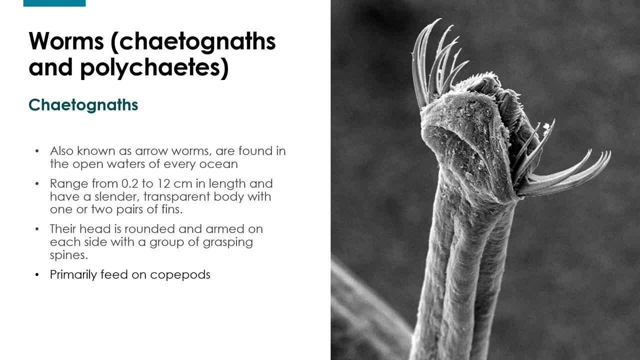 And they, like I said, primarily feed on copepods, but they will also eat amphipods and ostracods and other types of worms like polychaetes and other types of planktonic tunicates as well, And sometimes too fish larvae. 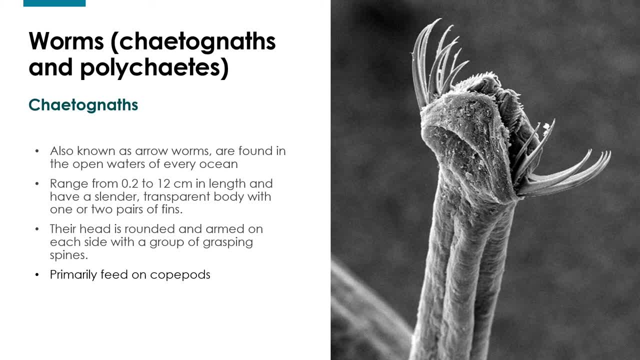 And what's really cool about this image is that you can see their teeth, and they use their teeth to also capture their prey. And what's really interesting about chitignaths- excuse me- is that even when I have seen these in my samples- 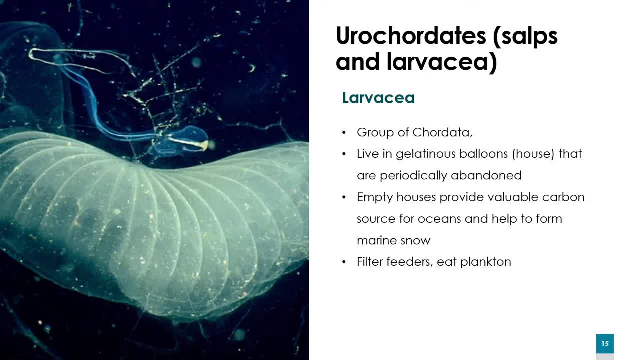 their source of food and nutrition. So these Lavrasiae are pretty cool and not much footage is recorded on their feeding behavior, So it's always really neat- when we do have that footage, to observe how they react in their natural environment. For this next slide. 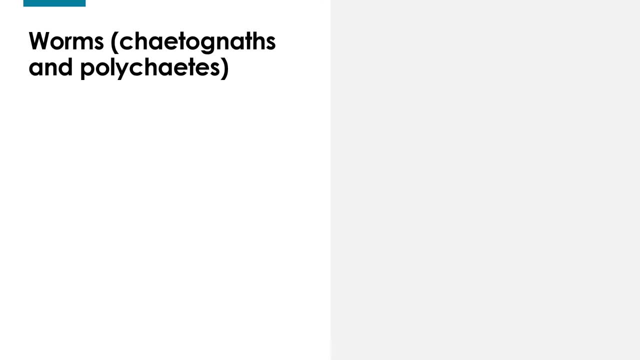 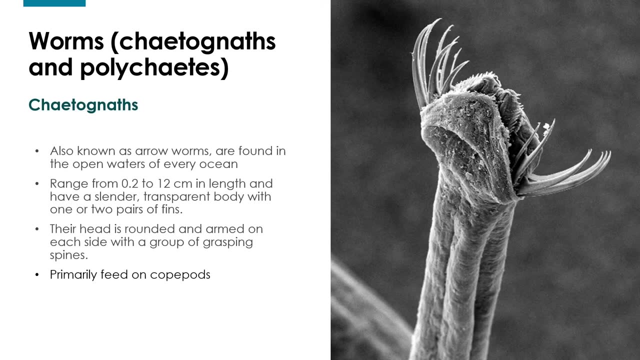 we're going to be talking about worms, which will include chetignaths and polychaetes, And so with chetignaths- this image, by the way, is so cool- They are also known as arrow worms, and they can be found in open waters. 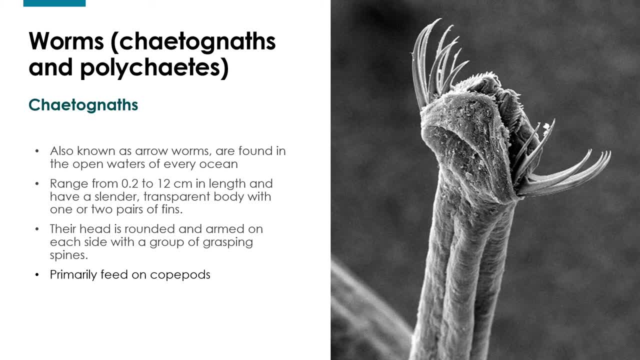 of pretty much every ocean, And they range from around 0.2 to 12 centimeters in length, and they have a slender, transparent body with one or two pairs of fins, And so their head is rounded, as you can see in this picture. 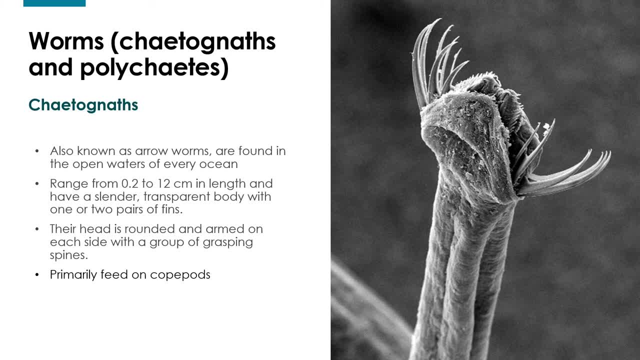 and armed with on each side a group of grasping spines, And they use these spines to hunt, primarily on copepods, And so they rely on the tufts of these tiny hairs, and you can kind of see it in this picture here. 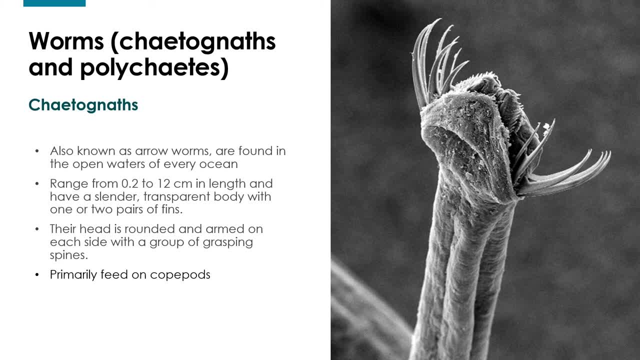 on their head to recognize the vibrations produced by their prey, And so what the chetignaths will do is they'll use the hairs and actually snatch up the prey, And they, like I said, primarily feed on copepods, but they will also eat amphipods. 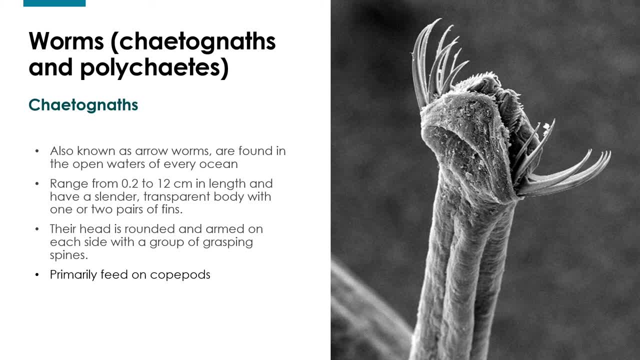 and ostracods and other types of worms like polychaetes and other types of planktonic tunicates as well, and sometimes too fish larvae, And what's really cool about this image is that you can see their teeth. 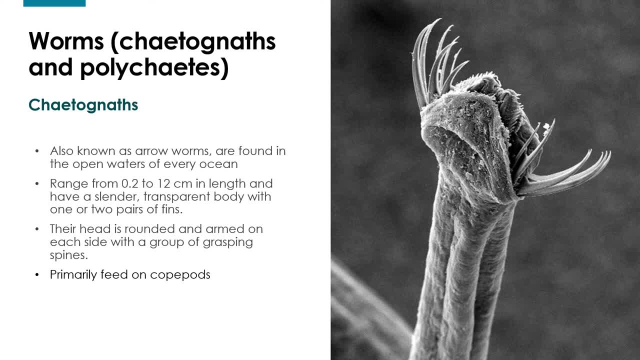 and they use their teeth to also capture their prey. And what's really interesting about chetignaths, excuse me, is that even when I have seen these in my samples, you can so easily see the head and the spines and the jaw pretty much. 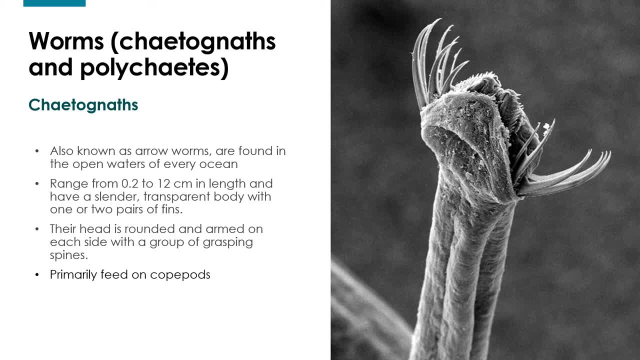 of these chetignaths and they truly look like carnivorous zooplankton, and they're ready to eat other types of zooplankton. And then the next types of worm again are polychaetes, and these guys are segmented worms. 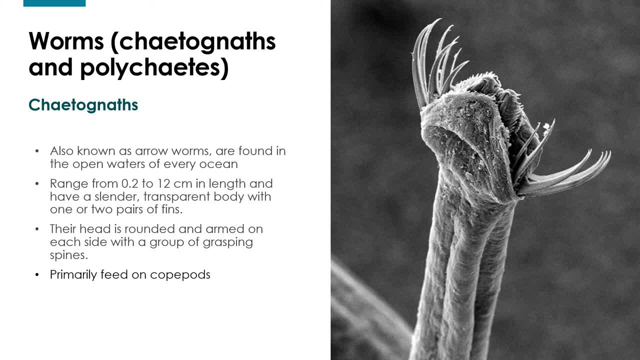 you can so easily see the head and the spines and the jaw, pretty much of these chitignaths And they truly look like carnivorous zooplankton And they're ready to eat other types of zooplankton. 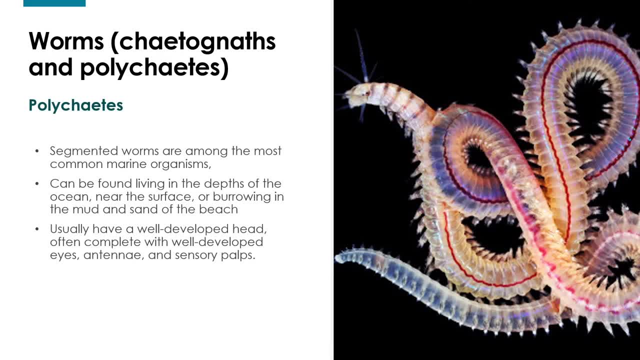 And then the next types of worm again are polychaetes, And they're ready to eat other types of zooplankton. And then the next types of worm again are polychaetes, And these guys are segmented worms. 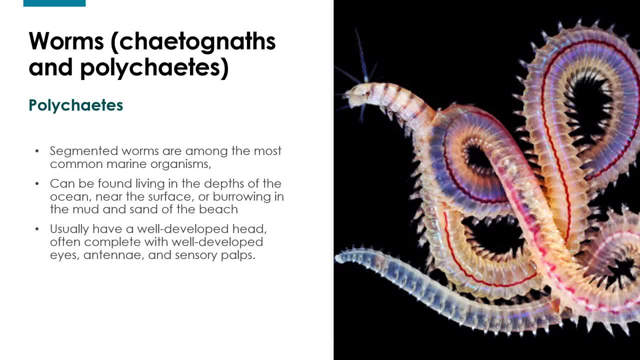 and they're among the most common marine organisms that we can find out there, And they can be found living in depths of the ocean or you can find them near the surface, And a lot of the time if you went tide pooling or out on the mud flats. 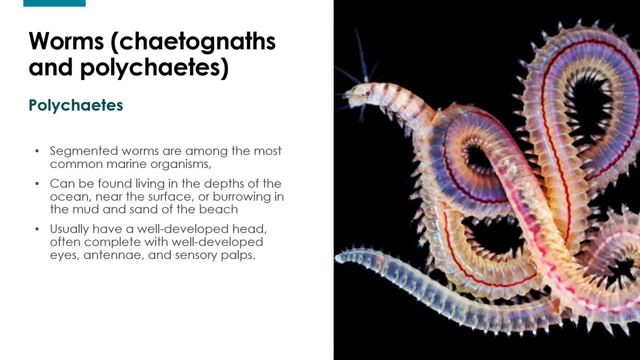 you would see them burying their bodies into the sand or mud at the beach And they usually have a well-developed head and often are complete with well-developed eyes, antennae and sensory palsy, Because a lot of the times, 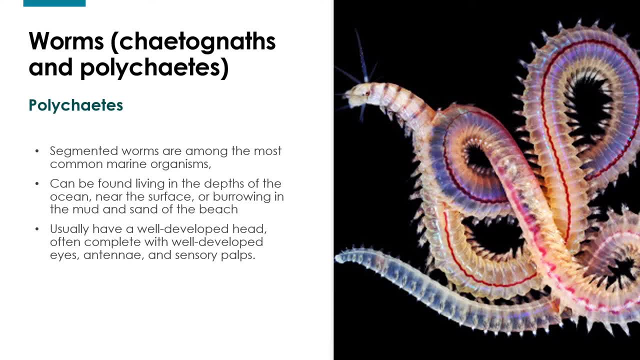 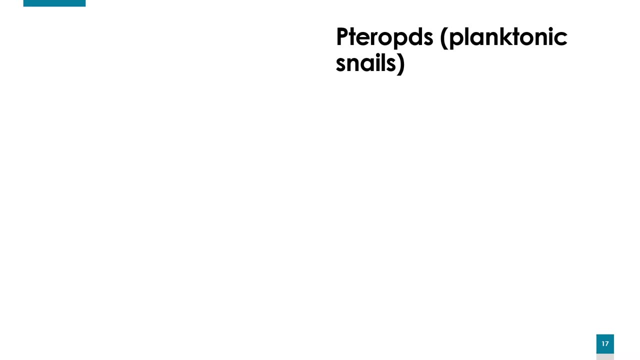 these polychaetes can be out of the water as well, So they need to have more developed organs and sensory or sensory organs to be able to detect light and oxygen when they're out of the water. All right, so pteropods are planktonic snails. 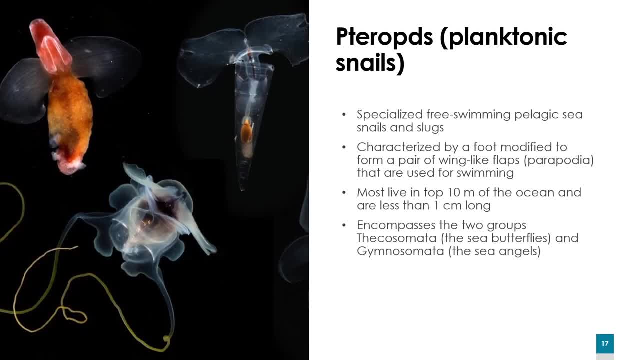 They are specialized free-swimming pelagic sea snails and slugs, And they're characterized by a foot that has been modified to form a pair of wing-like flaps, or parapodia, that allow them to actually swim within the water column, And they can actually be quite graceful. 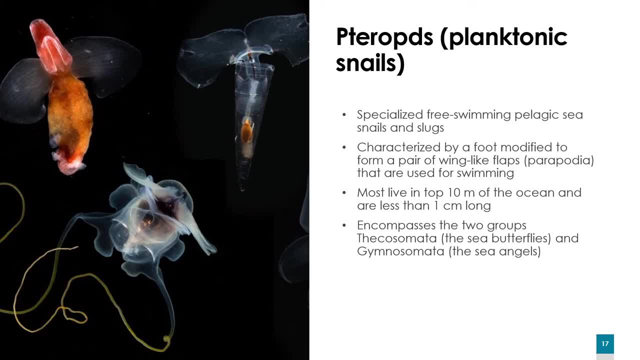 when we find them out in the ocean, And most live in the top 10 meters of the ocean, and they're pretty small, So they're less than about a centimeter in length. And pteropods include two different groups. Thecosomata are the sea butterflies. 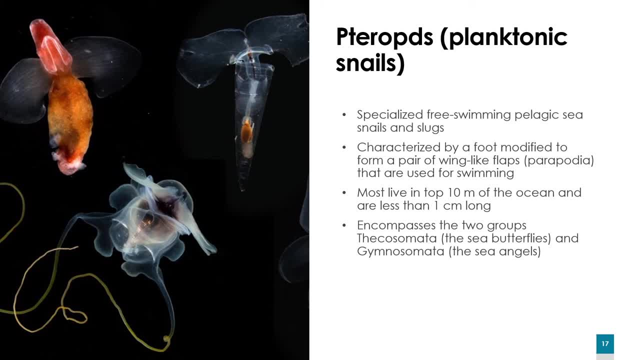 Or not sure if I'm pronouncing this right- gymnosomata, the sea angels, And thecosomata, the sea butterflies. they produce a net of sticky mucus to passively collect and eat marine snow, And so this is a great method to maximize amount of energy. 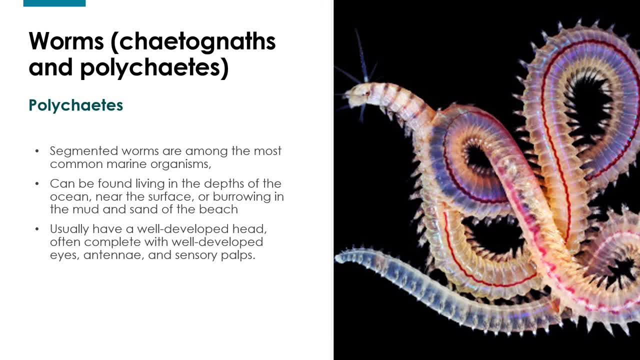 and they're among the most common organisms that we can find out there, and they can be found living in depths of the ocean or you can find them near the surface, and a lot of the time if you went tide pooling or out on the mudflats. 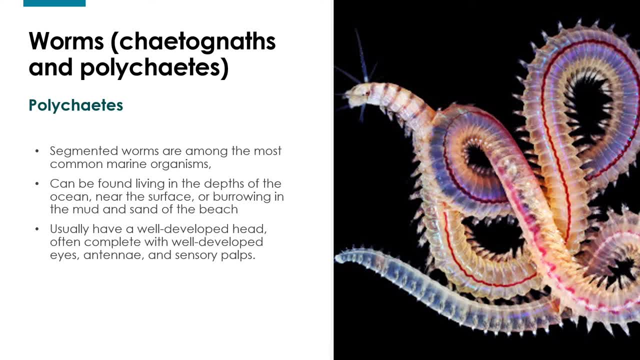 you would see them burying their bodies into the sand or mud at the beach And they usually have a well-developed head and often are complete with well-developed eyes, antennae and sensory palps, because a lot of the times, these polychaetes. 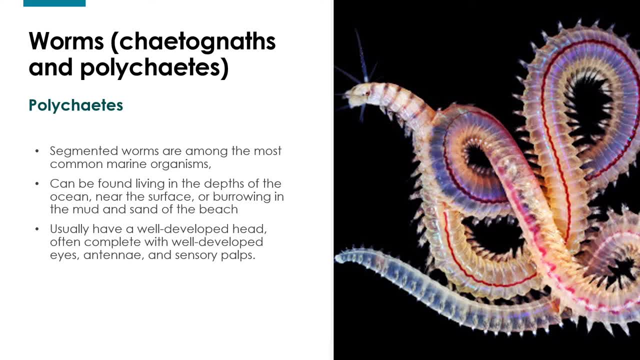 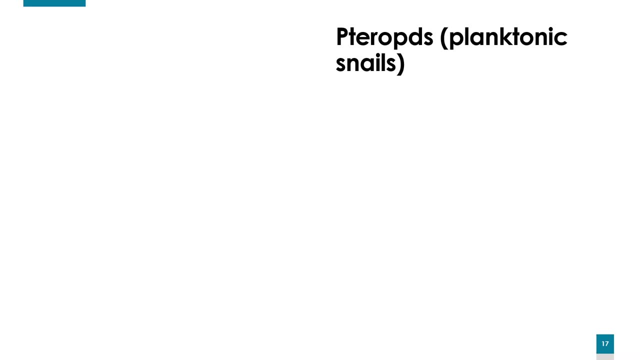 can be out of the water as well, so they need to have more developed organs or sensory organs to be able to detect light and oxygen when they're out of the water. Alright, so pteropods or planktonic snails. 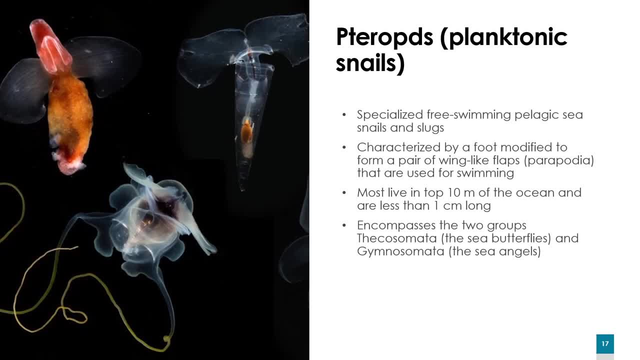 they are specialized free-swimming pelagic sea snails and slugs, and they are characterized by a foot that has been modified to form a pair of wing-like flaps, or parapodia, that allow them to actually swim within the water column. 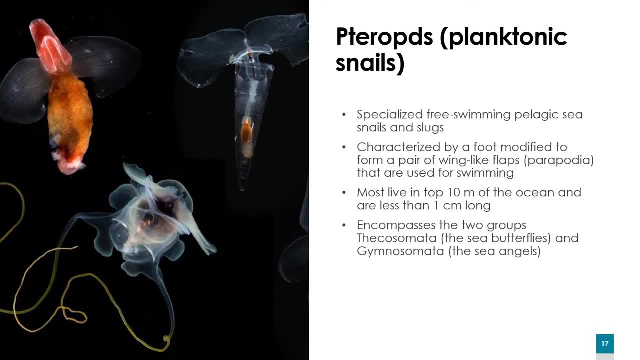 and they can actually be quite graceful when we find them out in the ocean, and most live in the top ten meters of the ocean and they're pretty small, so they're less than about a centimeter in length, and pteropods include. 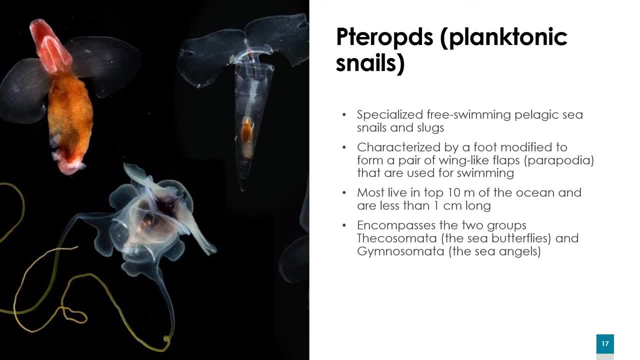 two different groups: Thicosomata or the sea butterflies, or not sure if I'm pronouncing this right- gymnosomata, the sea angels, and thicosomata, the sea butterflies. they produce a net of sticky mucus. 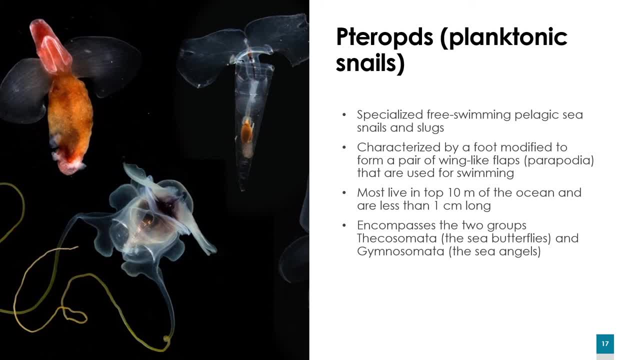 to passively collect and eat marine snow, and so this is a great method to maximize the amount of energy that you're using by creating just like a big net to do the work for you, versus trying to actively go out and hunt, whereas with gymnosomata. 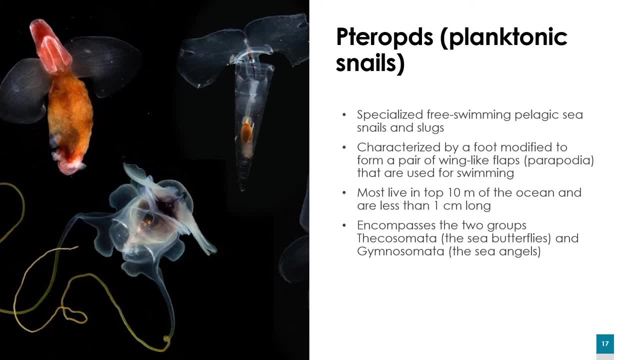 they do the opposite and they are active predators and they will go out and snatch up prey using these appendages that look like almost like a jaw of some sort, and they will pull the prey into their mouth to feed. And so two different types of pteropods. 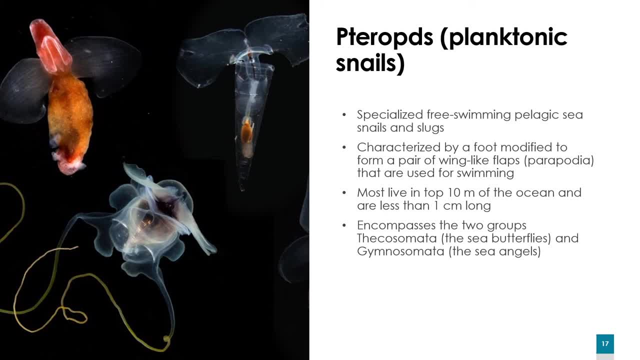 And this is a great way to stimulate your facet. Thank you, Okay, amount of energy that you're using by creating just like a big net to do the work for you, versus trying to actively go out and hunt, whereas with gymnosomata they do the opposite and they are. 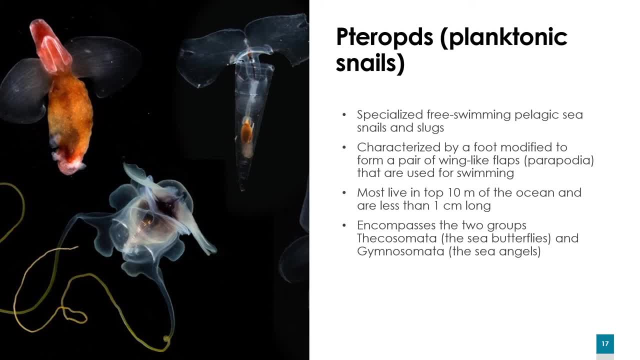 active predators and they will go out and snatch up prey um using these um appendages that look like almost like a jaw of some sort, and they will pull the prey into their mouth to feed. and so two different types of um pteropods and two very different methods for finding their food. 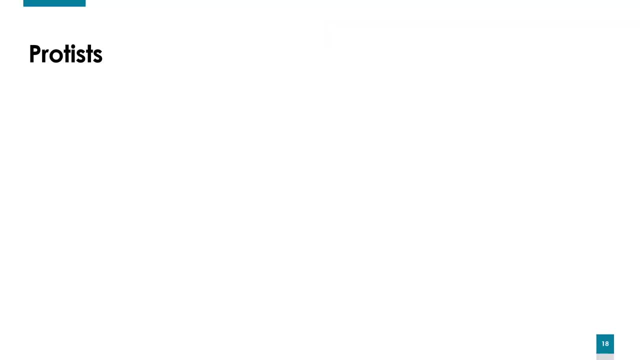 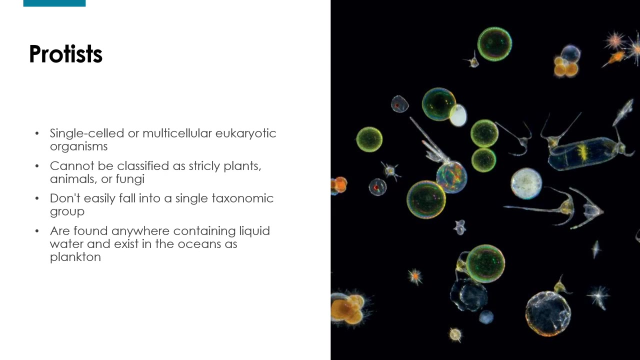 all right. so last of the taxonomic groups that we're going to cover today are protists, and with protists they are not easily categorized, and so they're single-celled or multicellular eukaryotic organisms and, again, like i said, they can't be classified strictly as either a plant or an animal or a fungi. so 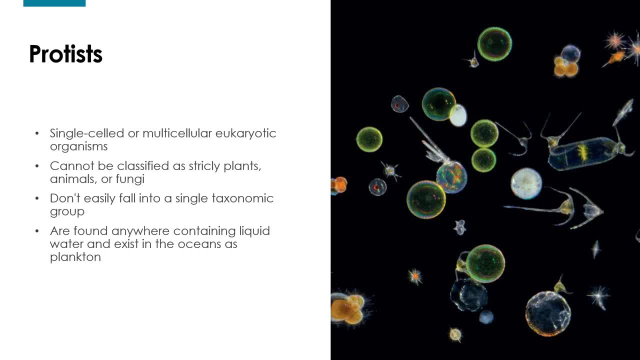 they don't easily fall into a single taxonomic group for that reason, and they can be found anywhere containing liquid water, so oceans or some fresh water bodies as well, and in the oceans they exist as types of plankton, and so what we're going to cover with protists today is talk about three. 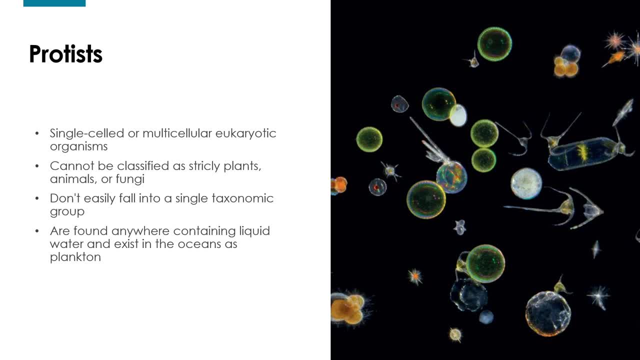 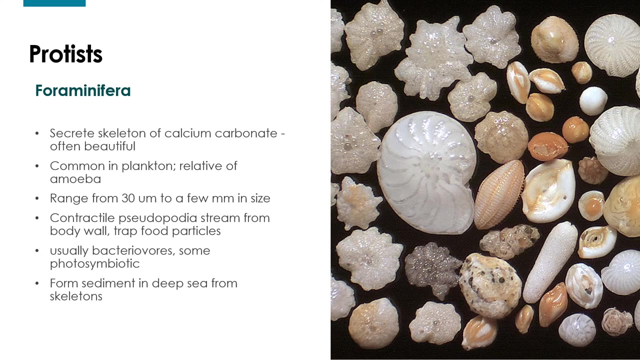 phylums, in particular within protista, that are animal-like, and then that they're heterotrophic and get their food by consuming other types of organisms, and so the first one is forams, or foraminifera, and so they secrete a skeleton of calcium carbonate, and their designs can be quite 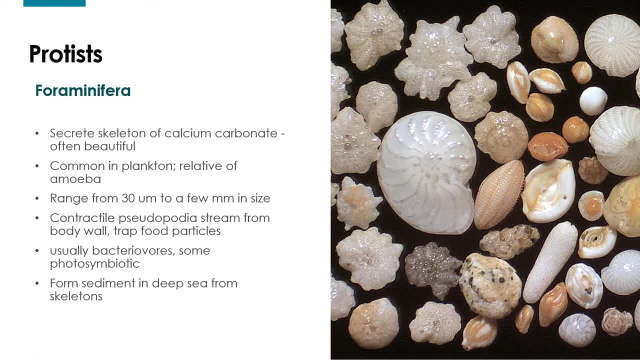 beautiful and symmetrical and they're common in a, a common type of plankton- excuse me- and relative of the amoeba, and they can range from 30 micrometers to a few millimeters in size. so you could, you can see some of them with the naked eye and they have contractile pseudopodia. 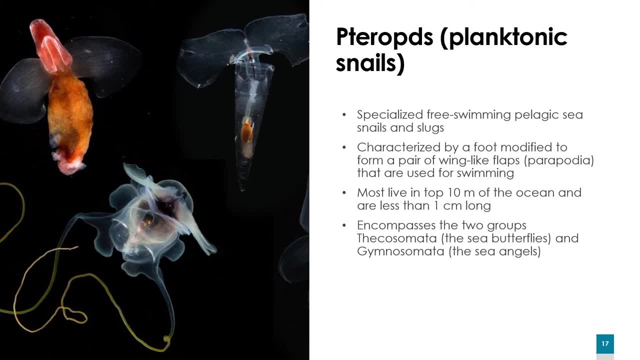 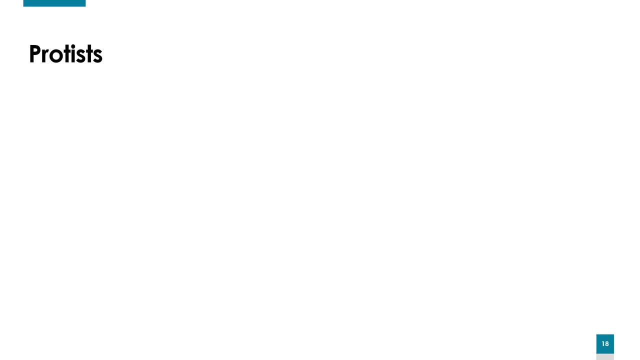 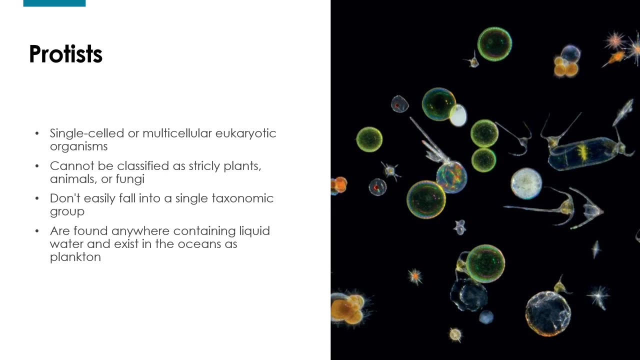 and two very different methods for finding their food. All right, so last of the taxonomic groups that we're going to cover today are protists, and with protists, they are not easily categorized, and so they're single-celled or multicellular eukaryotic organisms. 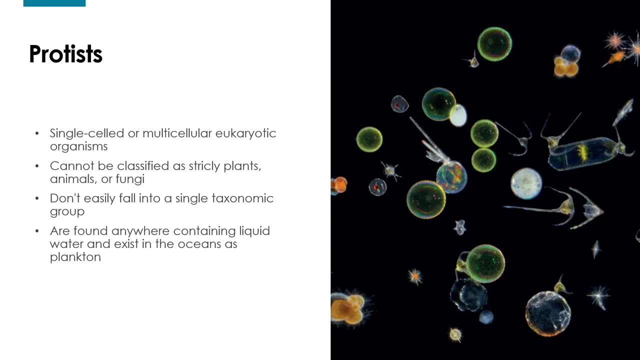 and again, like I said, they can't be classified strictly as either a plant or an animal or a fungi, so they don't easily fall into a single taxonomic group for that reason. and they can be found anywhere containing liquid water, so oceans. 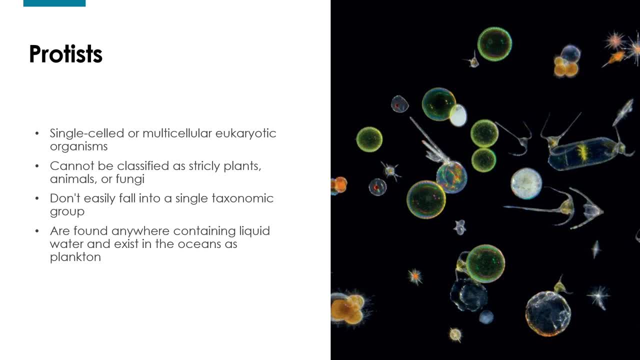 or some freshwater bodies as well, and in the oceans they exist as types of plankton, And so what we're going to cover with protists today is talk about three phylums, in particular within protista, that are animal-like, and then that they're heterotrophic. 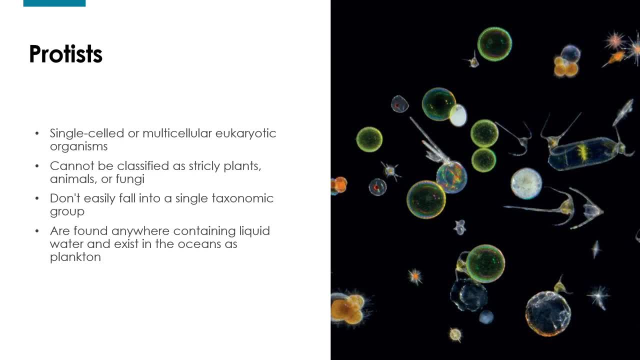 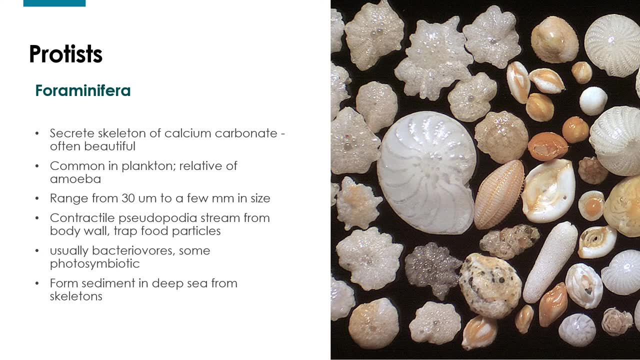 and get their food by consuming other types of organisms, And so the first one is forams, or foraminifera, and so they secrete a skeleton of calcium carbonate, and their designs can be quite beautiful and symmetrical. They're common in 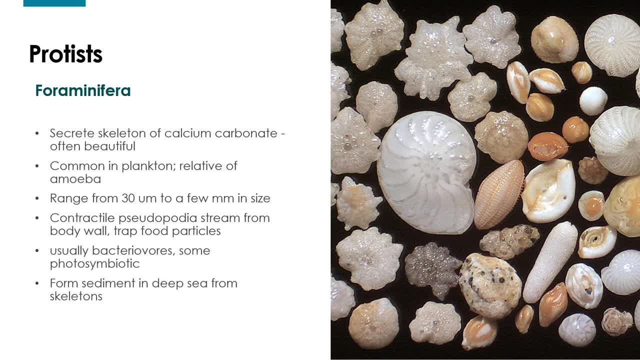 a common type of plankton, excuse me, and a relative of the amoeba, and they can range from 30 micrometers to a few millimeters in size, so you can see some of them with the naked eye, And they have contractile pseudopodia. 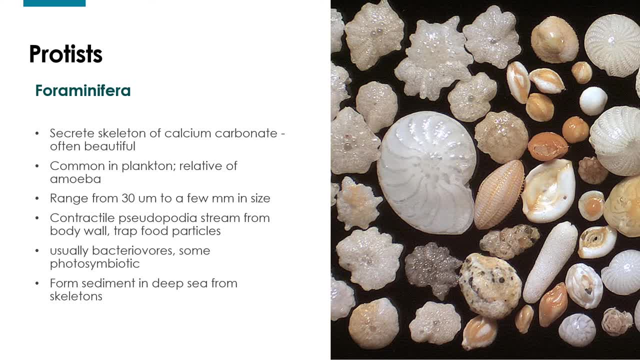 that stream from their body wall and that helps them to trap food particles, And so they're usually bacterivores, or sometimes they could be photosymbiotic, and so this is just another way that they're able to sustain themselves, And then they are able to form deep into the sediment. 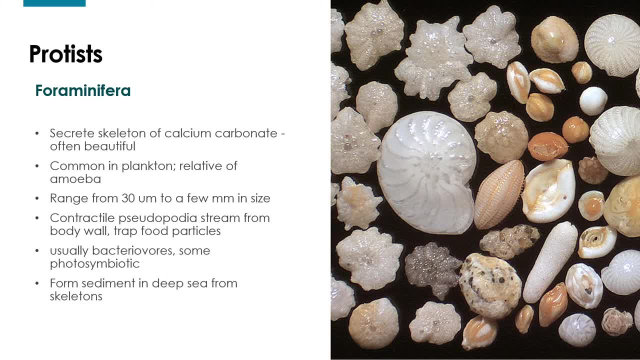 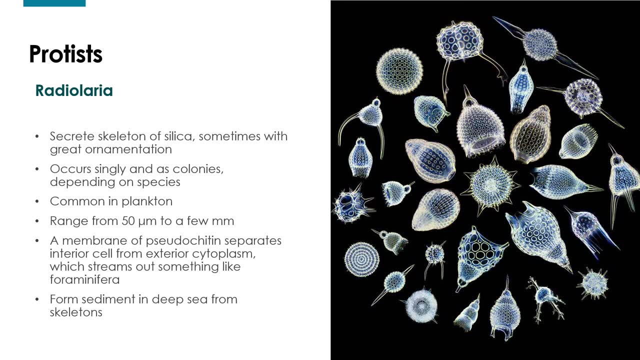 typically along the sea floor. And then next we have radiolaria, and these two also secrete a skeleton, but this one made out of silica, and sometimes the designs can be quite ornate, as you can see in this image here. 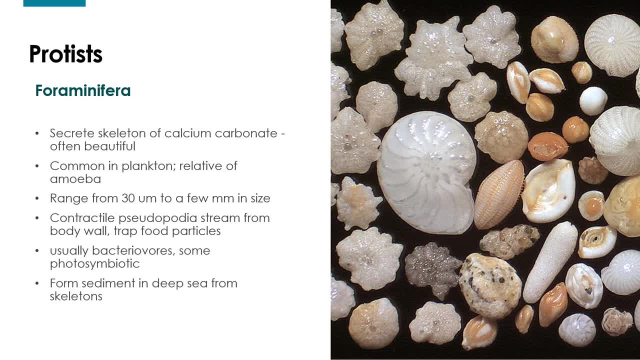 that stream from their body wall and that helps them to trap food particles, and so they're usually usually bacterial, or sometimes they could be photo-symbiotic, and so, um, this is just another way that they're able to sustain themselves, and then they are able to form. 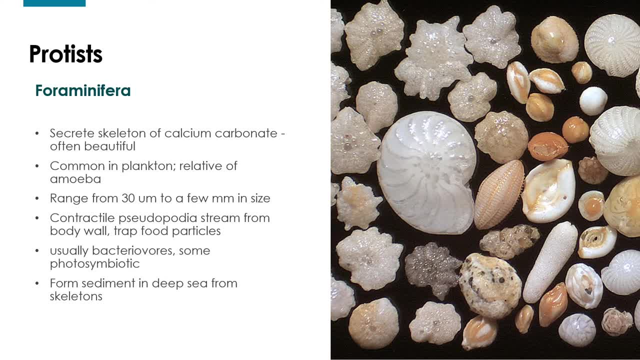 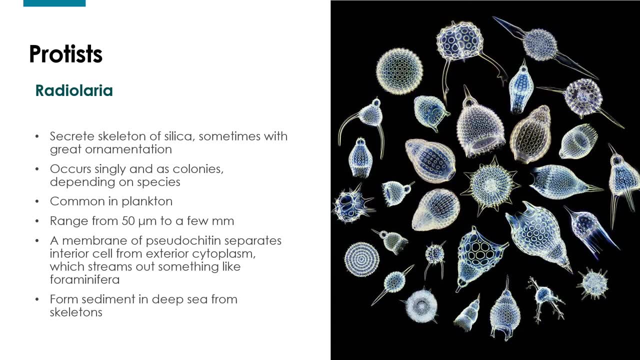 deep into the sediment, typically along the sea floor. and then next we have radioleria, and these two also secrete a skeleton, but this one made out of silica, and sometimes the designs can be quite ornate, as you can see in this image here, and they: 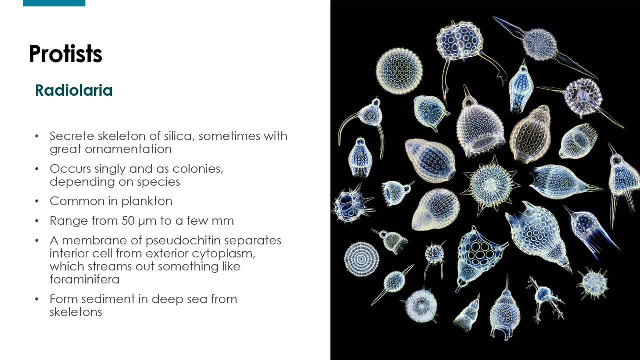 occur either singularly or in colonies, depending on the type of species, and these are also a common type of plankton that can range in size from 50 micrometers to a few millimeters, and some of the radiolarians that i've seen in samples i could definitely see just with the naked eye, and they 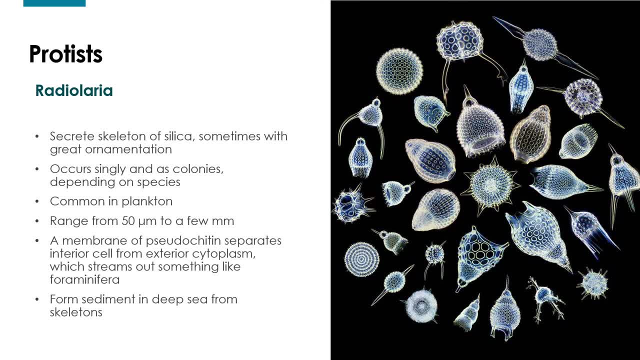 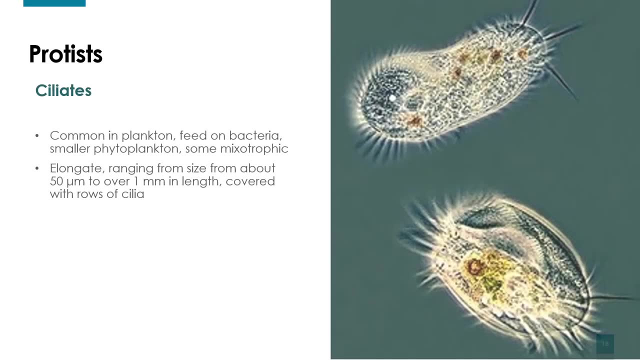 have a membrane of pseudokitin that separates the interior cell from the exterior cytoplasm, and they also form sediment deep within, or form sediment deep in deep sea from skeletons. and then, lastly, we have ciliates, and so ciliates are common types of plankton that feed on bacteria. 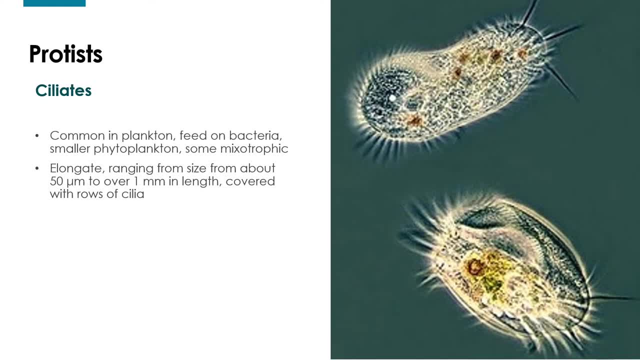 and other types of smaller phytoplankton, and so this sometimes makes them mix socially with each other, and that's why they're called ciliates. ciliates are common types of plankton, and so ciliates are common types of plankton, and they 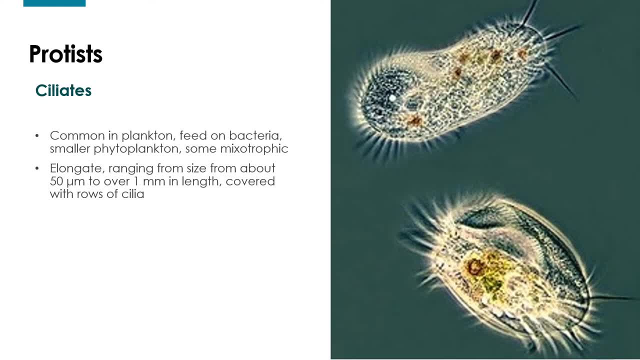 can they have more of a long, like a long get body structure, and they range in size from about 50 micrometers to over a millimeter in length, and and they can be covered in rows of cilia, like you can see in this image here. and so protists again are very unique in that they are 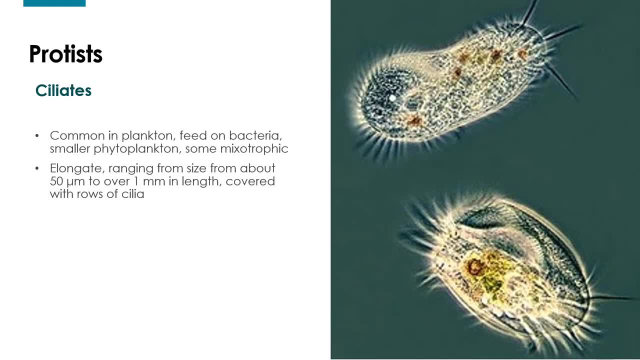 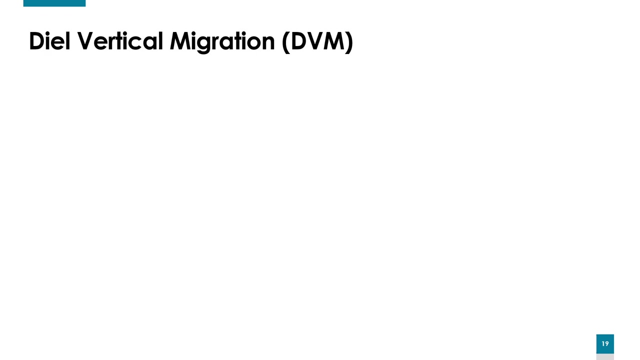 not easily confined to a particular category, and so we're learning, constantly learning new things about protists, and so our information um can quickly change from year to year, depending on what new discoveries are found about about protists. so i want to briefly talk about deal vertical migration and its importance in why zooplankton. 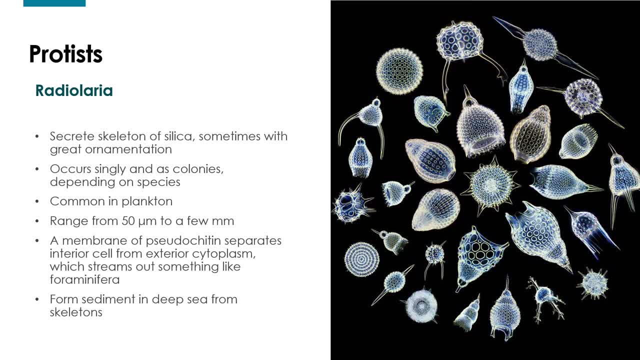 And they occur either singularly or in colonies, depending on the type of species, And these are also a common type of plankton that can range in size from 50 micrometers to a few millimeters, And some of the radiolarians that I've seen in samples. 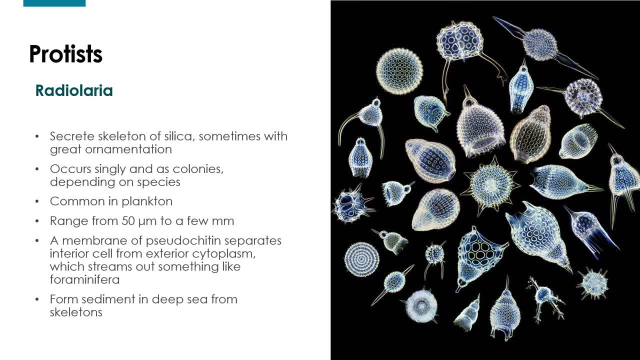 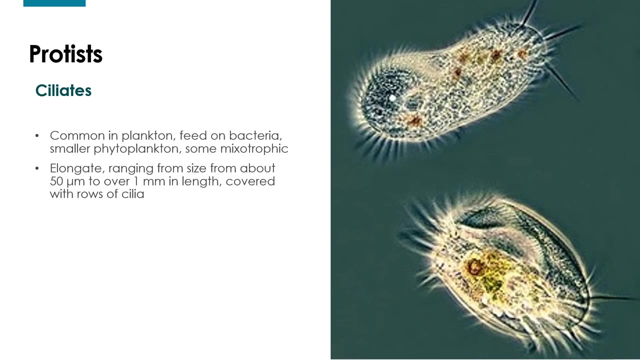 I could definitely see just with the naked eye, And they have a membrane of pseudokitin that separates the interior cell from the exterior cytoplasm, And they also form sediment deep within or form sediment deep in deep sea from skeletons. And then, lastly, we have ciliates. 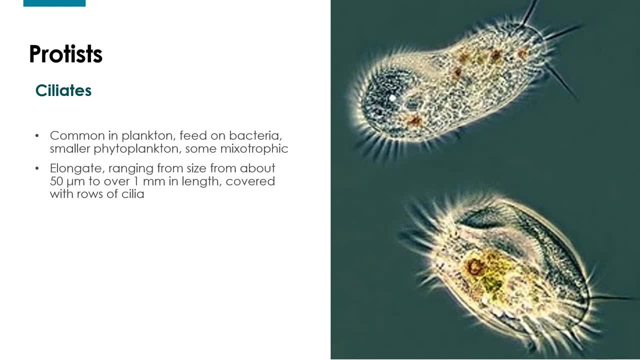 And so ciliates are common types of plankton that feed on bacteria and other types of smaller phytoplankton, And so this sometimes makes them mixotrophic, And they can. they have more of a long body structure and they range in size. 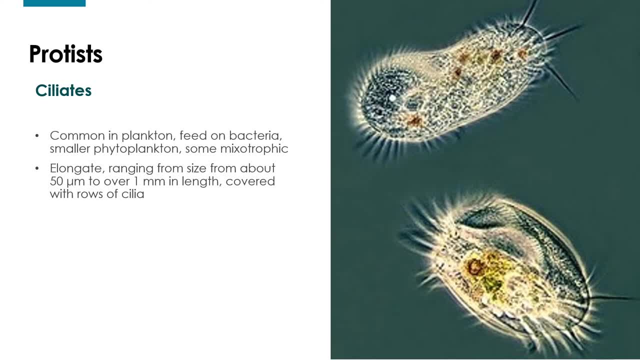 from about 50 micrometers to over a millimeter in length, And they can be covered in rows of cilia, like you can see in this image here, And so protists again are very unique in that they are not easily confined. 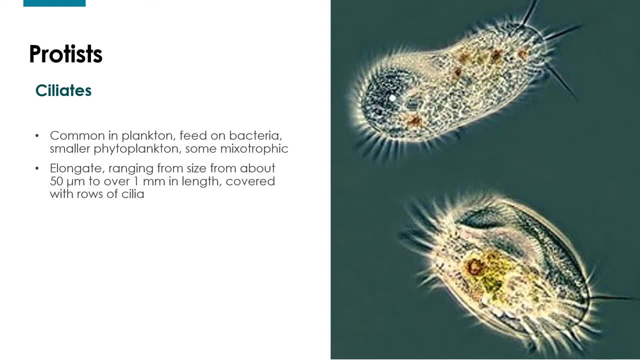 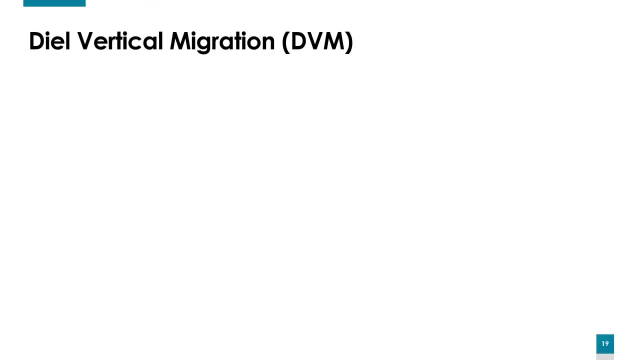 to a particular category, And so we're learning, constantly learning new things about protists, And so our information can quickly change from year to year, depending on what new discoveries are found about protists. So I want to briefly talk about deal vertical migration. 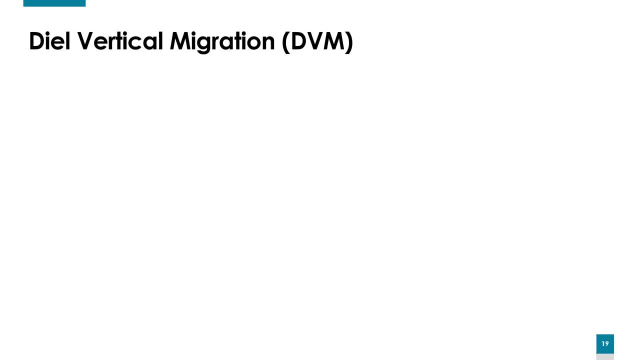 and its importance in why zooplankton do this and how it affects coastal communities and also communities at lower depths in the water column. And so deal vertical migration. to define it is synchronized movement of zooplankton that move up and down the water column. 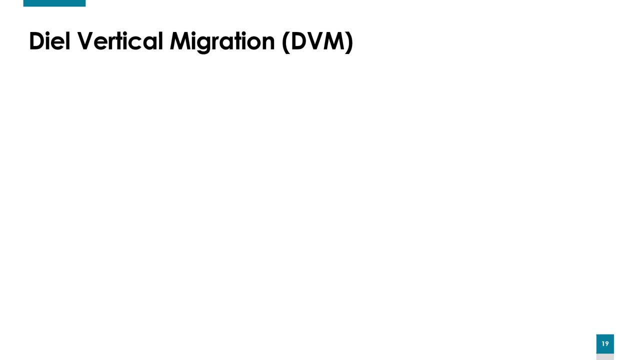 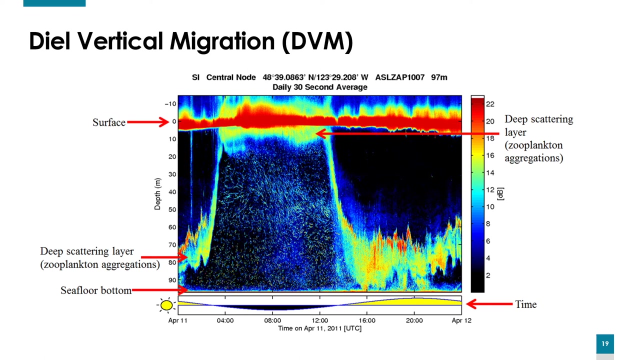 over a daily cycle, And a lot of people think that this may be the largest natural daily movement of biomass on our planet. And to show what this looks like, here I have an image of a eco-sounder images that were collected using a zooplankton acoustic profiler. 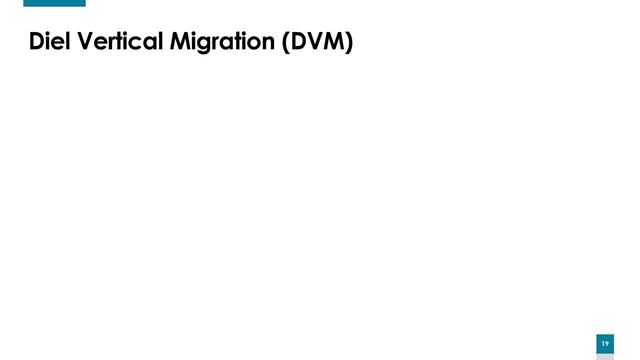 do this and how it affects um community or coastal communities and also um communities at lower deck or depths in the water column, and so deal vertical migration. to define it is synchronized movement of zooplankton that move up and down the water column over a daily cycle and a lot of people. 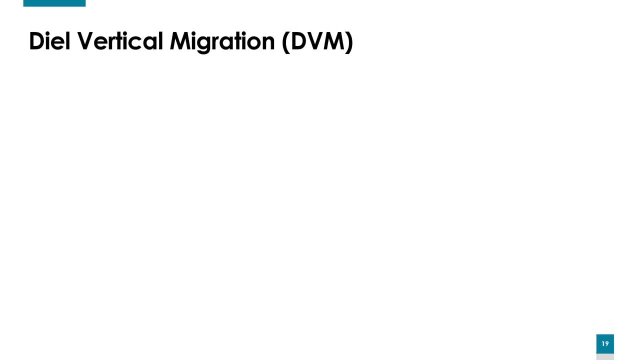 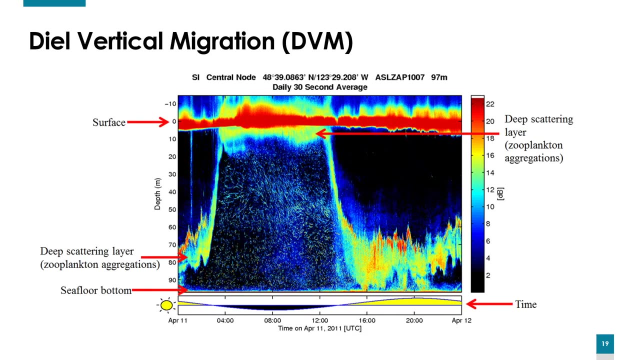 think that this may be the largest natural daily movement of biomass on our planet, and to show what this looks like, here i have an image of um, a eco sounder, images that were collected using a zooplankton acoustic profiler, and this is a type of active sonar system that 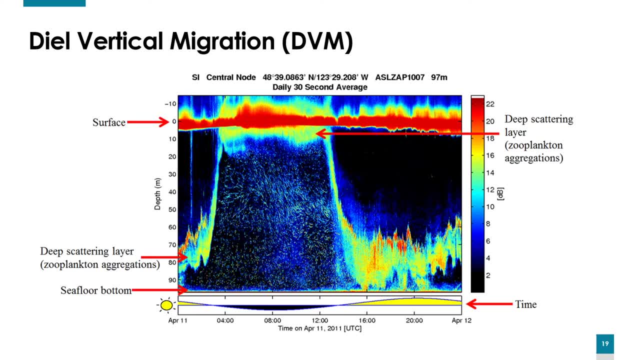 both transmits and receives acoustic or sound signals underwater, and by doing this we can actually kind of visualize aggregations of of whatever actually really is. um is sitting in the water at depth, and so what we see here if we look at the surface, um, everything is nice and labeled, so we have surface, and then 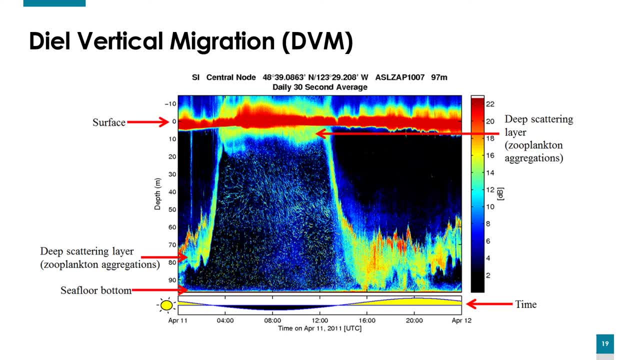 down below, over and between 70 and 90 meters, we have an aggregation of zooplankton at what looks like, probably around um 12 am or so, and as we get towards um near dawn we see that the aggregations of zooplankton start to move up in the water column. so the trigger as to 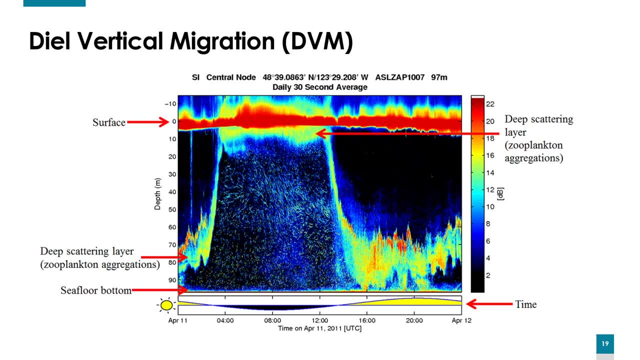 why this is occurring? um can be a change in light intensity, which is probably the most likely trigger for deal. vertical migration. um and then also changes in depth are associated with. could be associated with cloud cover or eclipses, phases of the moon. um all these fluctuations in 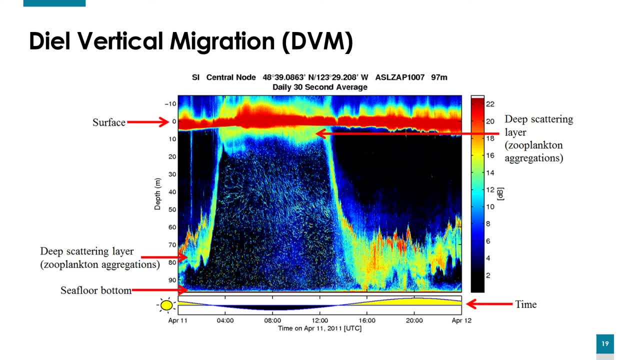 light, basically intensity, so like light, plays a significant role in how zooplankton travel up and down the water column and, as you can see, over a period of about 12 hours the zooplankton are near surface, most likely feeding on phytoplankton and then, as the sunlight dissipates over the evening. 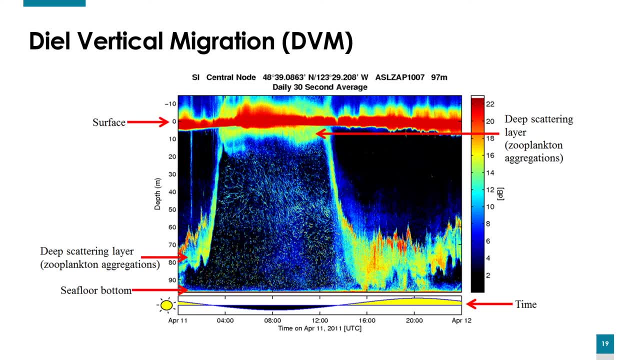 And this is a type of active sonar system that both transmits and receives acoustic or sound signals underwater, And by doing this we can actually kind of visualize aggregations of of whatever actually really is is sitting in the water at depth. 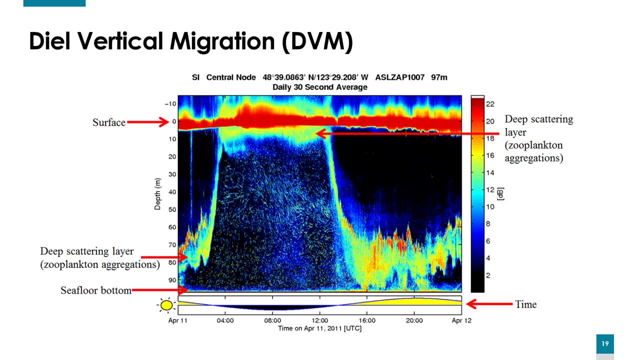 And so what we see here. if we look at the surface, everything is nice and labeled, So we have surface, and then down below and between 70 and 90 meters we have an aggregation of zooplankton at what looks like. 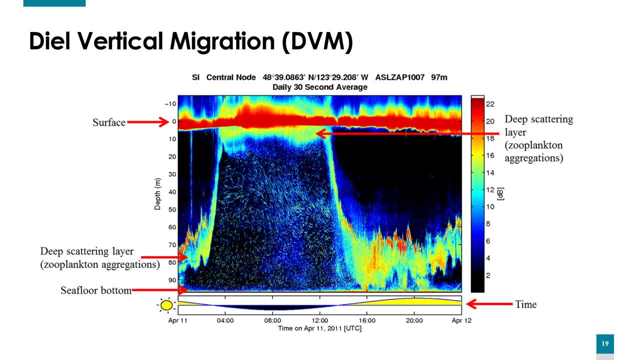 probably around 12 am or so, And as we get towards near dawn we see that the aggregations of zooplankton start to move up in the water column, So the trigger as to why this is occurring can be a change in light intensity. 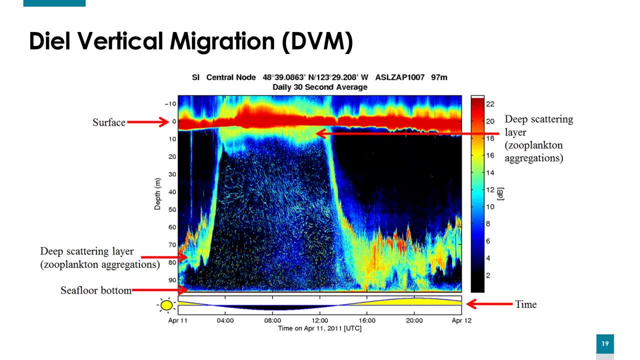 which is probably the most likely trigger for deal. vertical migration And then also changes in depth are associated with. could be associated with cloud cover or eclipses, phases of the moon, all these fluctuations in light, basically intensity, So like light plays a significant role. 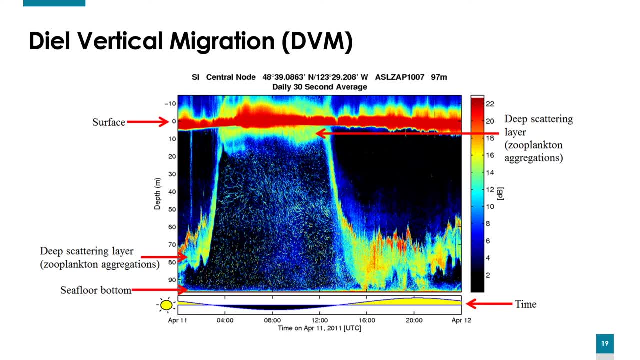 in how zooplankton travel up and down the water column And, as you can see, over a period of about 12 hours. the zooplankton are near surface, most likely feeding on phytoplankton, And then, as the sunlight dissipates. 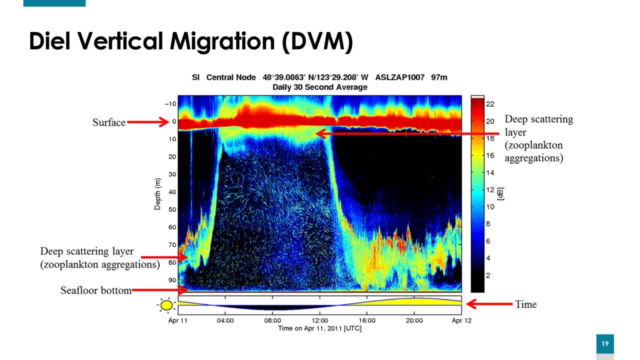 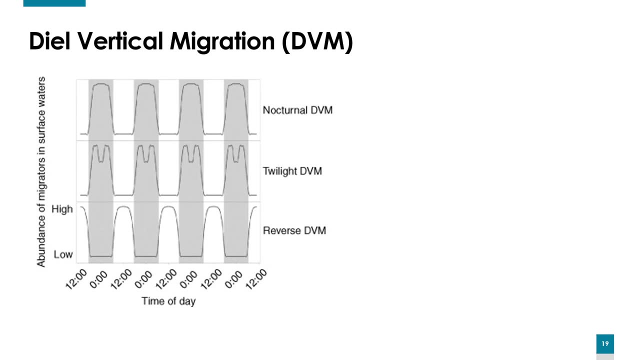 over the evening or the afternoon, the aggregation of zooplankton go back down to depth and reside there throughout the night and then starting the cycle over the next day. So there's different types of deal: vertical migrations. There's nocturnal, one period of maximum biomass. 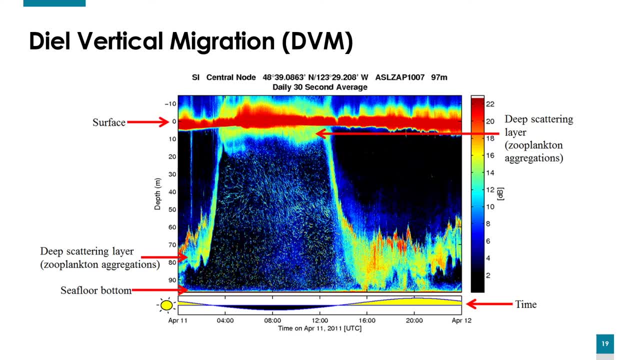 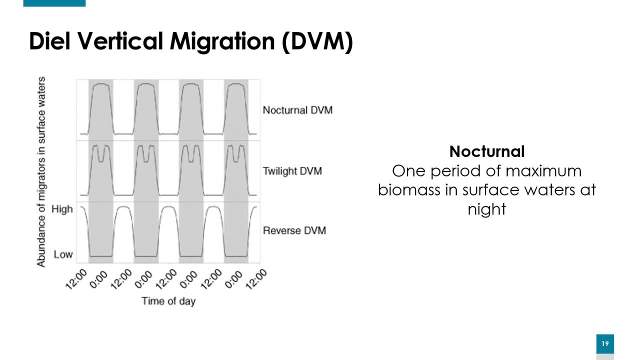 or the afternoon, the aggregation of zooplankton go back down to depth and reside there throughout the night and then starting the cycle over the next day. so there's different types of deal: vertical migrations. there's nocturnal, one period of maximum biomass and surface waters at night. 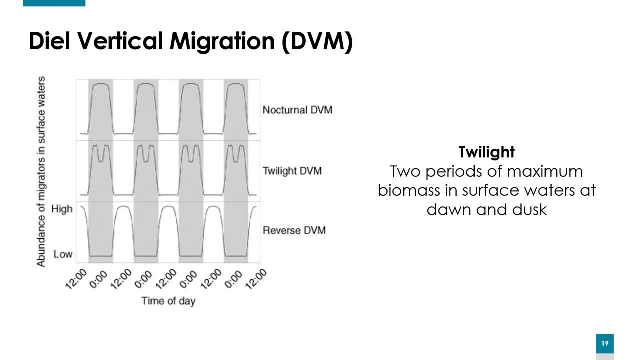 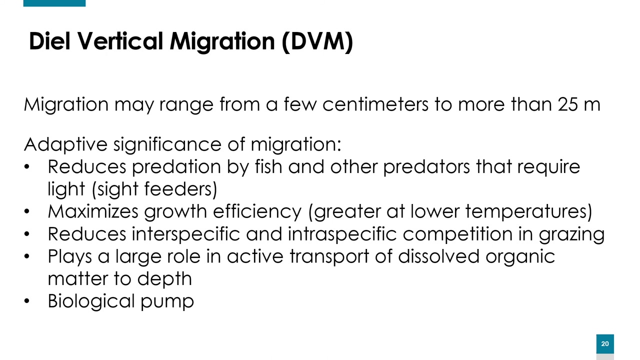 there are twilight, where two periods of maximum biomass and surface waters at dawn and at dusk, and then there's reverse, dvm, which is one period of maximum biomass and surface waters during the daylight, and so with deal vertical migration: the zooplankton are more likely to migrate to the surface during the day, and so the range of 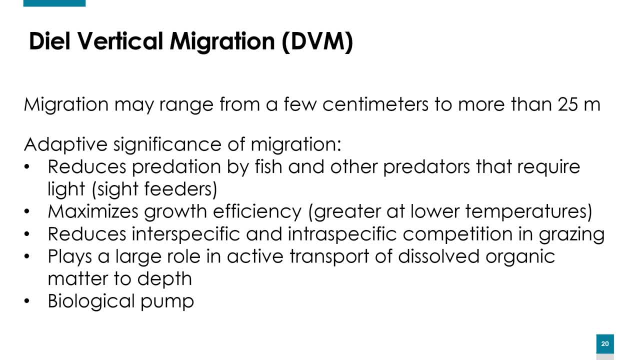 what this occurs. that could be between a few centimeters or more than 25 meters, and what we could see in the previous image is that it definitely was in a much larger range, and some of the reasons why zooplankton might prep or perform deal vertical migration is to perhaps reduce 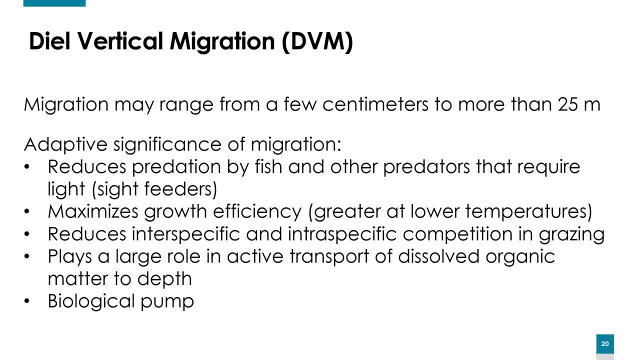 predation by fish and other predators that require sight or, i'm sorry, require light, so they're site feeders, so predation. other reasons could include maximizing growth efficiency, reducing interspecific and intraspecific competition in grazing, and dvm plays a large role in the active transport of dissolved 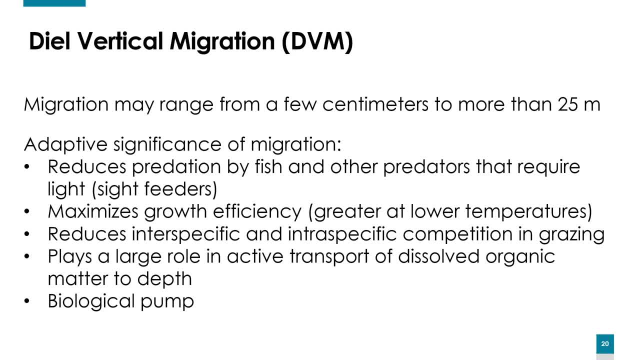 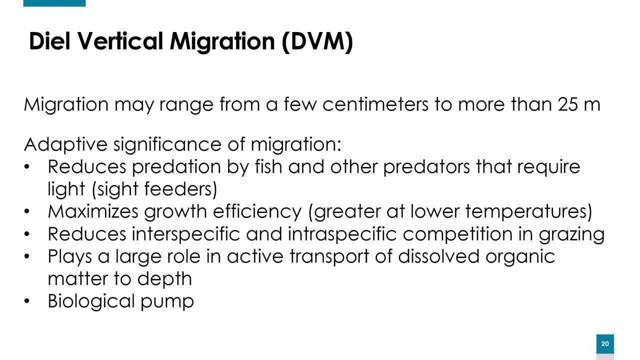 of calcium carbonate. so when zooplankton are going up and down the water column, they are eating the phytoplankton, so thus ingesting the co2 that has been that has been converted by the phytoplankton, as well as creating fecal pellets that drop in the 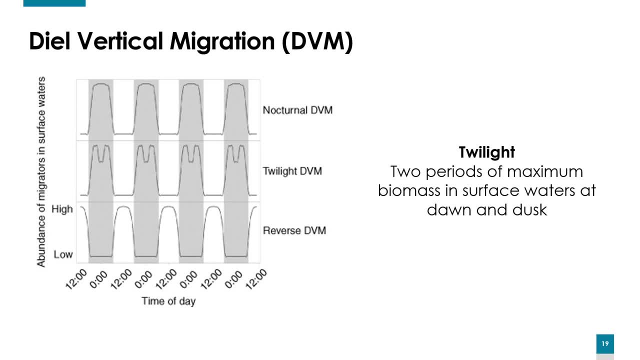 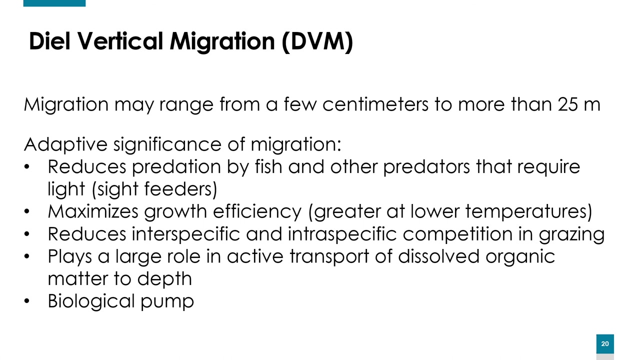 in surface waters at night There are twilight, where two periods of maximum biomass in surface waters at dawn and at dusk, And then there's reverse DVM, which is one period of maximum biomass in surface waters during the daylight, And so with deal vertical migration. 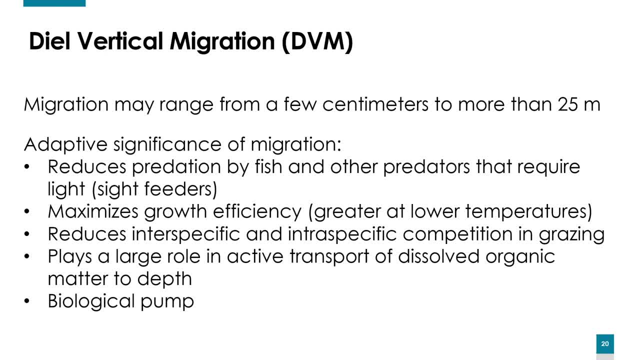 the range of what this occurs at could be between a few centimeters or more than 25 meters, And what we could see in the previous image is that it definitely was in a much larger range And some of the reasons why zooplankton might pre-. 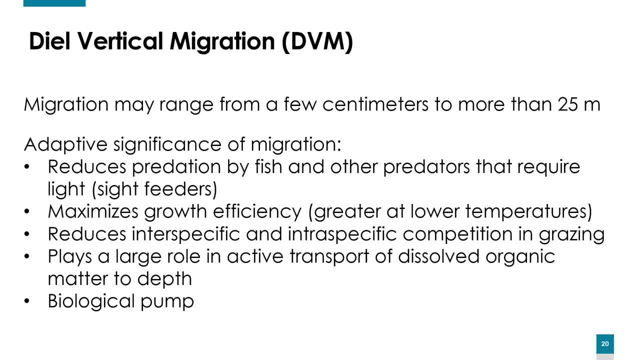 or perform deal. vertical migration is to perhaps reduce predation by fish and other predators that require sight or, I'm sorry, require light. So they're sight feeders. So the zooplankton will stay at depth during the day to avoid predation. 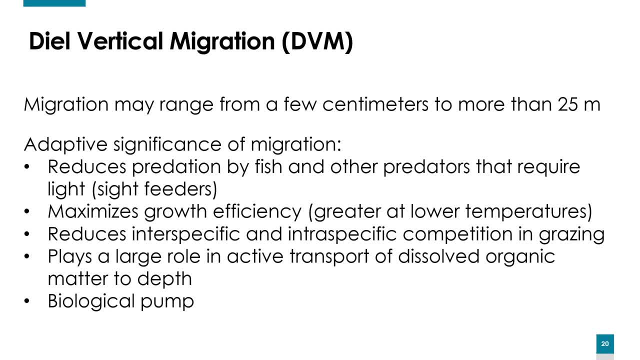 Other reasons could include maximizing growth efficiency, reducing interspecific and intraspecific competition in grazing, And DVM plays a large role in the active transport of dissolved organic matter to depth, So we're talking about the biological pump And what that is. 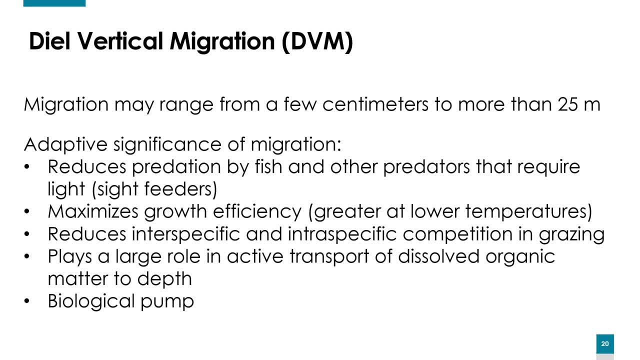 is that it's the conversion of CO2 and inorganic nutrients by phytoplankton during photosynthesis, as well as the cycling of calcium carbonate. So when zooplankton are going up and down the water column, they are eating the phytoplankton. 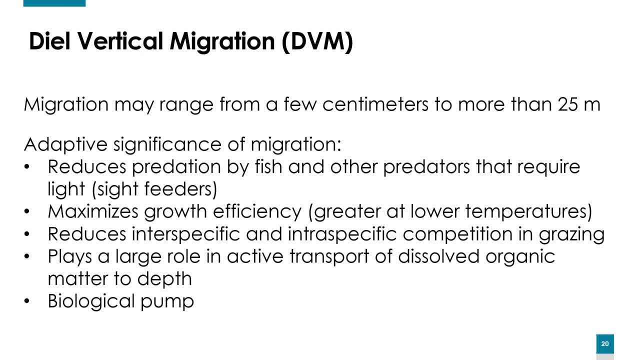 so thus ingesting the CO2 that has been converted by the phytoplankton, as well as creating fecal pellets that drop in the water column. And all of this falls down into different depths of the water column, which provide nutrients that other marine organisms need. 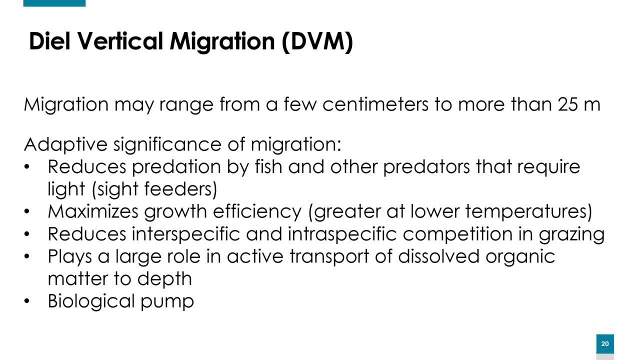 in order to survive, And so DVM is a pretty important process, and hopefully maybe someone in the future would be interested in diving deeper- no pun intended- into expanding on why this is an important role in our ecosystem and why zooplankton are encouraged. 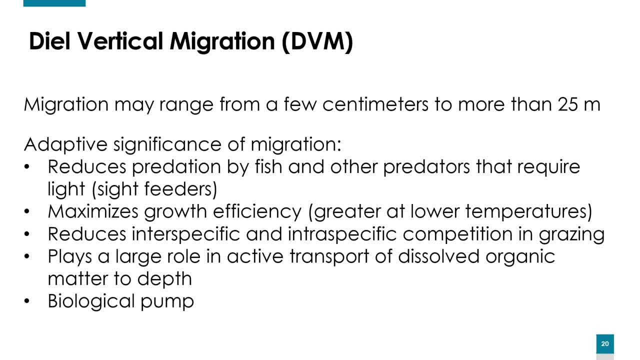 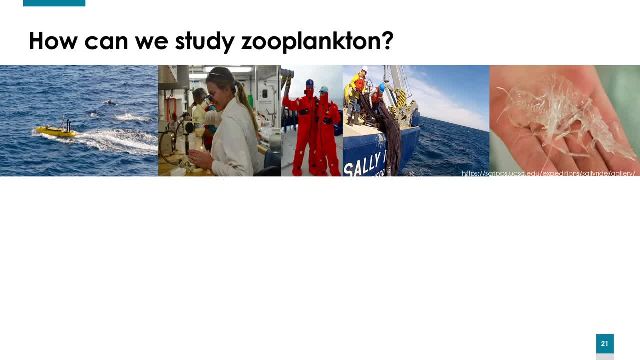 or have adapted to perform this. Okay, so now that we have covered some ground on what zooplankton are and getting a basic introduction, now we can start asking some questions about how can we study zooplankton. And for as long as people have been curious, 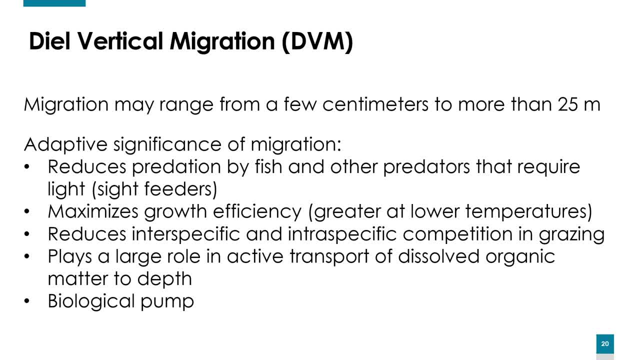 water column and all this falls down into different depths of the water column which provide nutrients to other marine organisms need in order to survive. and so dvm is pretty important process and hopefully maybe someone in the future would be interested in diving deeper- no pun intended- into expanding on why this is an important role in our 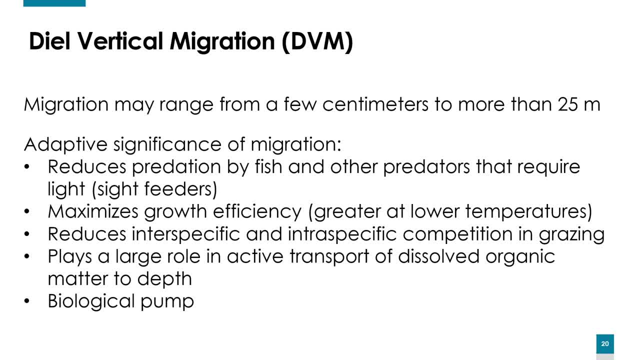 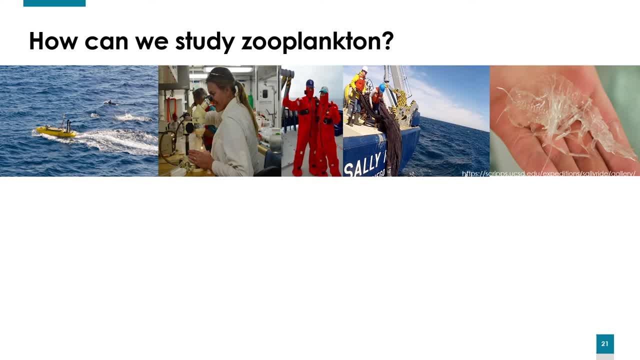 ecosystem and why zooplankton are encouraged or have adapted to perform this. okay, so now that we have covered some ground on what zooplankton are and getting a basic introduction, now we can start asking some questions about how can we study zooplankton and for as long as. 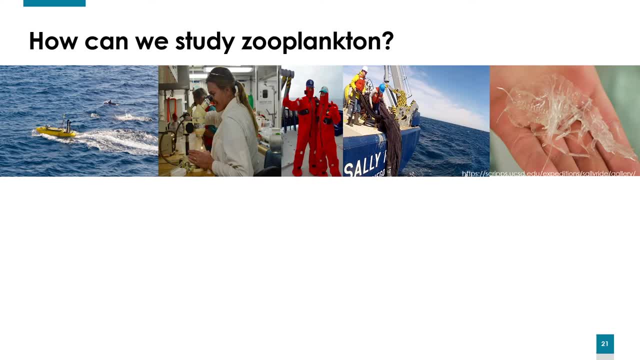 people have been curious about the natural world. scientists have been trying to answer this question, and different themes that we can start to think about in terms of how to study zooplankton might include diversity or, as a mesma, reason for based on different insect species. and the next couple of slides we're going to go ahead and dive into different examples of what current grad students 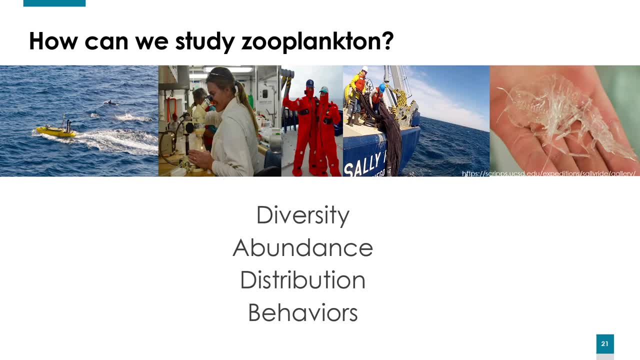 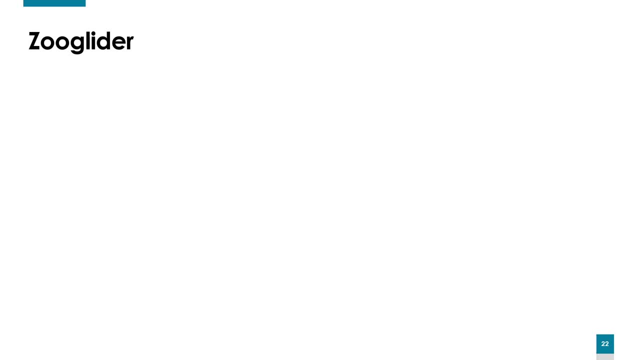 and past grad students have worked on to better answer. how can we study zooplankton? first up, we have ben whitmore and he studied zooplankton, predator-prey interactions, and today's about where zooplankton or replied to the zooplankton on the sea is that we have to start applying. 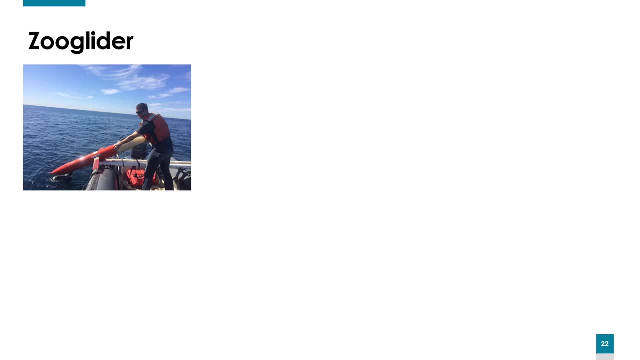 And typically sample collection is done by using a large net, whether it's a bongo net, And in this case, for a lot of samples that Ben had looked at, it was collected by using the mock nets, And the mock nets is a multiple opening, closing net and environmental sensing system. 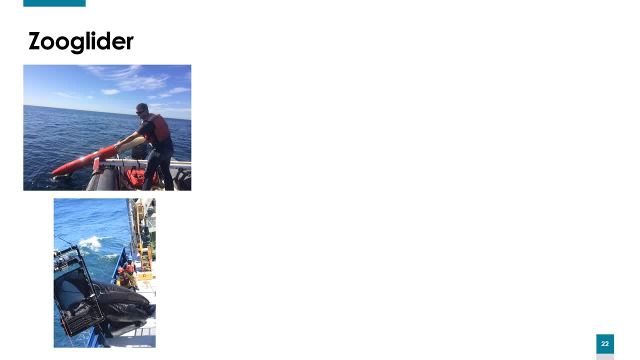 That's the acronym for mock nets, And it collects zooplankton at different depths in the water column And then these samples are brought back to surface and are preserved, And so, while this is a good way to look at the different types of zooplankton that are at different depths, 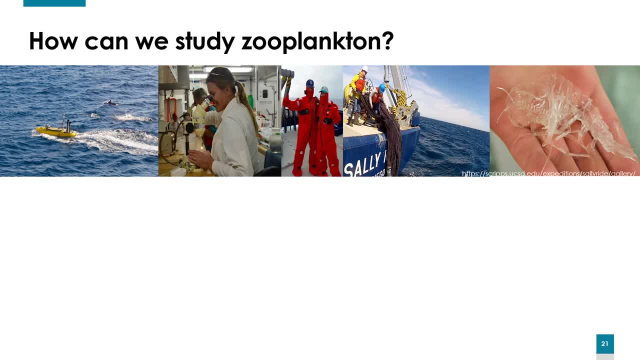 about the natural world? scientists have been trying to answer this question, And different themes that we can start to think about in terms of how to study zooplankton might include diversity, abundance distribution or behaviors. And the next couple of slides: 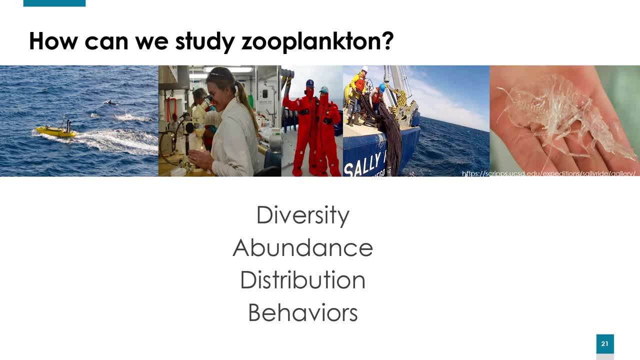 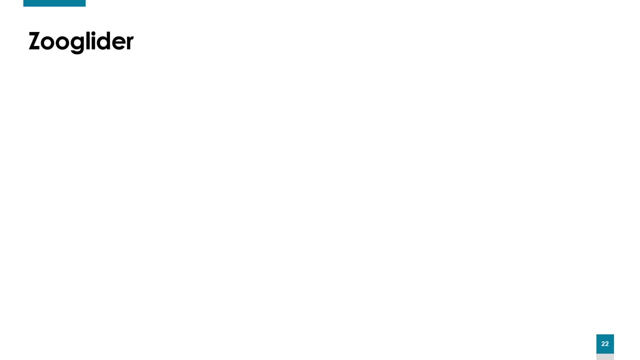 we're going to go ahead and dive into different examples of what current grad students and past grad students have worked on to better answer. how can we study zooplankton? First up we have Ben Whitmore and he studied zooplankton-predator-prey interactions. 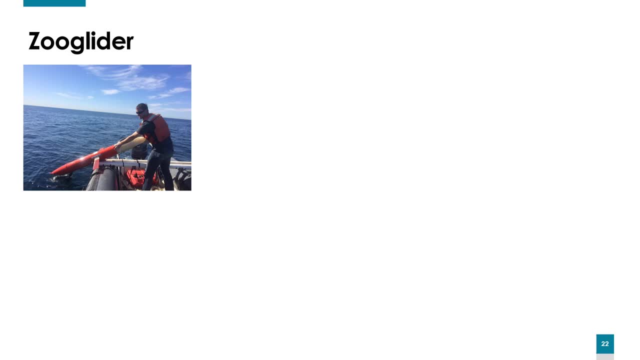 And typically sample collection is done by using a large net, whether it's a bongo net, And in this case, for a lot of samples that Ben had looked at, it was collected by using the MOCNES, And the MOCNES is a multiple opening-closing net. 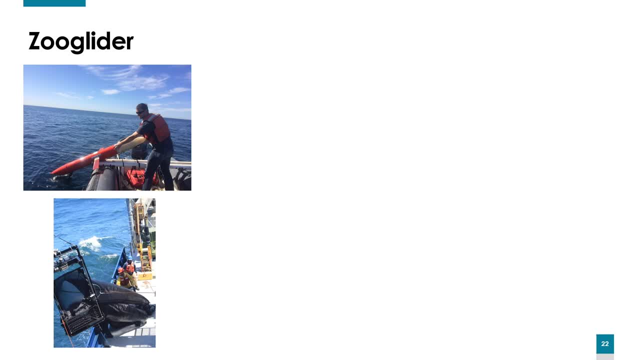 and environmental sensing system- That's the acronym for MOCNES- And it collects zooplankton at different depths in the water column, and then these samples are brought back to surface and are preserved. And so, while this is a good way, 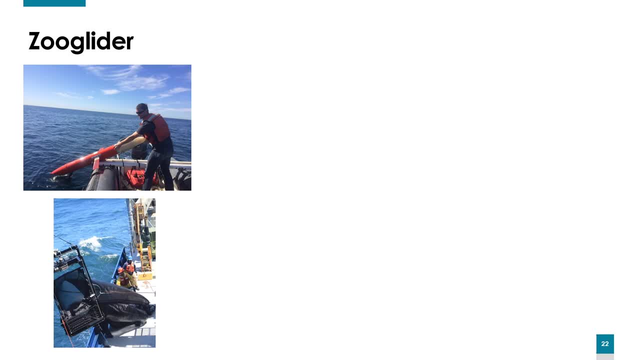 to look at the different types of zooplankton that are at different depths. it's not the best way to observe how far apart organisms are, and it makes it almost impossible to study zooplankton-predator-prey interactions. So, instead, what Ben had done, 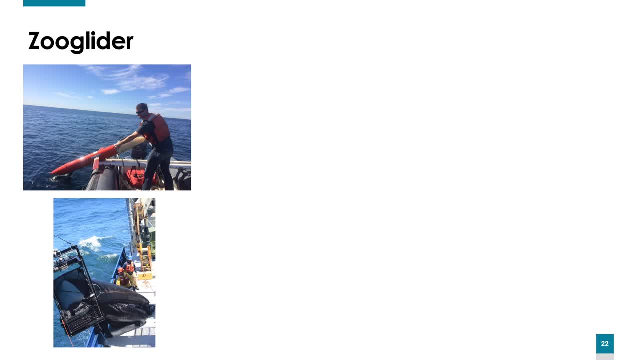 instead of using a net. he helped come up with the idea of using a high-resolution camera called the ZoCam and that is attached to an unmanned submersible that glides through the water very slowly, about four inches per second. So this is called the ZoGlider. 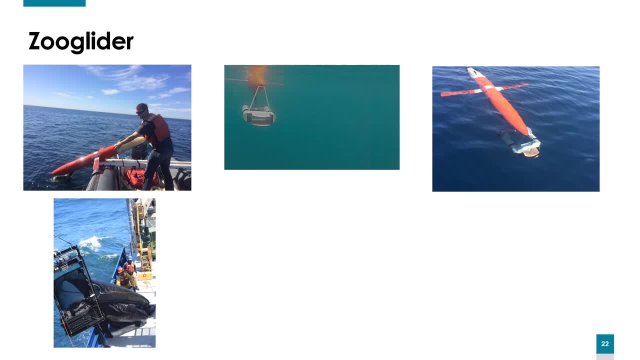 And here we have two different images of the ZoGlider in action And, as you can see, the ZoCam is attached at the bottom here or at the end of the ZoGlider, and the submersible can stay. goes on deployments. 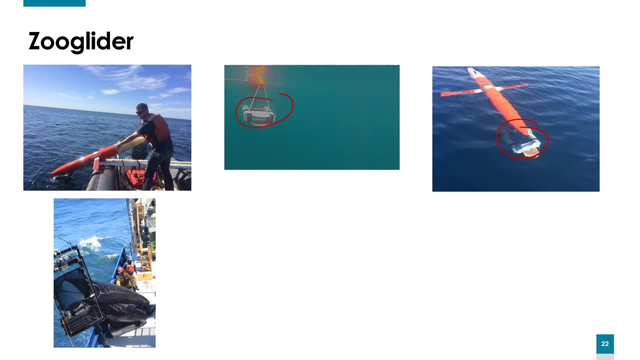 between 14 and 30 days, And the types of metadata that are collected from the ZoGlider would include depth and time, so that allows Ben to get a better picture or tell more accurately how far apart the zooplankton are. And so, with that metadata, 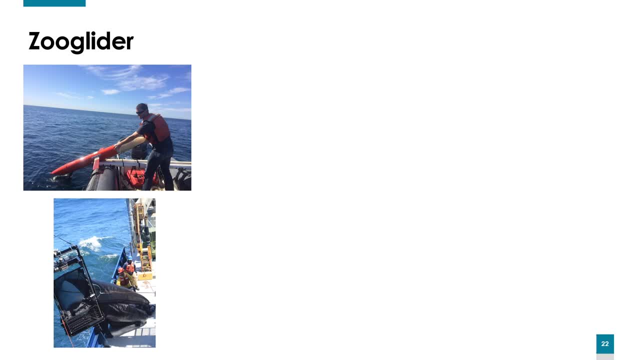 it's not the best way to observe how far apart organisms are And it makes it almost impossible to study zooplankton predator-prey interactions. So instead, what Ben had done, instead of using a net, he helped come up with the idea of. 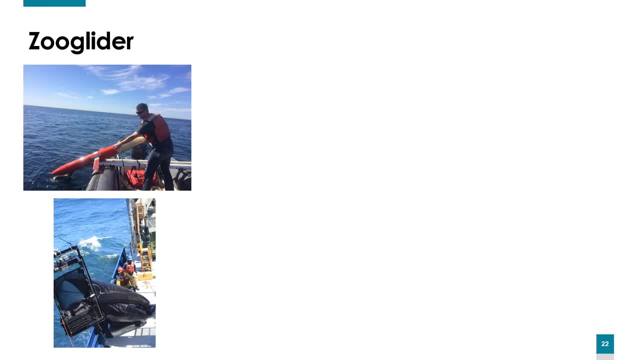 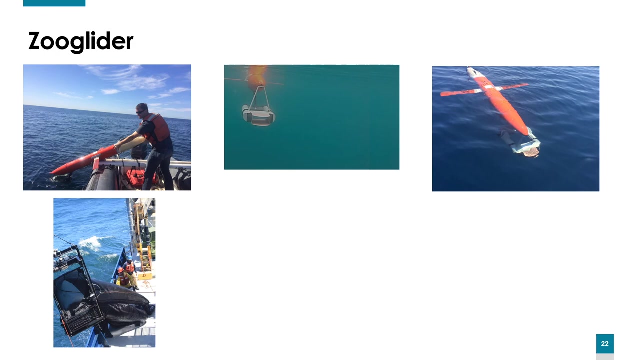 using a high-resolution camera called the Zocam And that is attached to an unmanned submersible that glides through the water very slowly, about four inches per second. So this is called the Zoglider, And here we have two different images of the Zoglider in action. 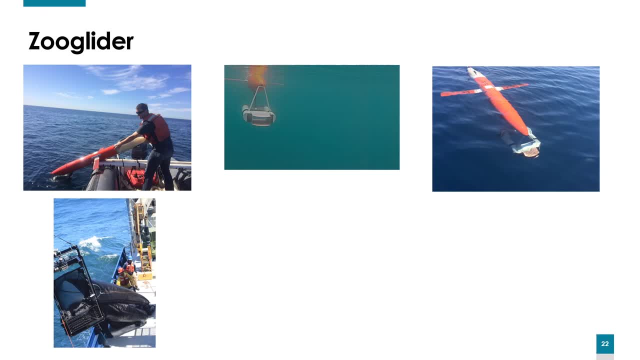 And, as you can see, the Zocam is attached at the bottom here or at the end of the Zoglider And the submersible can stay. goes on. deployments between 14 and 30 days And the types of metadata that are collected from the Zoglider would include depth and time. 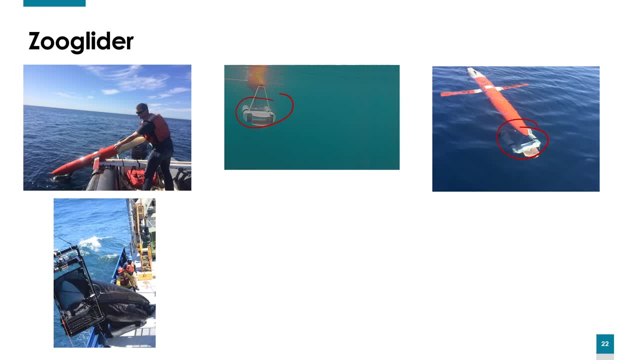 so that allows Ben to get a better picture or tell more accurately how far apart the zooplankton are. And so, with that metadata, when he is able to pull these images from the zooplankton, and he is able to pull these images from the zooplankton, 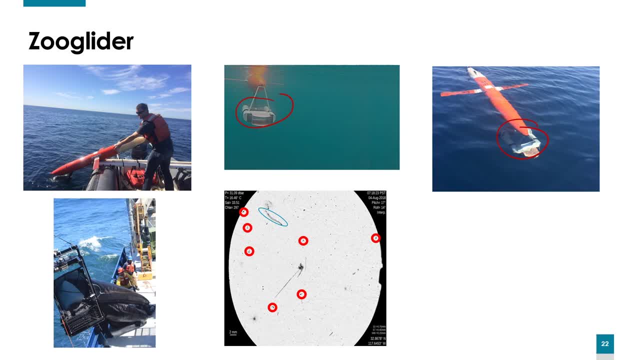 and he is able to pull these images from the zooplankton, he can see where the predator and potential prey are in a much better sense than if we were just to collect it with a net. And so in this image here we see that marked in blue what looks like a chetignath perhaps. 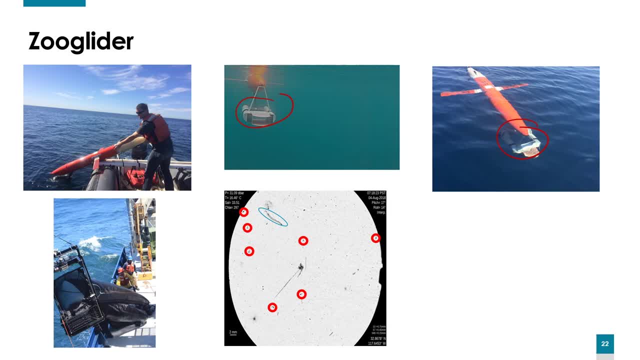 and surrounding it in the red circles are its potential prey items, which are most likely different types of copepod. And this is giving us a much better picture of the Zoglider. And this is giving us a much better picture of the Zoglider. 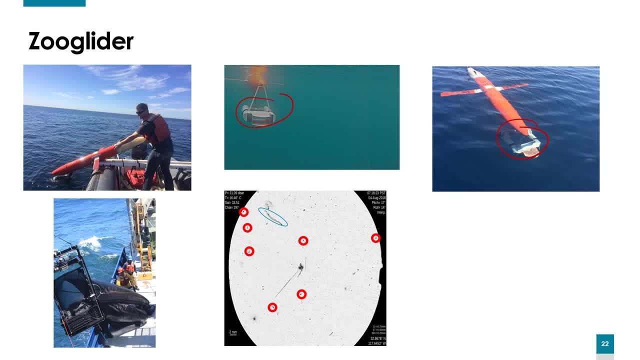 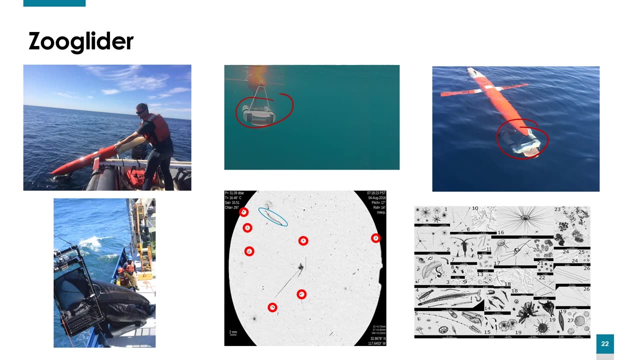 And this is giving us a much better picture of the Zoglider, And this is giving us a much better picture and representation of the amount of prey available in relation to the different types of predators that are within the water column. Another benefit of using the Zocam is that it generates these amazing images that have a lot of detail. 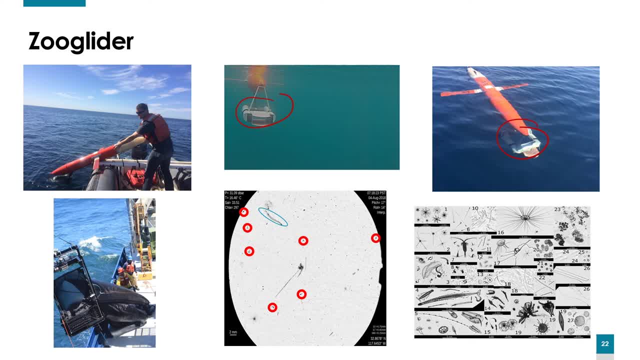 And the difference between these images and the images I'm going to show you with the Zoscan that I use is that the Zoglider is able to collect special data to capture the zooplankton in their natural posture, which is really important. 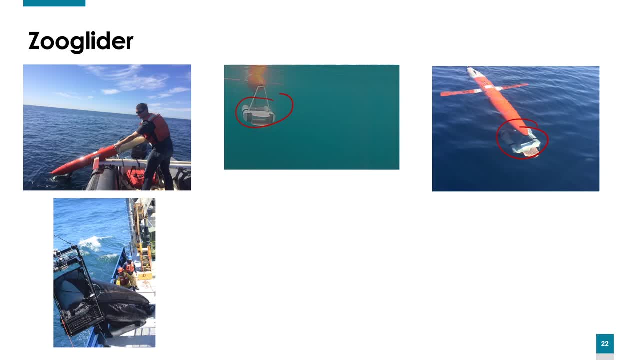 when he is able to pull these images from the ZoCam, he can see where the predator and potential prey are in a much better sense than if we were just to collect it with a net, And so in this image here we see that marked in blue. 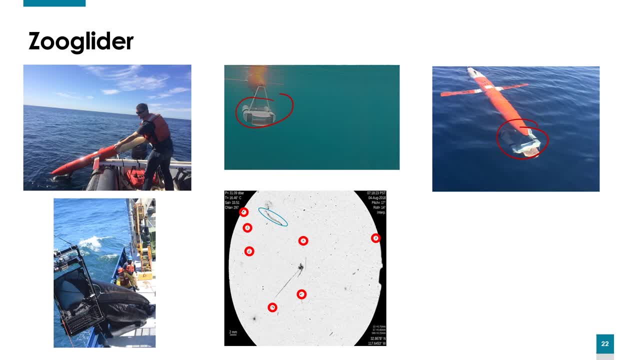 what looks like a chetignath perhaps, and surrounding it in the red circles are its potential prey items, which are most likely different types of copepod, And this is giving us a much better picture and representation of the amount of prey available. 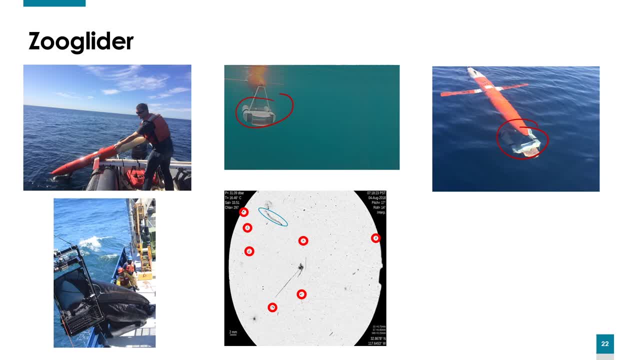 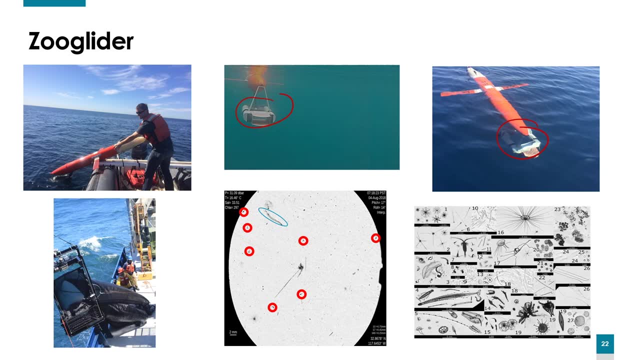 in relation to the different types of predators that are within the water column. Another benefit of using the ZoCam is that it generates these amazing images that have a lot of detail, And the difference between these images and the images I'm going to show you. 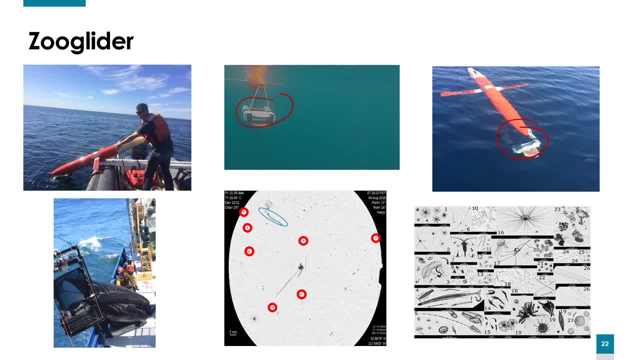 with the ZoScan that I use is that the ZoGlider is able to capture the zooplankton in their natural posture, which is really important. So it gives us a better idea of what the different zooplankton look like naturally versus when they're preserved in formalin. 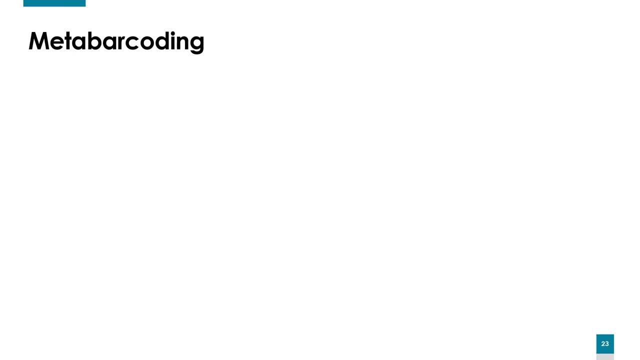 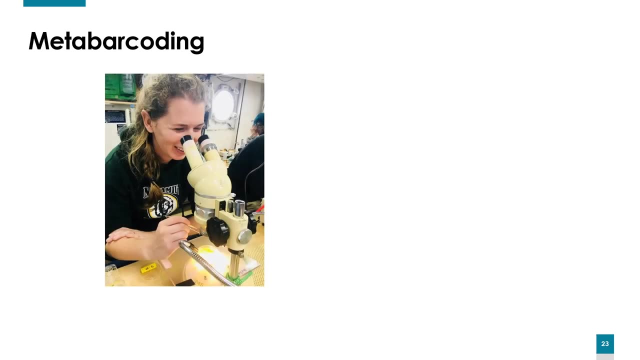 So next up we have Stephanie Matthews and she studies zooplankton in the mesopelagic part of the ocean. And so here we have Stephanie here looking at something that's called a mesopelagic zooplankton, And this is a very classic telescope. 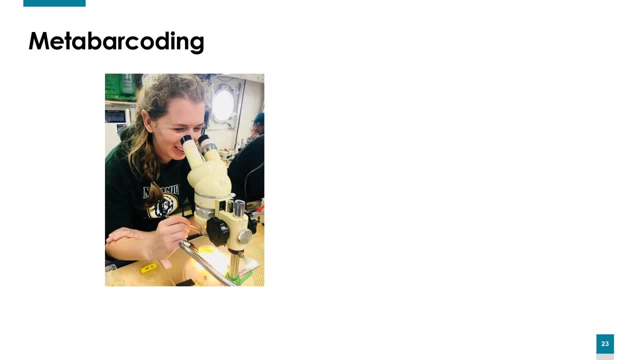 very classic And so mesopelagic zooplankton, which live in the deep ocean between 200 and 1,000 meters, are fairly small and are advected by ocean currents, And so they're usually eaten by pelagic fish. 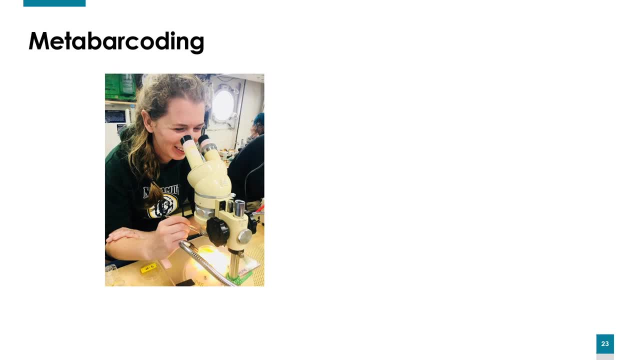 such as tuna or mahi-mahi. And again, Stephanie also uses the mock nest to collect samples. And also with the mock nest, salinity, oxygen and fluorescence is also gathered. So what Stephanie does is that she uses DNA sequencing to identify organisms present at each location. 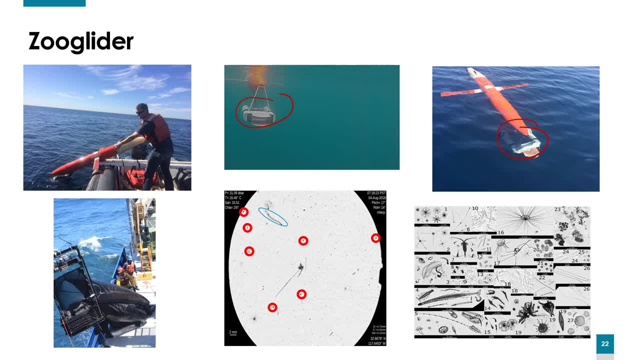 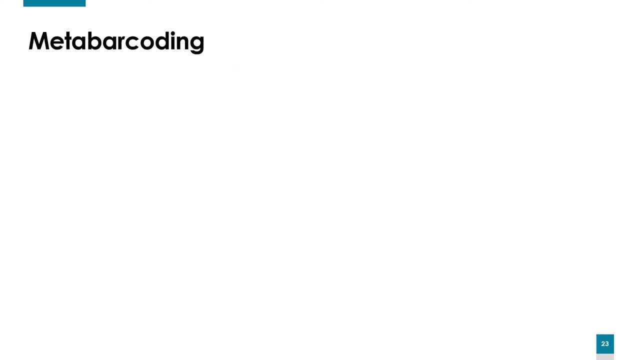 So it gives us a better idea of what the different zooplankton look like naturally versus when they're preserved in formalin. So next up we have Stephanie Matthews, and she studies zooplankton in the mesopelagic part of the ocean. 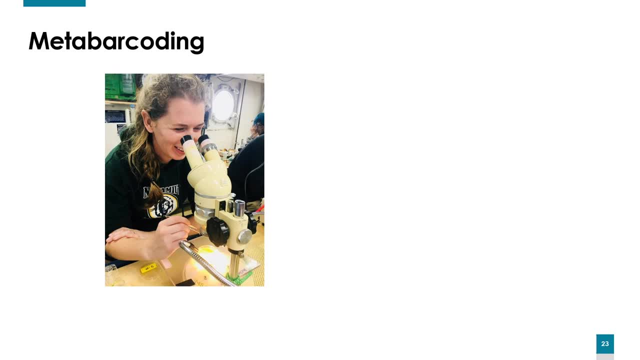 And so here we have Stephanie here looking at something at the microscope. very classic And so mesopelagic: zooplankton, which live in the deep ocean between 200 and 1,000 meters, are fairly small and are affected by ocean currents. 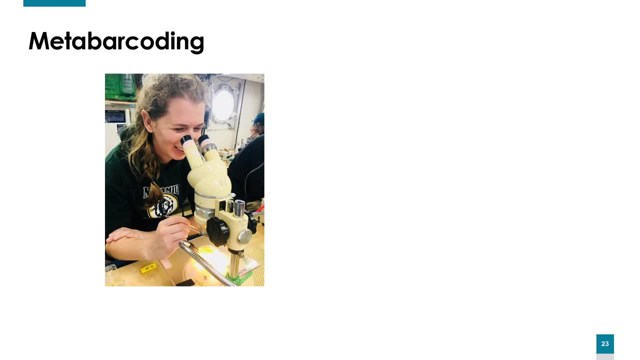 And so they're usually eaten by pelagic fish such as tuna or mahi-mahi. And again, Stephanie also uses the mock nest to collect samples And also, with the mock nest data, such as temperature, salinity and temperature. 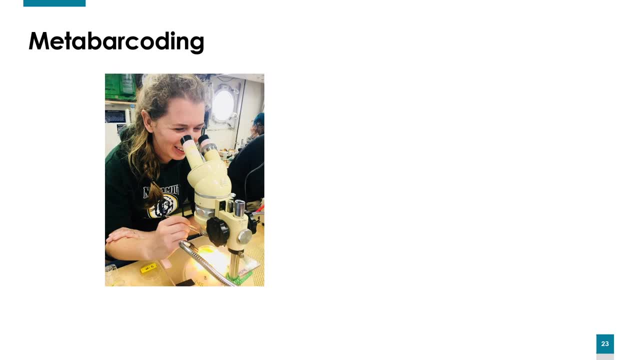 oxygen and fluorescence is also gathered. So what Stephanie does is that she uses DNA sequencing to identify organisms present at each location, And this is important because it can help her identify the different organisms that were sampled, And Stephanie does prefer this method over microscopy. 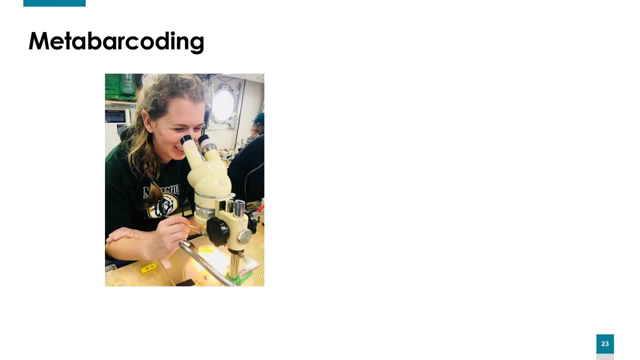 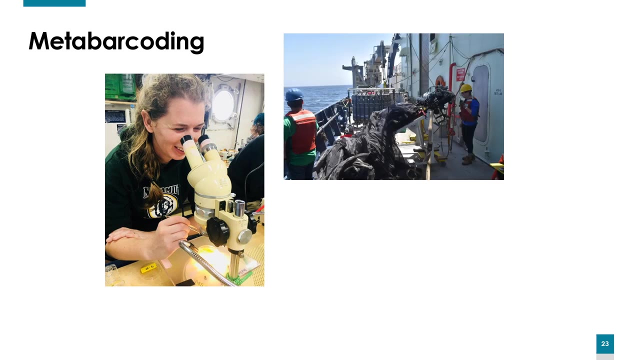 which I totally understand, And DNA analysis allows her to work with other scientists that are doing samples and doing sample collections in different parts of the ocean and compare and see what the diversity looks like. And so here we have her looking at getting the mock nest. 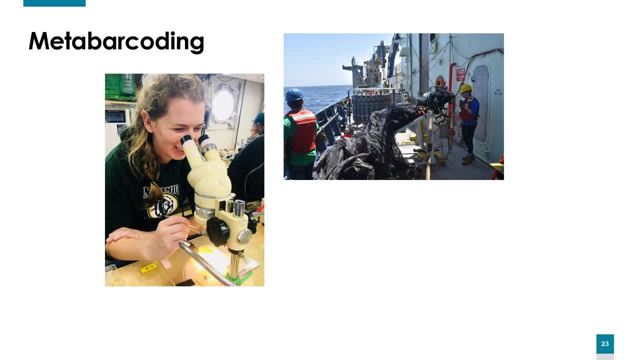 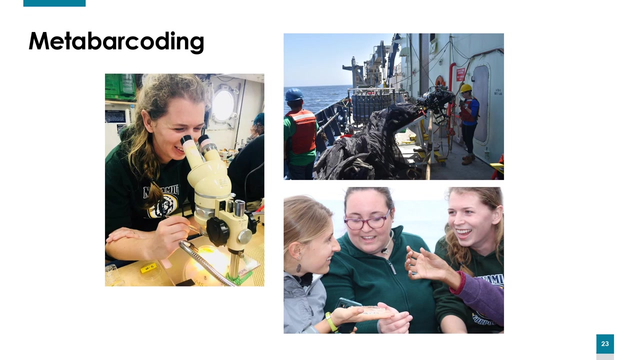 set up for deployment And her ultimate goal is to map the distribution of zooplankton species in the mesopelagic ocean so that she can understand the what aspects of the environment are important for the zooplankton survival, And so, if she can create a database, 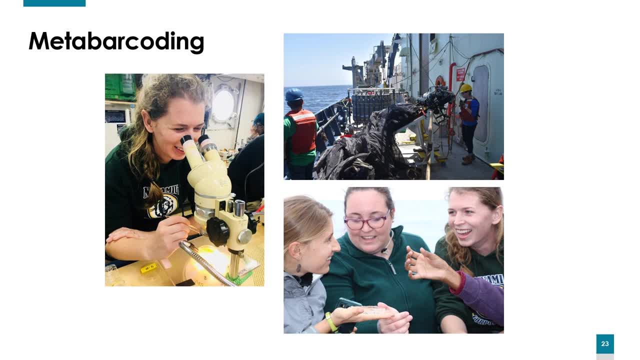 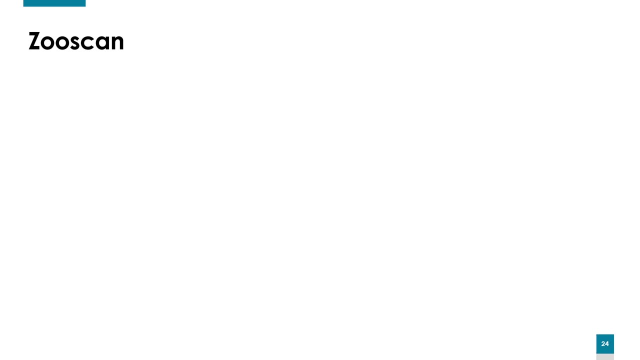 that includes many different species. with metal barcoding, then she can help other researchers as well identify the different, the abundance and diversity of zooplankton in the ocean. Okay, so now we're at the part where I talk about what I do. 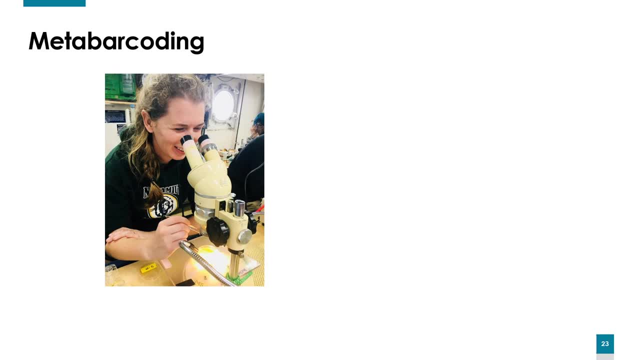 And this is important because it can help her identify the different organisms that were sampled- And Stephanie does prefer this method over microscopy, which I totally understand- And DNA analysis allows her to work with other scientists that are doing sample collections in different parts of the ocean. 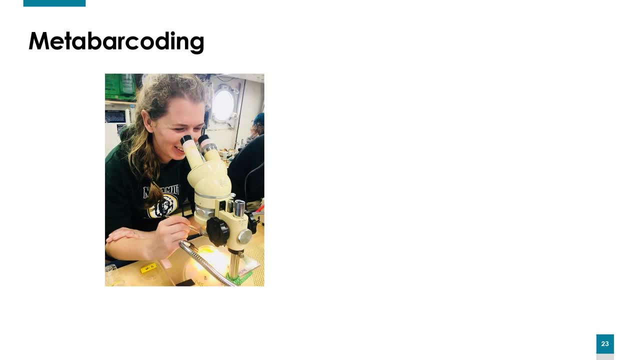 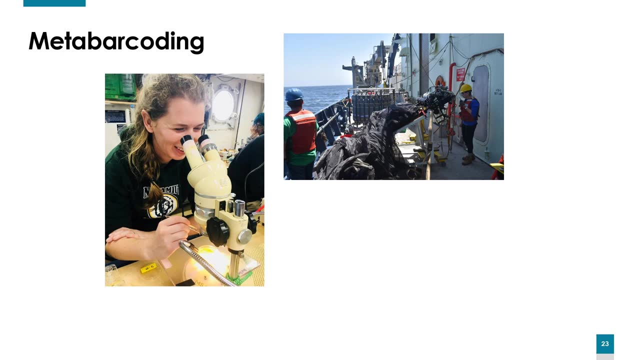 and compare and see what the diversity looks like. And so here we have her looking at or getting the mock nest set up for deployment, And her ultimate goal is to map the distribution of zooplankton. map the distribution of zooplankton species. 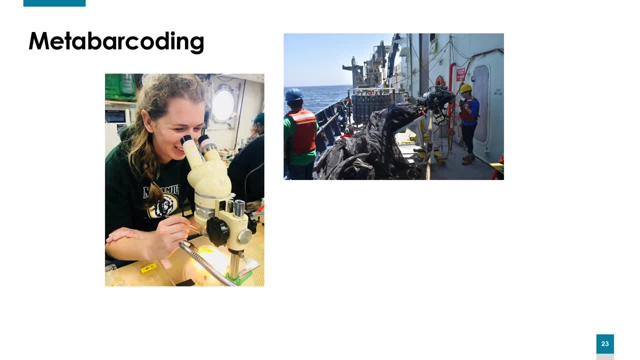 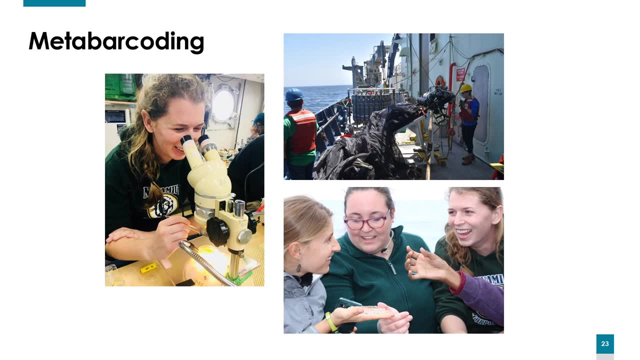 in the mesopelagic ocean so that she can understand what aspects of the environment are important for the zooplankton survival, And so if she can create a database that includes many different species with metal barcoding, then she can help other researchers as well. 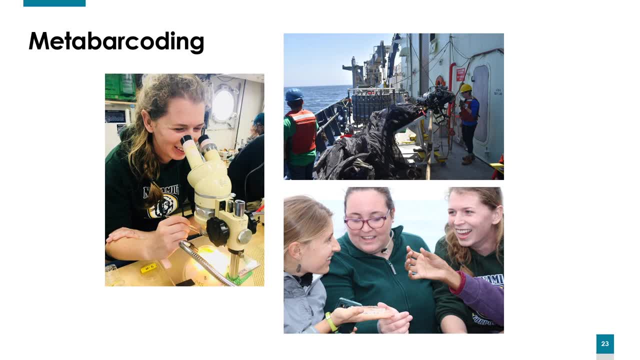 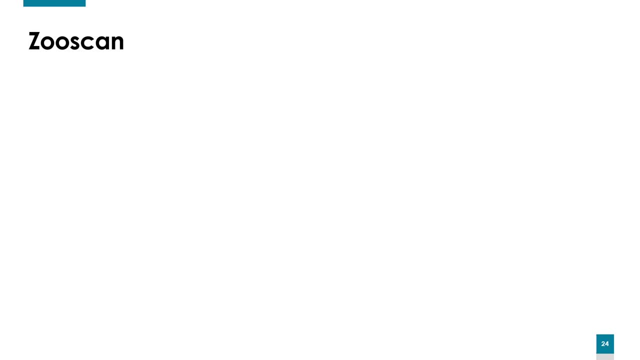 identify the different, the abundance and diversity of zooplankton in the ocean. Okay, so now we're at the part where I talk about what I do, And so I use ZoScan to scan and catalog organisms that were collected at sea using different types of nets. 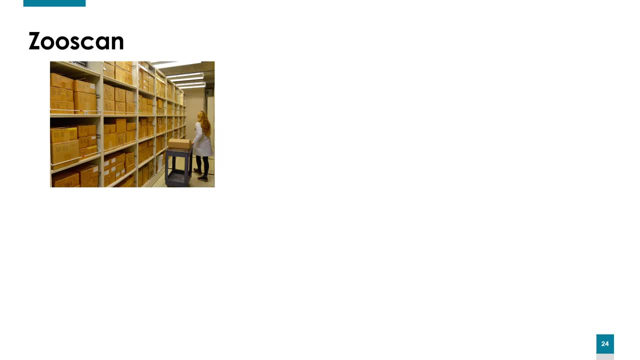 And so in order to actually get the samples, I have to go visit Lindsey down at she's the Pelagic Invertebrate Collections Manager at Scripps- And I gather my samples from her and take them back to the lab And basically what I do with each sample. 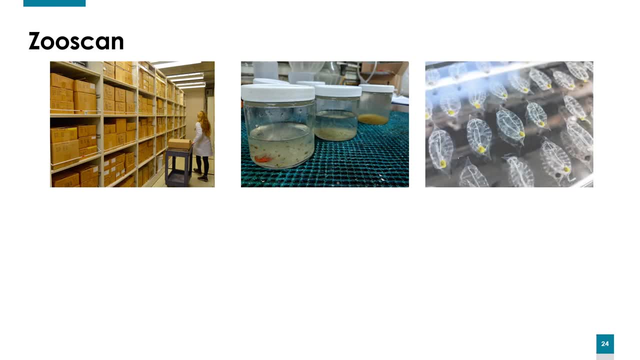 is, I split the sample based off of size And then from there I take an aliquot of the different size fractions and put the aliquot on the scan and disperse it so that none of the organisms are touching each other. And that's important because 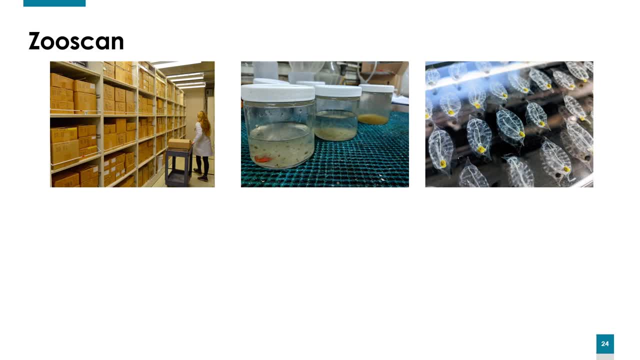 if organisms are touching each other and you go to scan it, it'll make it very hard for me to separate and manually sort the images later, And so, as you can see here at the bottom, these images are very detail rich, And if you were to zoom in on a raw image, 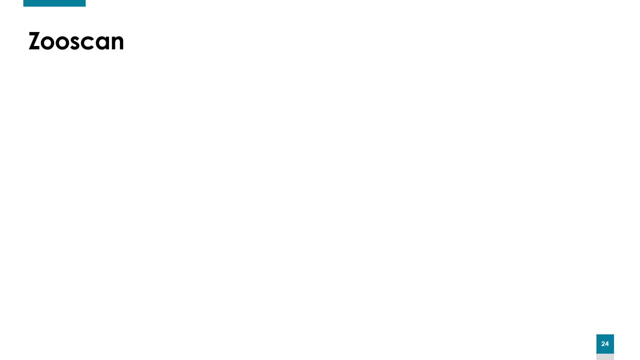 And so I use the zooscan to scan and catalog organisms that were collected at sea using different types of nets, And so, in order to actually get the samples, I have to go visit Lindsey, down at she's the pelagic and vertebrate collections manager. 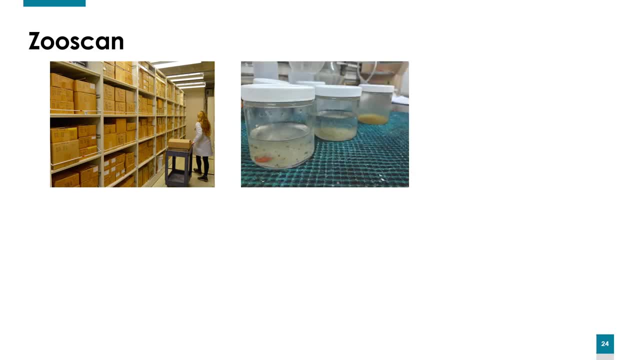 at Scripps And I gather my samples from her and take them back to the lab And basically I what I do with each sample is I split the sample based off of size And then from there I take an aliquot of the different size fractions. 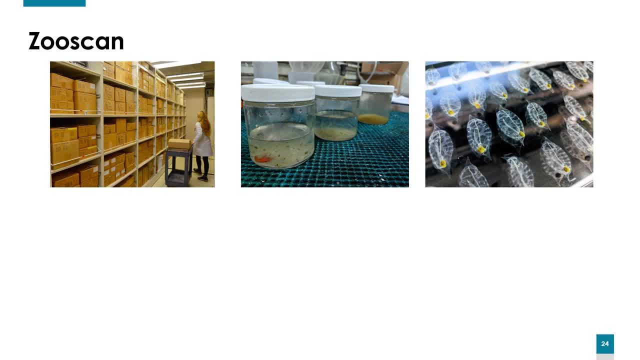 and put the aliquot on the scan and disperse it so that none of the organisms are touching each other. And that's important, because if organisms are touching each other and you go to scan it, it'll make it very hard for me to separate. 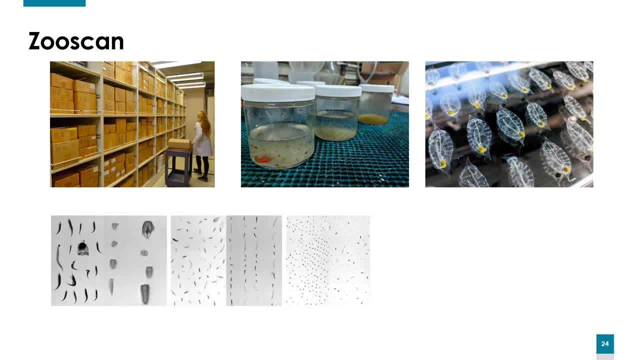 and manually sort the images later, And so, as you can see here at the bottom, these images are very detail rich And if you were to zoom in on a raw image, you could really see a lot of characteristics in the different zooplankton. 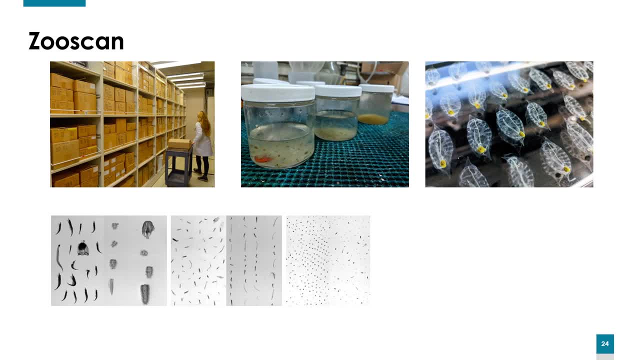 And making sure that they're not touching. it helps me better see the different characteristics and identifying them, And the images that are produced using the ZoScan are quite beautiful actually, and again full of detail, And they kind of give us a better image. 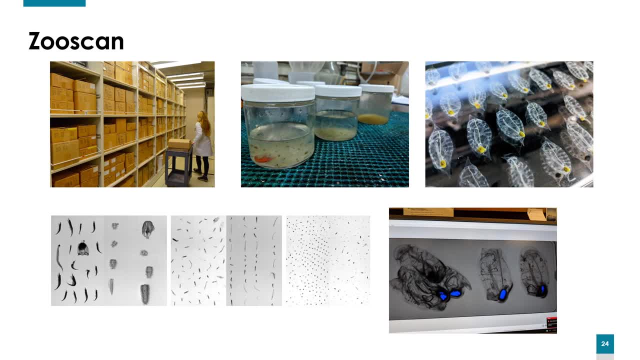 or a better idea of what some of these smaller zooplankton look like, And sometimes what we might do is we compare ZoScan images with images captured from the ZoScan or Zocam as well, And so what I want to show you quickly is a video. 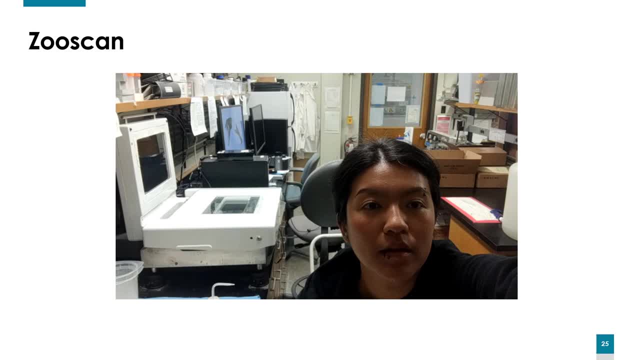 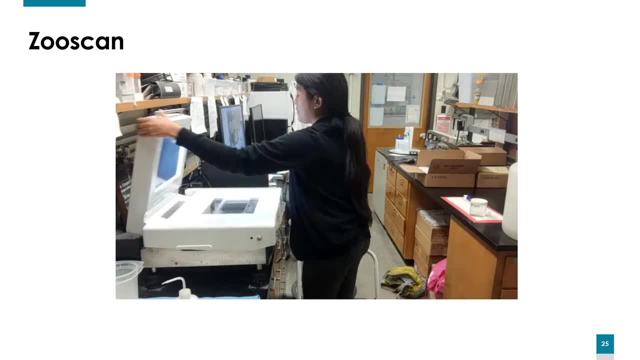 like a very simple time lapse of what I do in the lab. So here's my glamorous face, Just kidding. So what we see here is just me walking around using the ZoScan, And so I have to use a step stool to get up there. 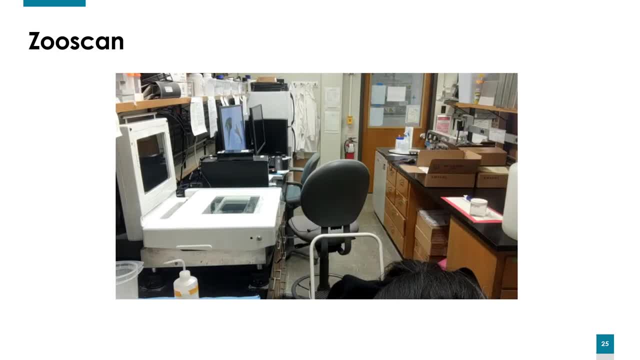 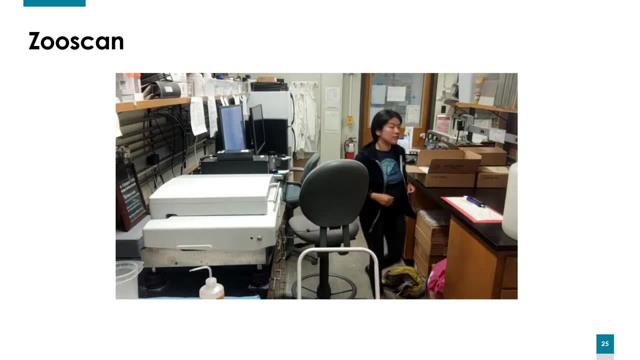 because I am on the shorter side, And though this may not be glamorous work, it is definitely necessary work, And so, by scanning images from these different samples collected out at sea, we're able to get a snapshot of the abundance and diversity of different types. 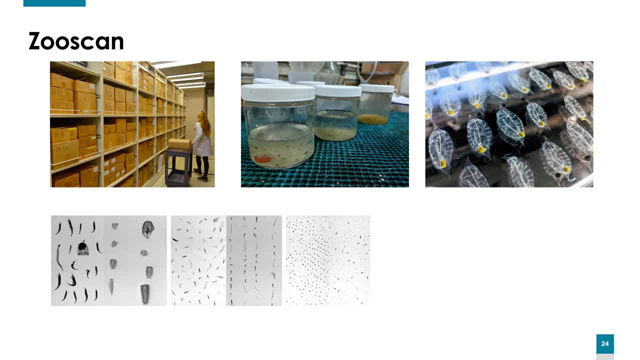 you could really see a lot of characteristics in the different zooplankton, And making sure that they're not touching it helps me better see the different characteristics and identifying them, And the images that are produced using the zooscan are quite beautiful actually. 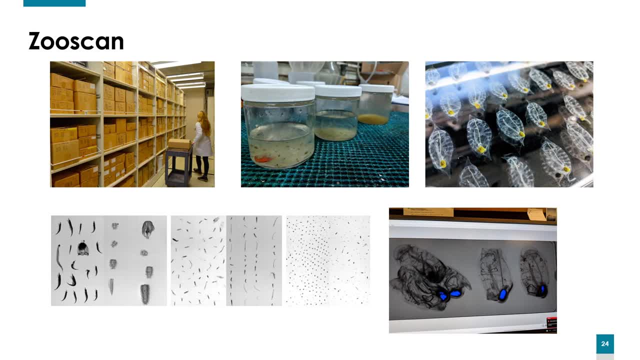 And again full of detail, And they kind of give us a better idea of what some of these smaller zooplankton look like. And sometimes what we might do is we compare zooscan images with images captured from the zooscan. 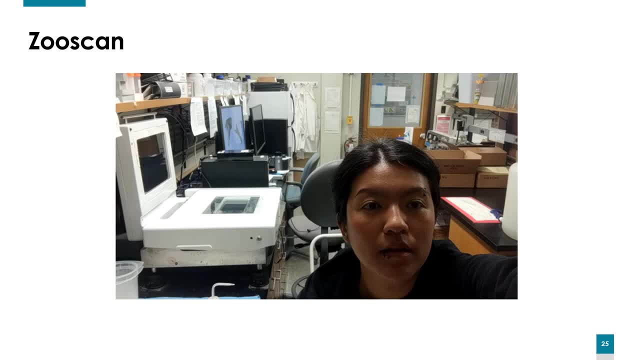 or zocam as well, And so what I want to show you quickly is a video, like a very simple time lapse of what I do in the lab. So here's my glamorous face, Just kidding. So what we see here is just me walking around right. 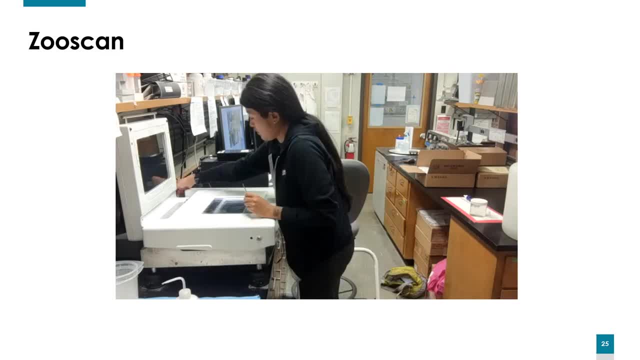 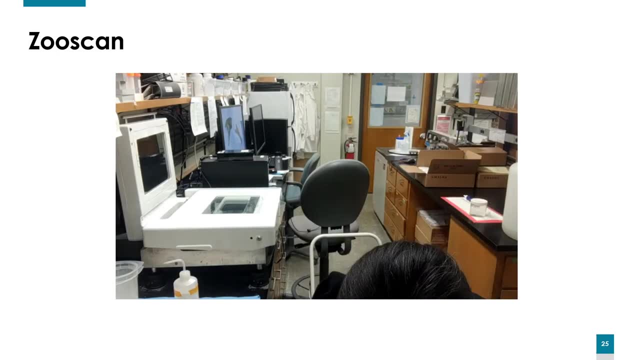 using the zooscan, And so I have to use a step stool to get up there because I am on the shorter side. And though this may not be glamorous work, it is definitely necessary work, And so, by scanning images from these different samples, 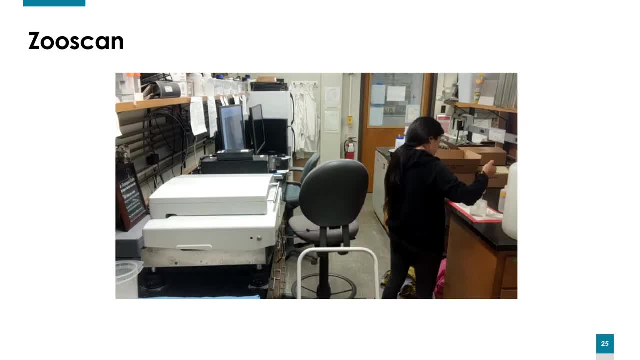 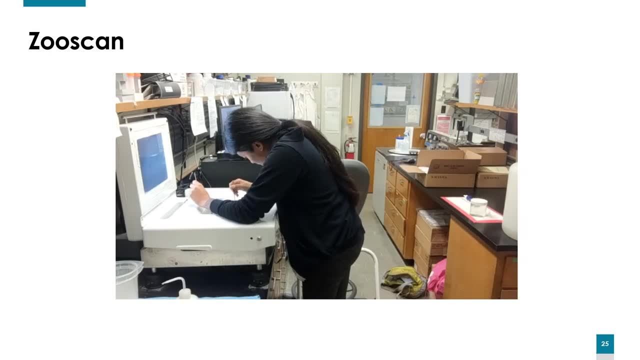 collected out at sea. we're able to get a snapshot of the abundance and diversity of different types of zooplankton that are collected from different parts along the Santa Barbara basin and other parts of the ocean, So it's good work overall. Hey, we are near the finish line. 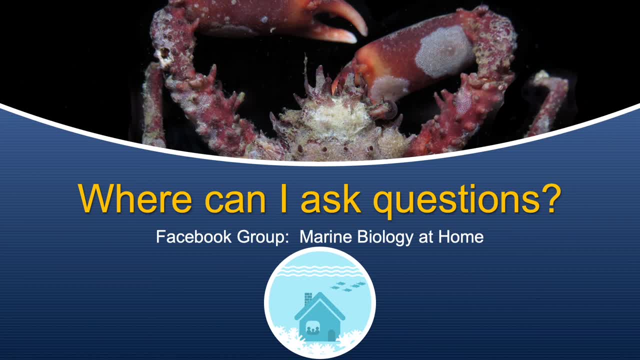 I'm sure you guys are ready to exit out of your web browser, And so, before we wrap it up today, though, I just want to encourage everyone to please help spread the word about marine biology at home, And if you know someone that would like to contribute. 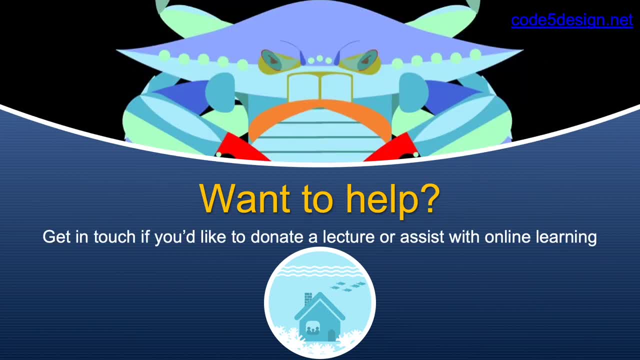 or you know someone that maybe would like to expand more on a specific topic that they have seen in our videos here. please go ahead and send them over to our Facebook group, Marine Bio at Home to get more info and to figure out how to contribute, like that. 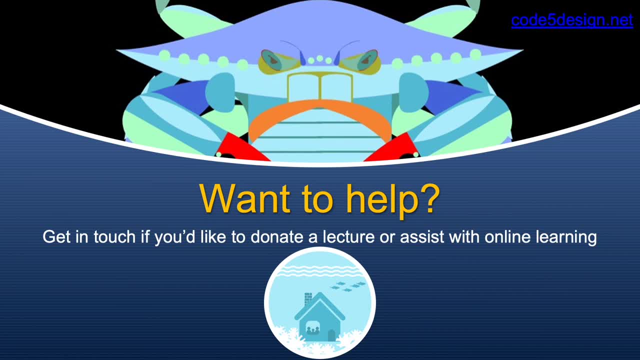 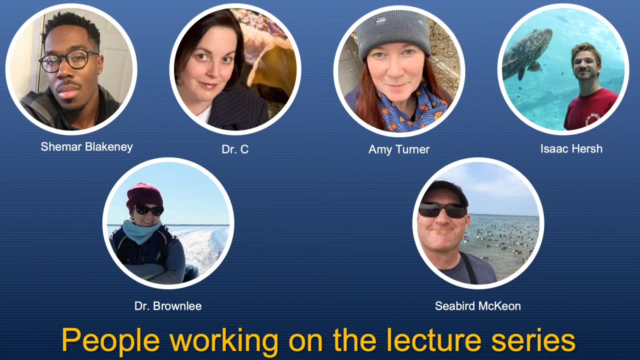 And so thank you everyone for your support for continuing to stay interested, for asking questions and being present. Sometimes it can't be easy because, given the current situation, a lot of us are stuck at home, So let's try our best to try to stay engaged with one another. 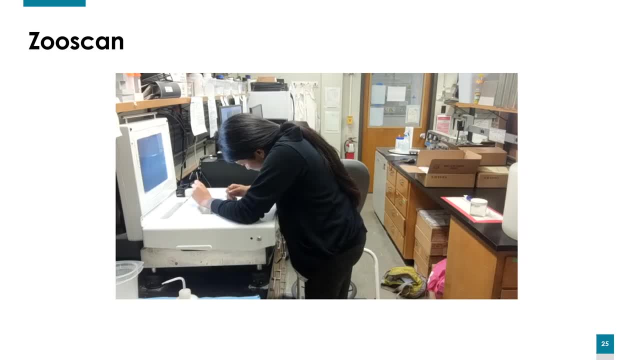 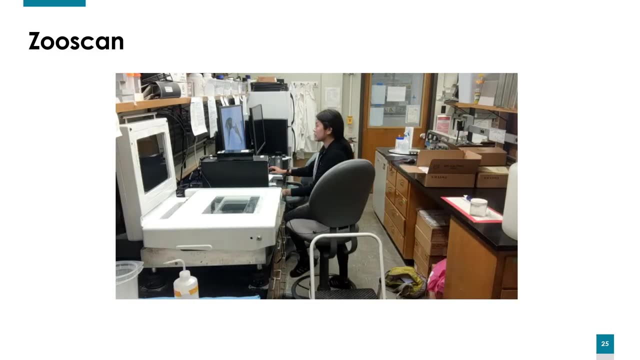 of zooplankton that are collected from different parts along the Santa Barbara Bay, So we can see the different types of zooplankton that are collected from different parts of the ocean. So it's good work overall. Hey, we are near the finish line. 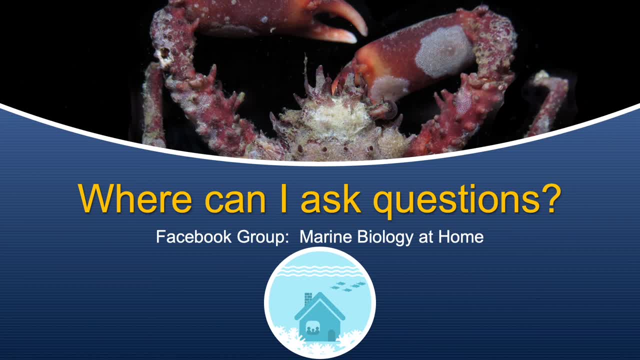 I'm sure you guys are ready to exit out of your web browser, And so, before we wrap it up today, though, I just want to encourage everyone to please help spread the word about marine biology at home, And if you know someone that would like to contribute. 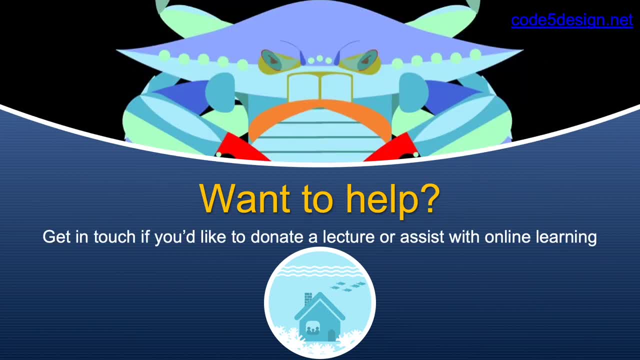 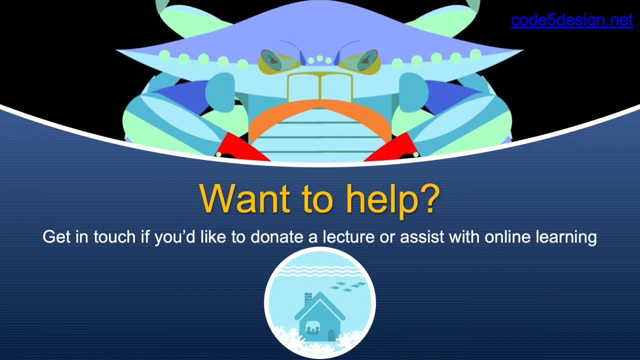 on a specific topic that they have seen in our videos here. please go ahead and send them over to our Facebook group, Marine Bio at Home to get more info and to figure out how to contribute like that, And so thank you everyone for your support. 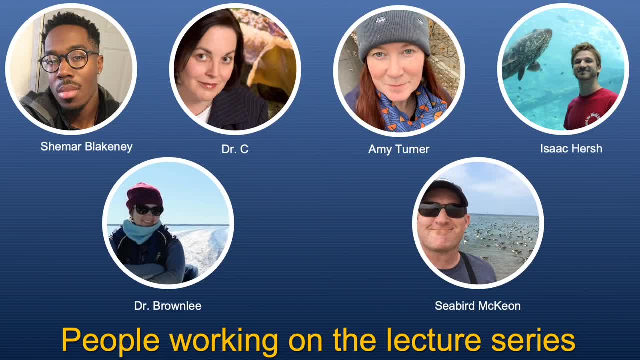 for continuing to stay interested, for asking questions and being present. Sometimes it can't be easy Because, given the current situation, a lot of us are stuck at home. So let's try our best to try to stay engaged with one another, to check in with one another and to continue awesome research. 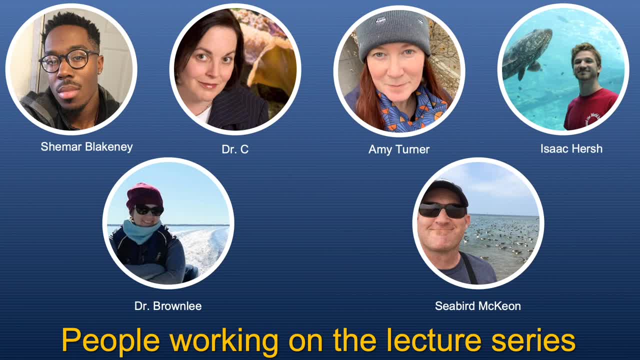 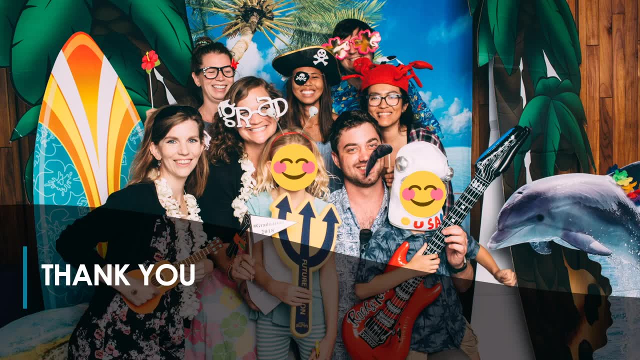 in the sciences and to report back and tell other people about what we've learned. And again, thank you to everyone for watching this video today. I hope that it was informative enough to give you a little bit of a sense of what's going on. 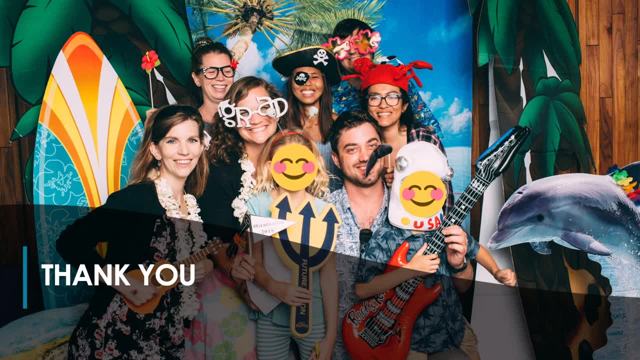 And I hope that you have a great day. And I hope that you have a great day, Generate some interest for yourself and learn more about zooplankton and the oceans in general. Thank you to everyone that contributed information for this lecture. 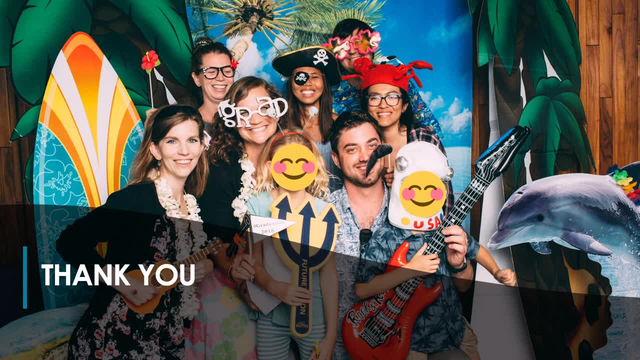 And I hope that everyone has a great and fantastic day. See you later.